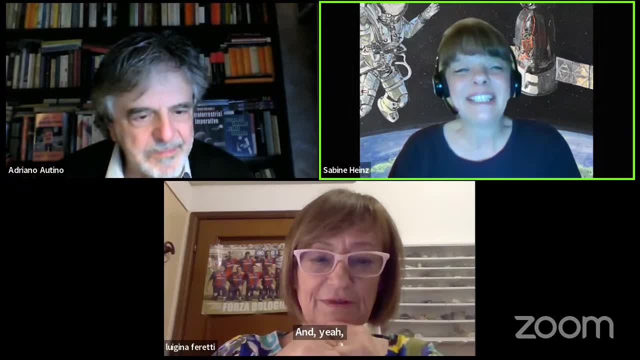 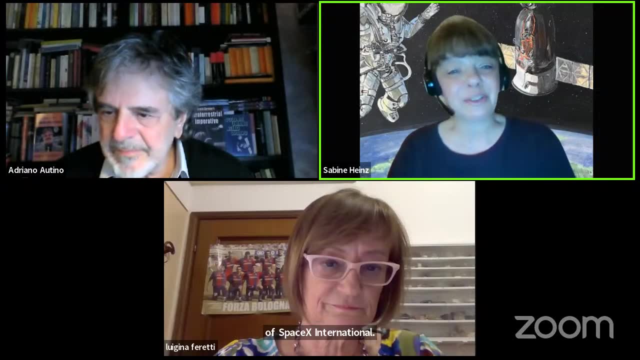 And yeah, I welcome you to our webinar by the Academy of Space Renaissance International And on this 8th of April, I'm really delighted that you have come to join us. My name is Sabine Heinz and I'm the person responsible for our webinar series. 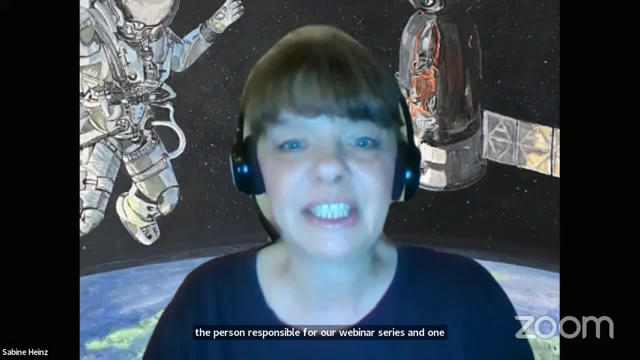 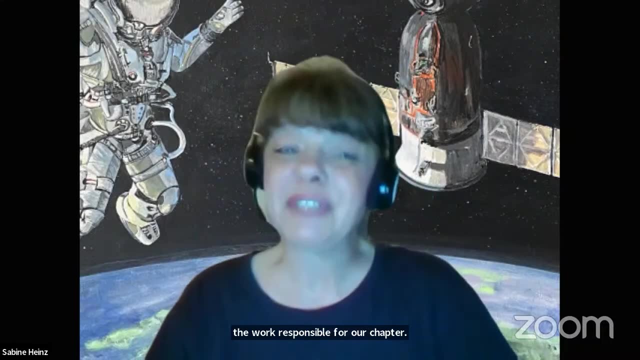 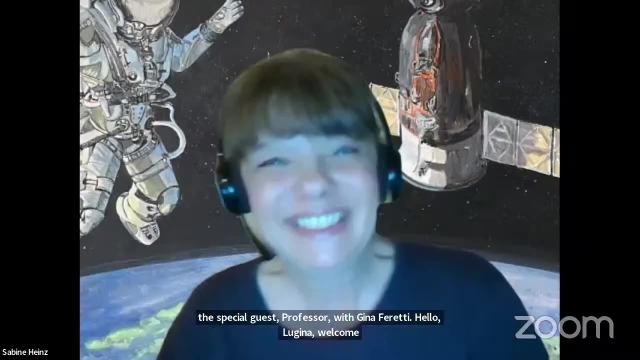 and one of the vice presidents of Space Renaissance International and also responsible for our art chapter. Our today's special guest is Professor Luigina Ferretti. Hello, Luigina, welcome. Hello. thank you, We are really glad that you are here. 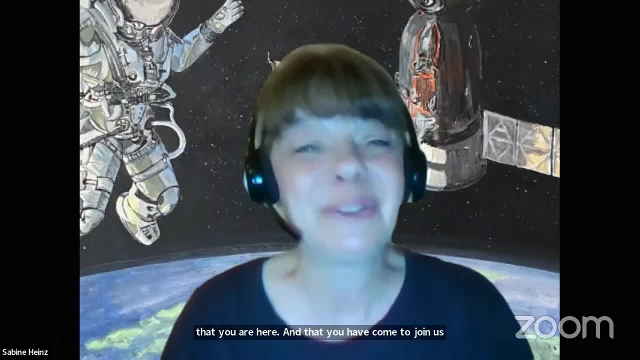 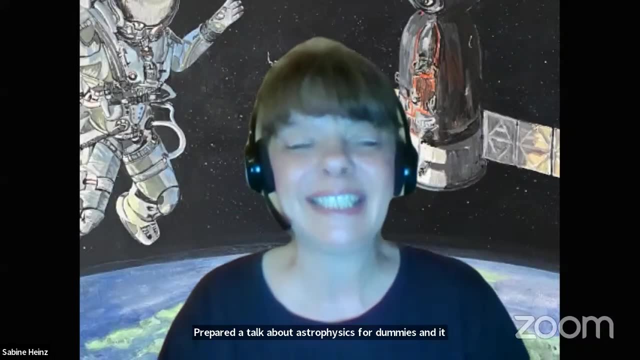 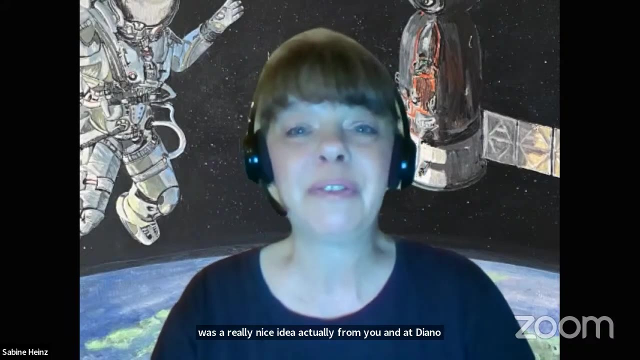 that you have come to join us and that you have prepared a talk about astrophysics for dummies, And it was a really nice idea actually from you and Adriano to initiate this, because in our audience we also have many artists and space-interested people. 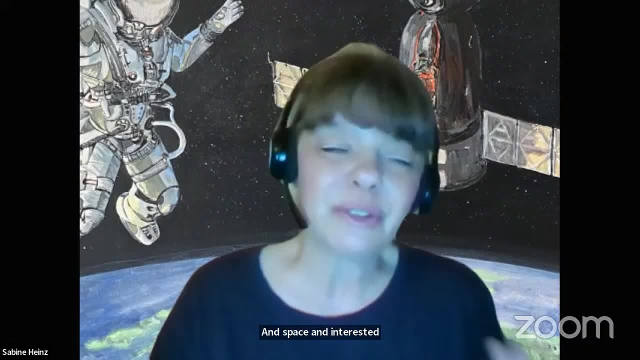 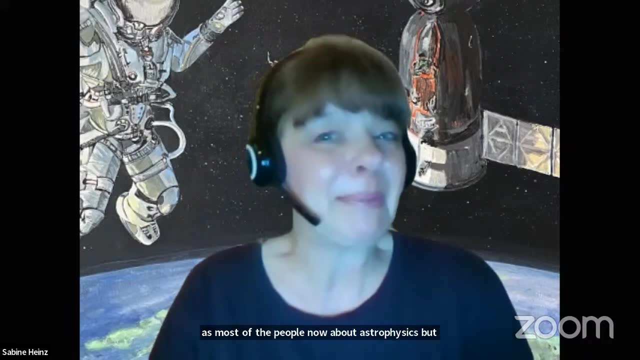 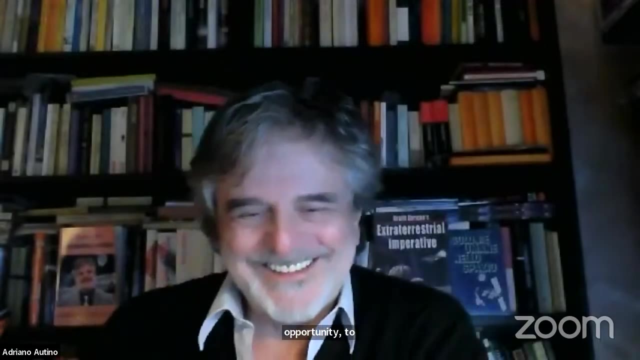 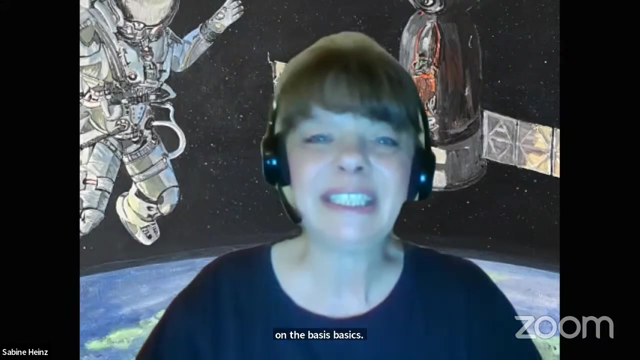 engineers and yeah, but most of the people know about astrophysics, But There are some who are really happy that you give us the opportunity to have a fundamental look on the basics. I also would like to welcome Adriano Ortino. He is also one of our vice presidents and former presidents of Space Renaissance International. 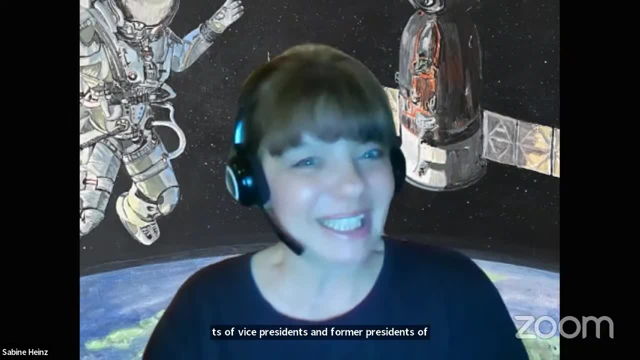 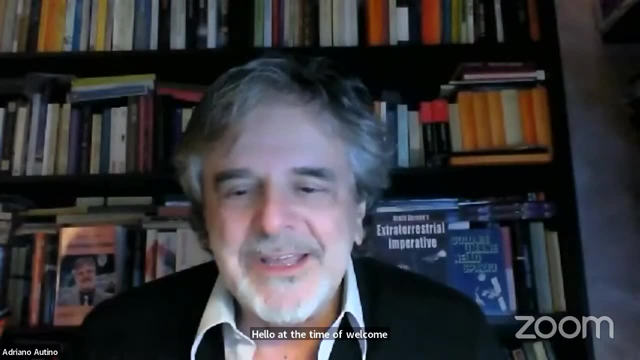 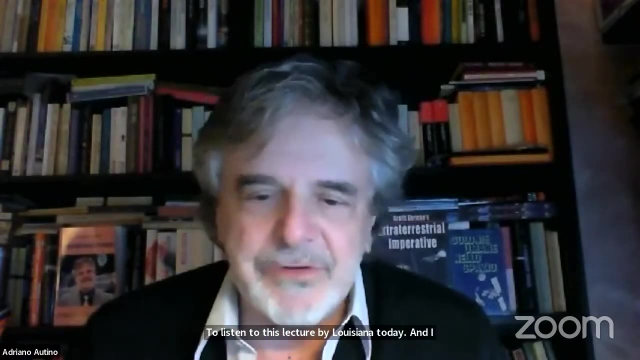 and one of the founders. Hello Adriano, welcome. Hello Sabine. Hello Luigina, Welcome to you both. And yeah, I'm very happy to listen to this lecture by Luigina today And I will try to learn something, because I have to confess I'm very, very ignorant about astronomy and astrophysics. 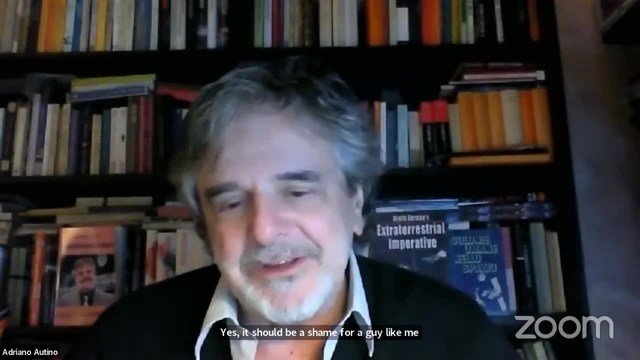 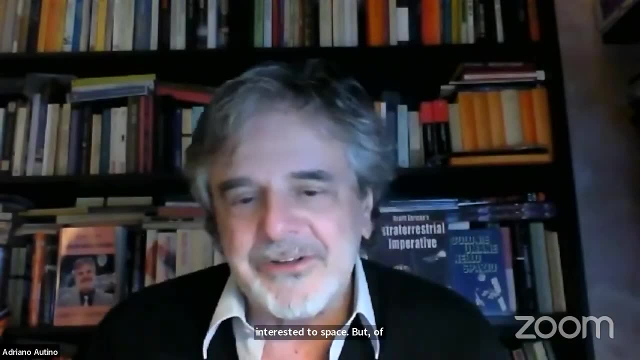 Yes, it should be a shame for a guy like me that I'm interested to space. But of course one thing is to be interested and to be interested And another thing is to be a scientist And to know everything what is to be known. 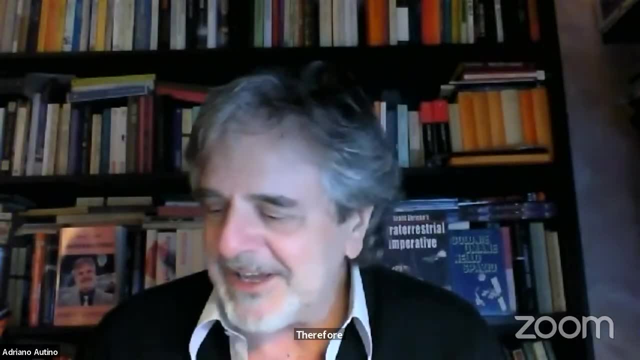 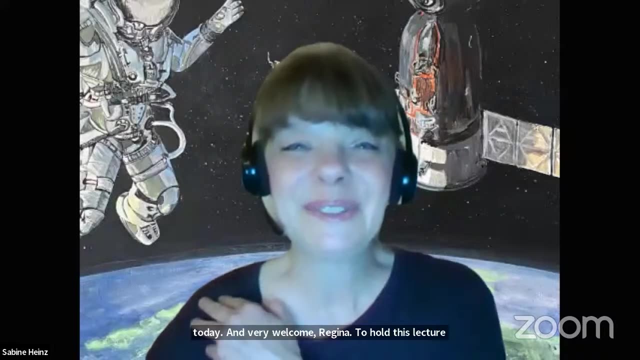 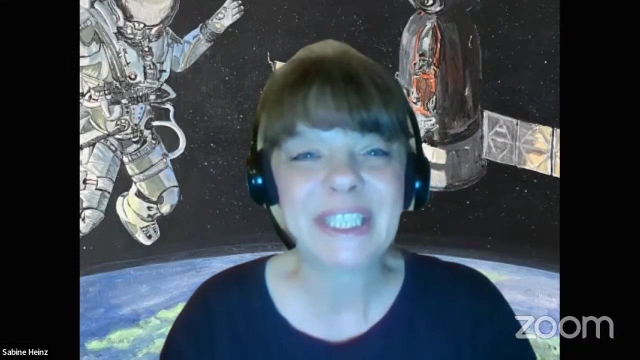 Therefore, I'm very happy to try to learn something today And very welcome Luigina to hold this lecture. Yes, thank you, Adriano And Luigina. before I give you the floor, I would like to introduce you to our audience. 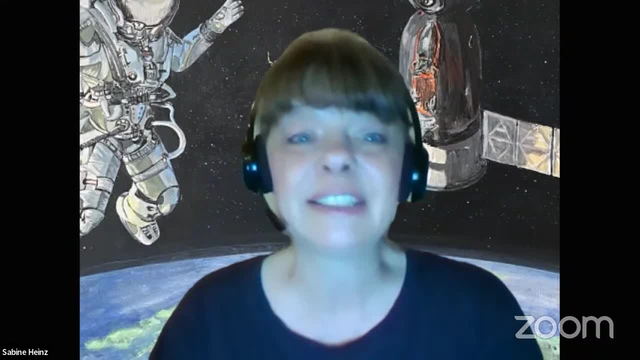 Professor Luigina Ferretti graduated in physics at the University of Bologna and carried out research in the field of astrophysics. Professor Luigina Ferretti graduated in physics at the University of Bologna and carried out research in the field of astrophysics. 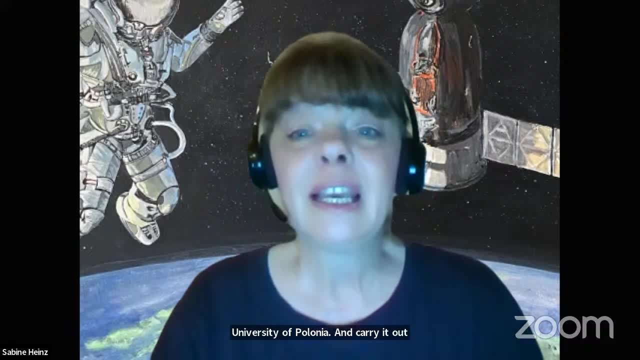 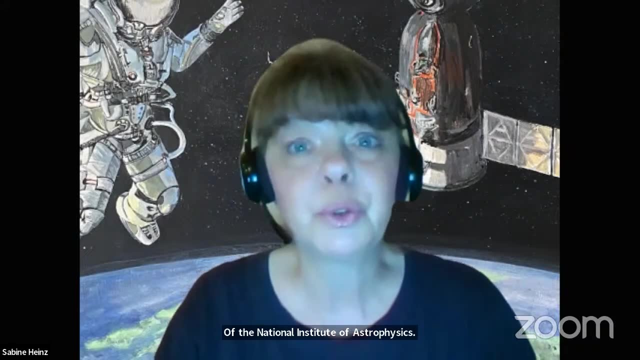 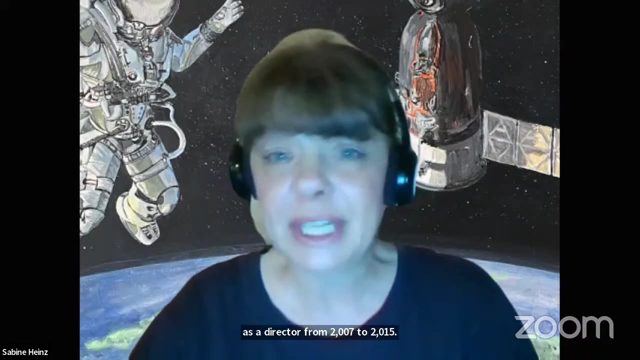 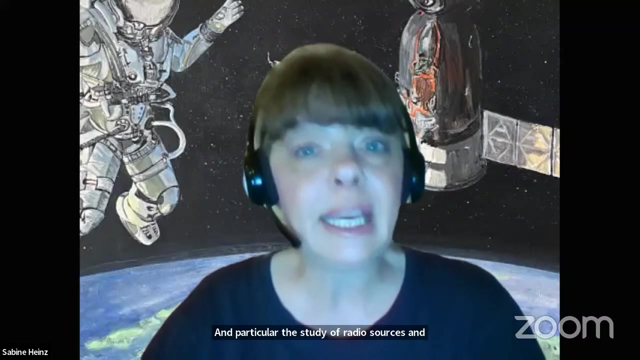 She held a research activity at Instituto de Radioastronomia of the National Institute of Astrophysics, where she acted as a director from 2007 to 2015.. The field of research is extra-galactic radio astronomy, in particular, the study of radio sources and clusters of galaxies, and the study of large-scale cosmological magnetic fields. 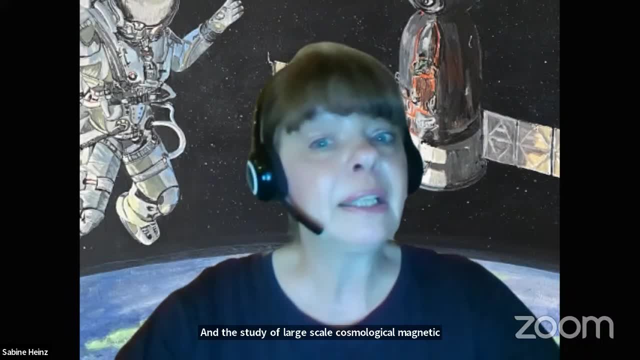 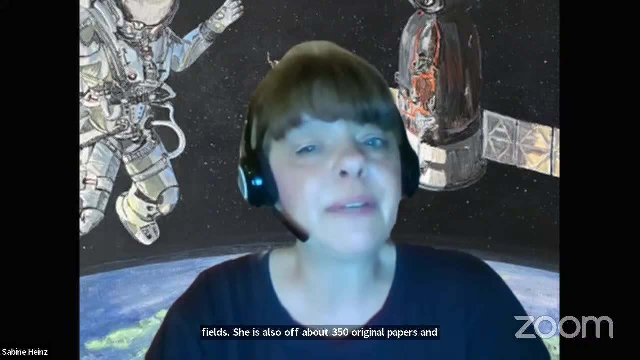 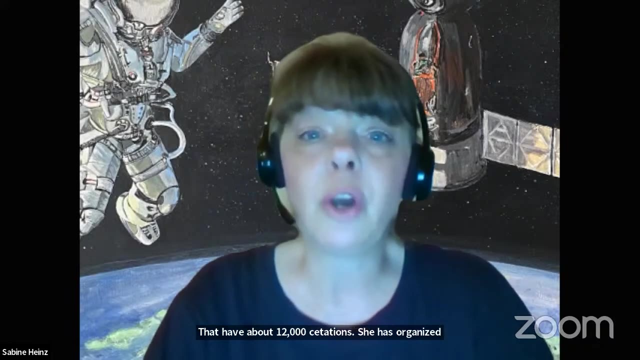 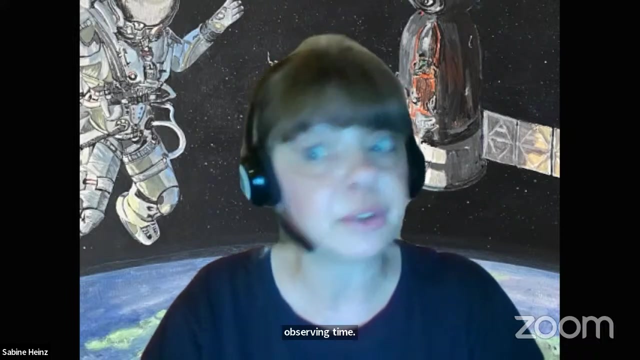 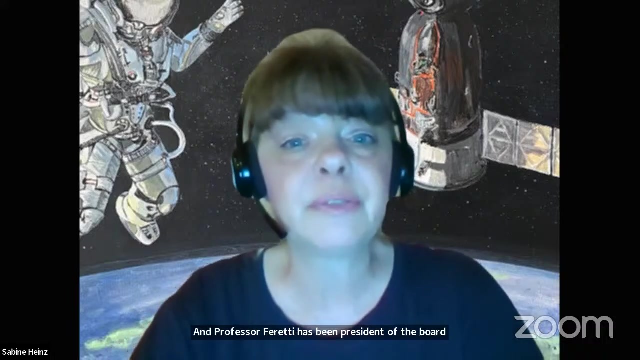 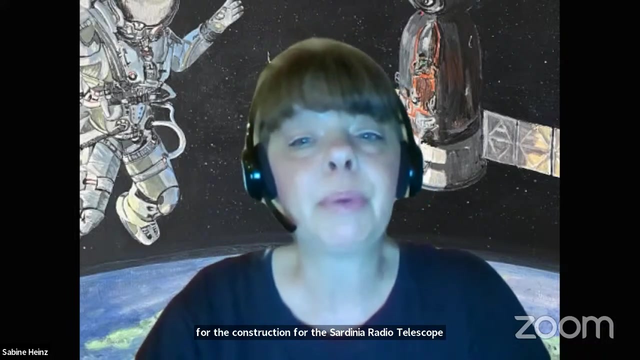 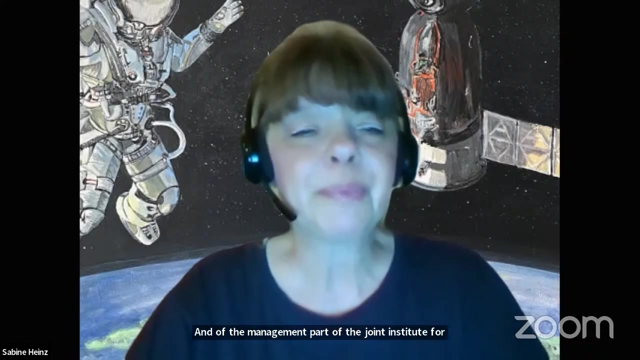 She is author of about 350 original papers in international scientific journals that have about 12,000 citations. She has organized several international conferences and participates in committees for research funding and allocation of observing time at international instruments. And Professor Ferretti has been president of the board for the construction for the Sardinia radio telescope near Cagliari and of the management board of the joint institute for YLBE in Europe- LBI in Europe. 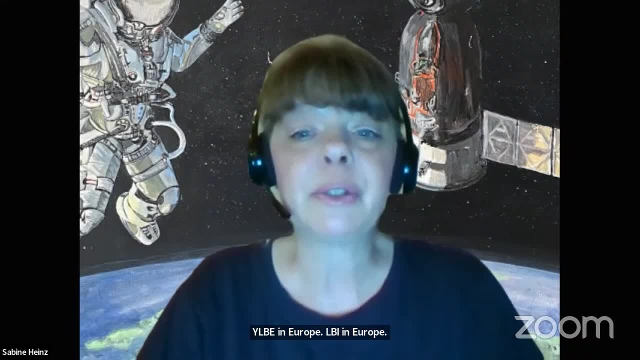 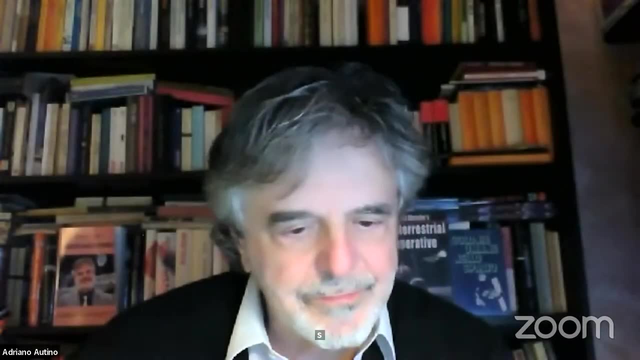 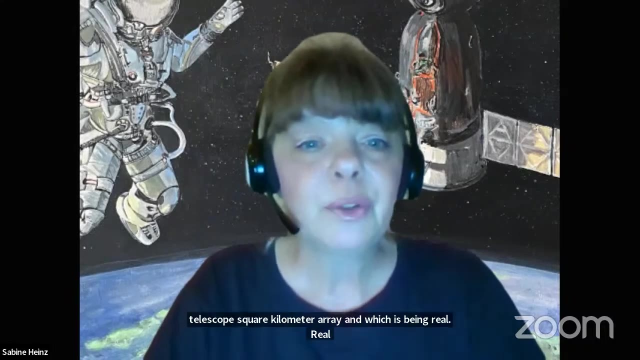 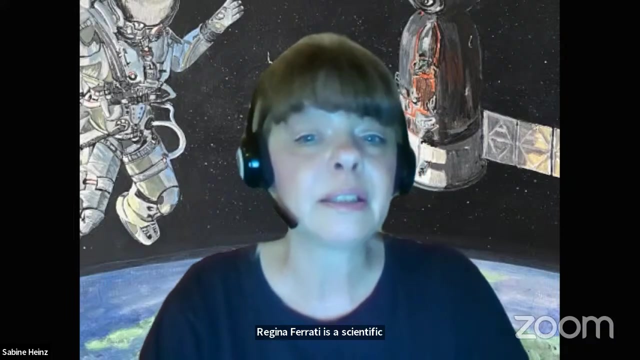 She's involved in science working groups of the new generation radio telescopes- square radio telescopes, Sardinia radio telescopes, square kilometer array- which is being realized in South Africa and Australia. Lugina Ferretti is a scientific editor of the international journal the Astronomy and Astrophysics Review and is a member of the International Astronomical Union. 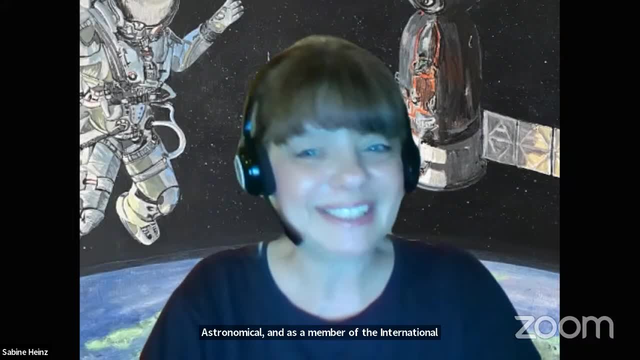 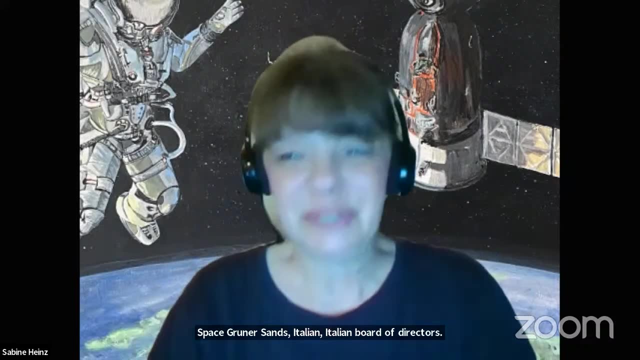 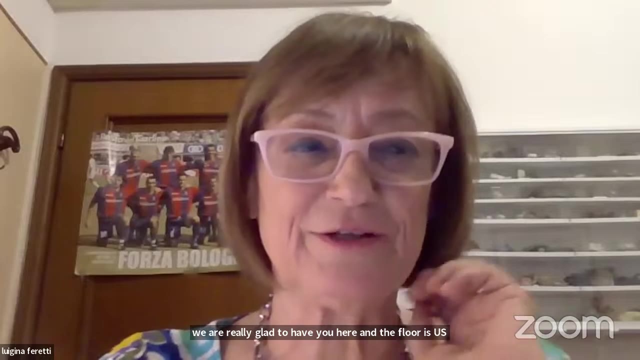 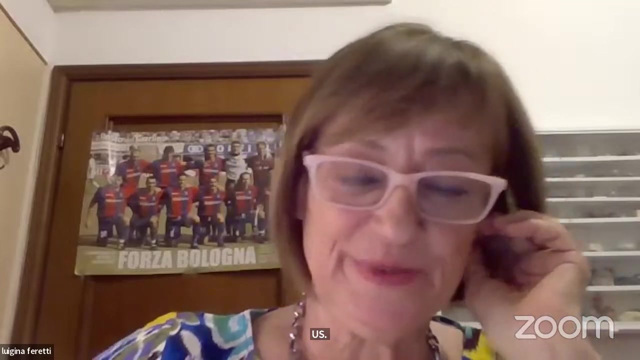 And she is also a member of the Space Renaissance Italia Board of Directors. Lugina, we are really glad to have you here and the floor is yours. Thank you very much for your nice introduction, Too good. I mean, it's really an honor to be here and I hope, to teach you something. 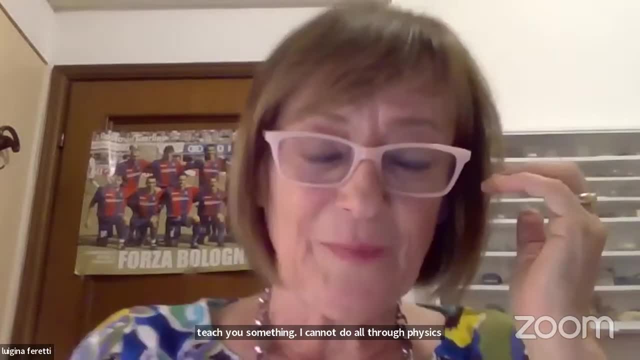 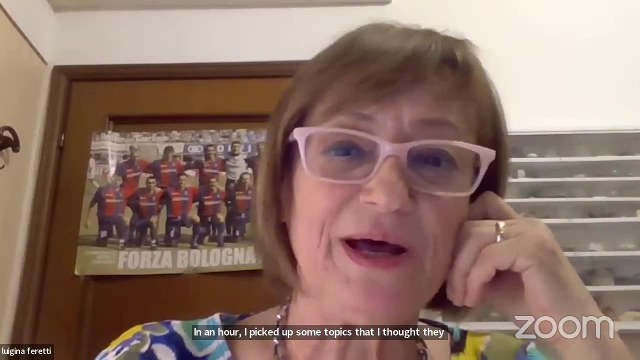 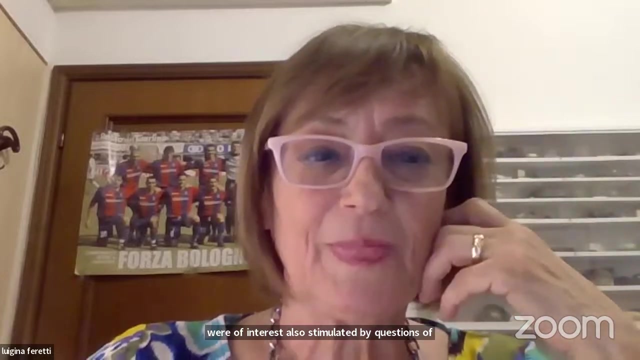 I cannot do all astrophysics in an hour. I picked up some topics that I thought They were of interest, also stimulated by questions of Adriano and talks with him, And so can I start. Yes, you may share. I have one more question, then. 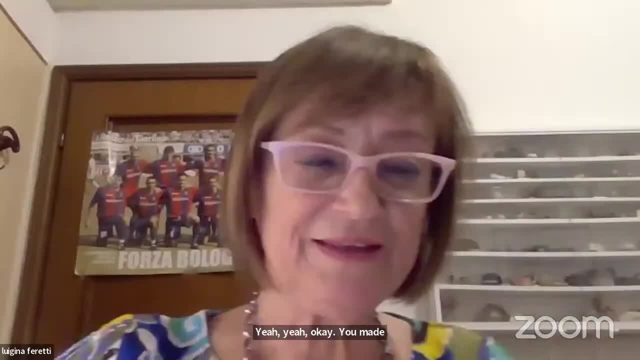 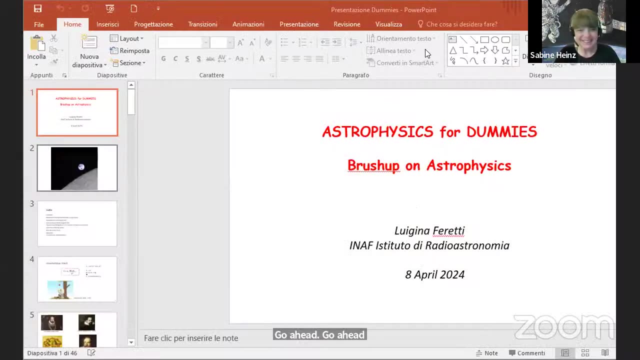 Ah, yeah, okay, You may share the screen first and then after that you can ask all your questions. So you may share through the screen. So It's shared and you can start your slides. So you see the screen. 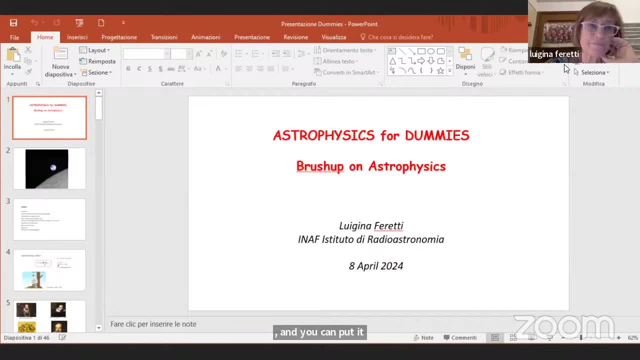 Yes, and you can put it on full screen. Yeah, yeah, this is what I'm trying to do, Adriano. can you explain her in Italiano, where it is One on the right, This icon? No, no, no. 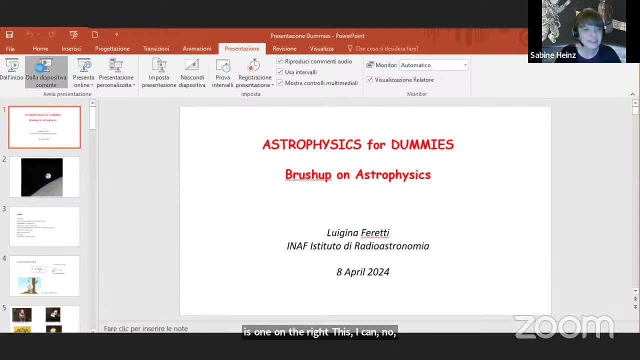 On the left-hand side, second icon, You can touch No, no, no more up. Yes, it's okay. Oh, yeah, it's okay. Yeah, perfect, We made the right answer today. Never mind, Is it okay? 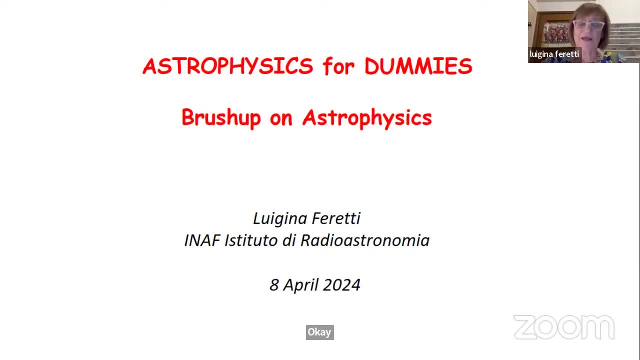 Yes, it's perfect, Great, Great. So the title was Astrophysics for Dummies. I think I put a subtitle which is a brush up on astrophysics for those who know already something, So it's kind of a refreshment. 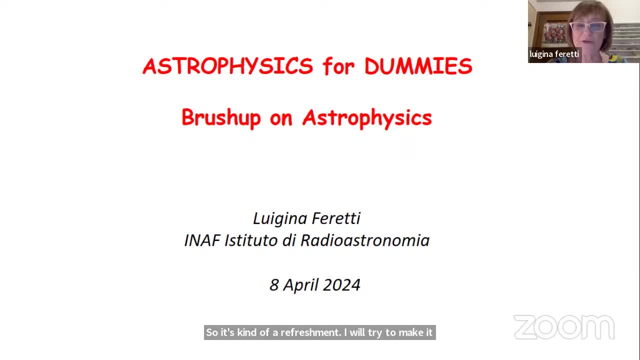 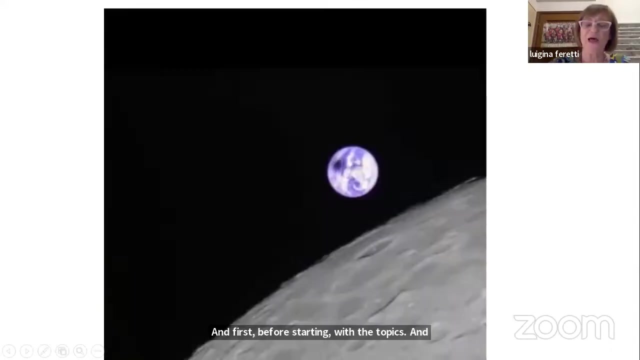 I will try to make it simple Without avoiding the formulas, So please stop me if you don't understand, if there is anything unclear. First, before starting with the topics, I wanted to honor this solar eclipse of today. Okay, And this is a picture that was taken. 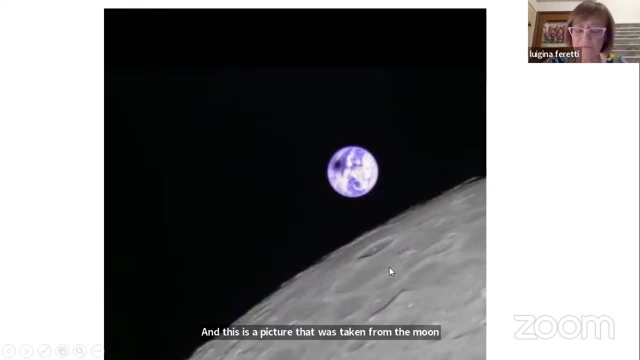 This is a picture that was taken from the moon already five or four years ago, And you see the surface of the moon And you see the earth, And you see the shadow cast from the moon on the earth, which is exactly what is happening right now. 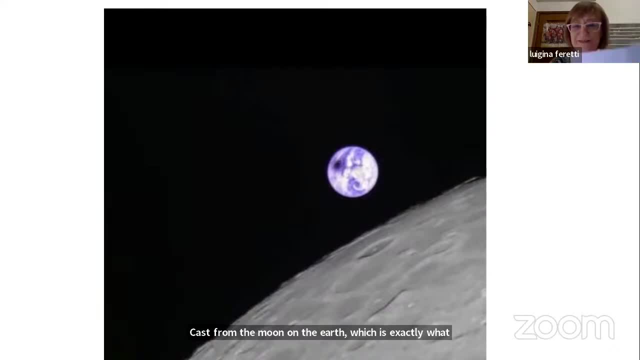 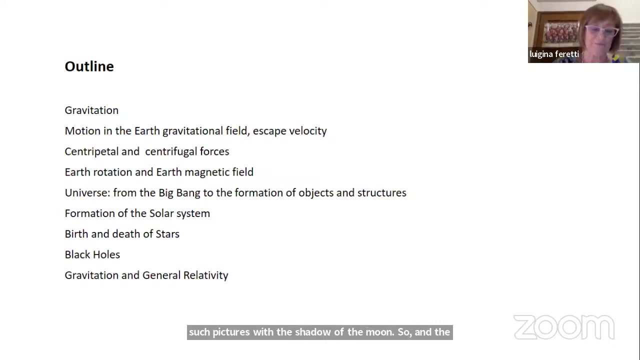 I think this picture is not of good quality, but in my opinion it's very impressive. There are not many Such pictures with the shadow of the moon, So the outline of my talk is talking of basics Issues in physics: gravitation, motion in the earth, gravitational field, escape velocity, centripetal and centrifugal forces, and then earth rotation and earth magnetic field. 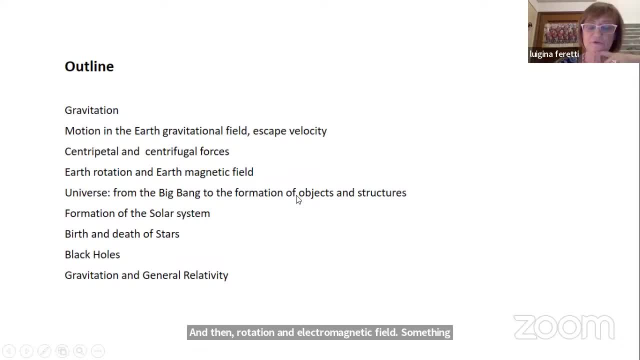 Something about the universe, from the Big Bang To the formation of object and structure, formation of the solar system and quickly on the evolution of stars. Then I put a few slides on black holes and gravitation as interpreted by Einstein. So gravitation and general relativity. 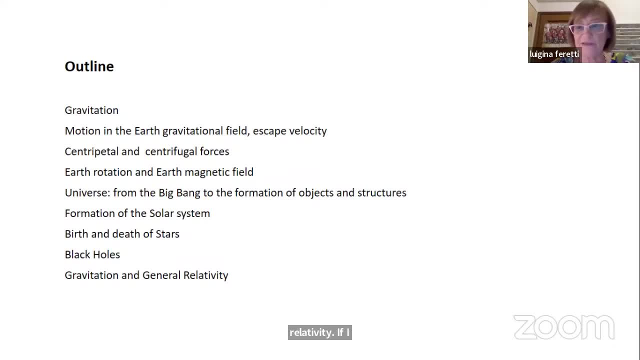 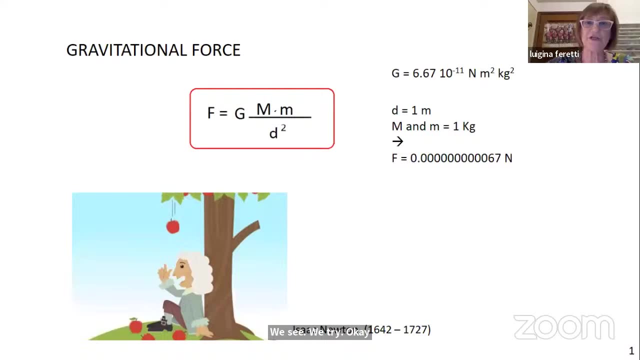 I'm not sure I will have time to do everything, But We'll see, We'll try. We'll try. Okay, So gravitation. Gravitation is the dominating force in the universe, So we have to start with this. 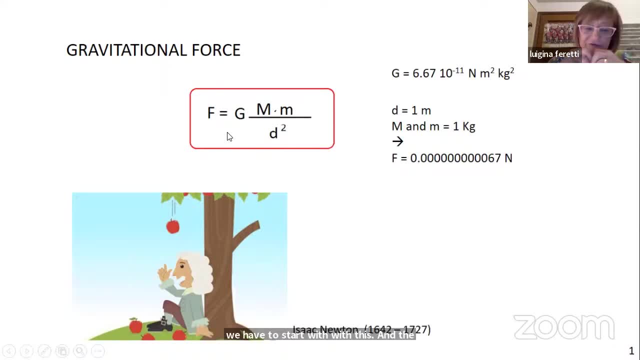 The force is. the law of gravitation is very simple and complete And it says that every object in the universe with a certain mass- m, A big M- attracts any other object of a different mass with the force that is proportional to both masses and it is inversely proportional to the square of the distance between them. 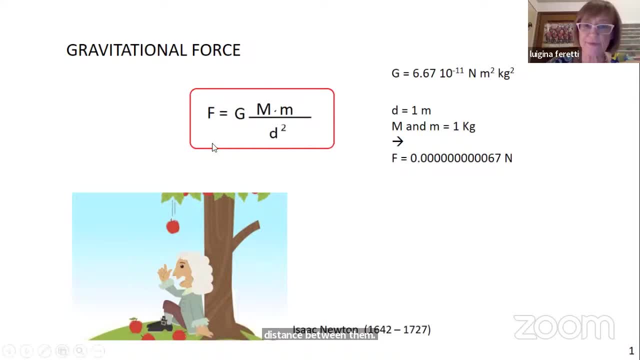 So this is the mathematical expression: F force equal m times small m divided by the distance squared. There is a constant, There is a constant. There is a constant. There is a proportionality constant, which is a G, which is the gravitational constant- and it is a very small number- is a zero, comma, zero, zero, zero. you need the 10 zeros before arriving to the first digit. 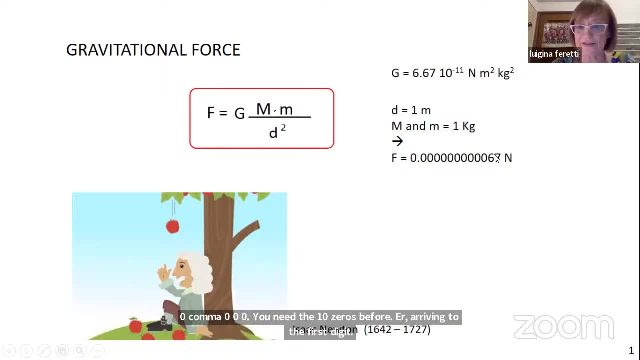 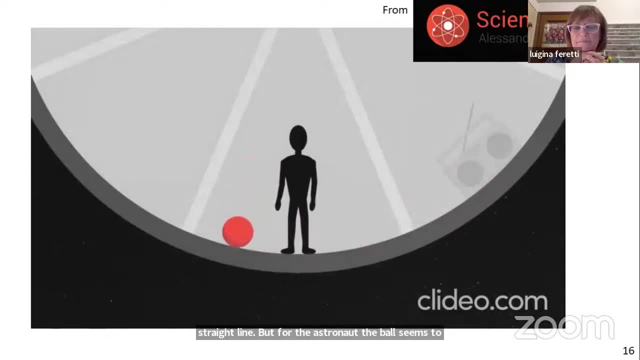 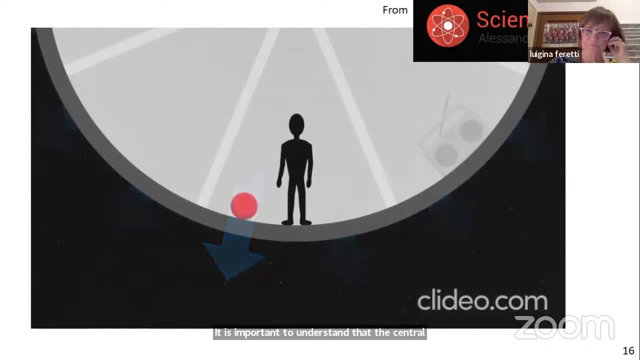 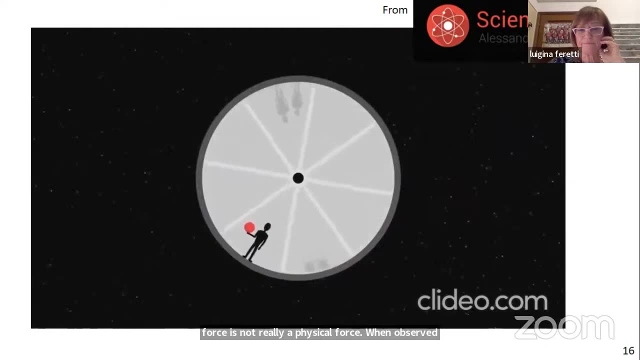 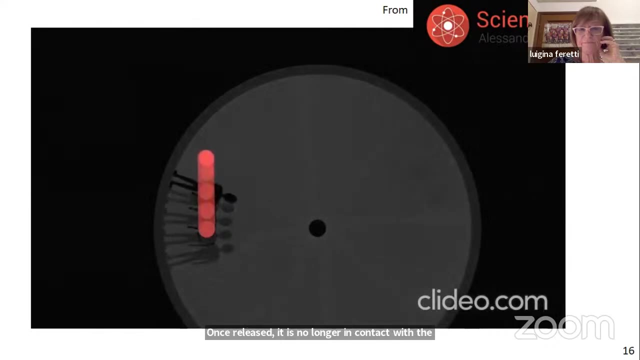 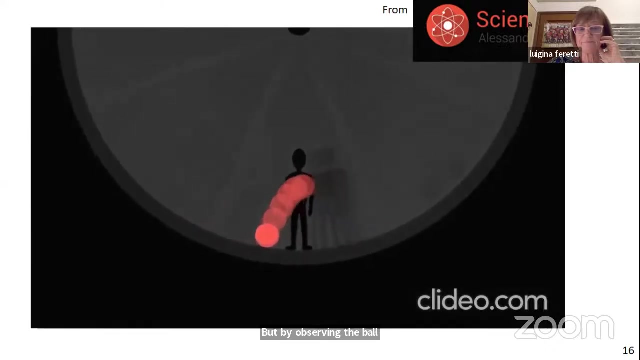 It is important to understand that the centrifugal force is not really a physical force. When observed from the outside, we understand that the ball has not undergone anything. Once released, it is no longer in contact with the astronaut and it therefore moves straight ahead. But by observing the ball while spinning, the astronaut has the impression that there is an 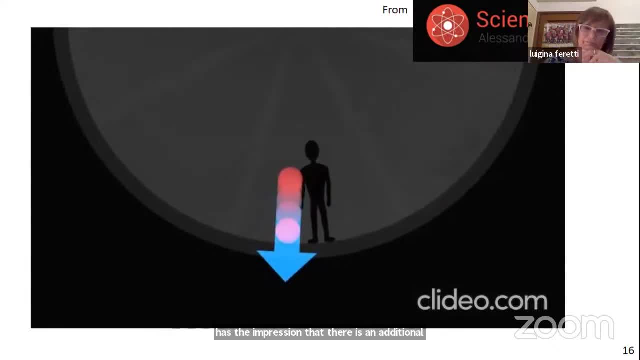 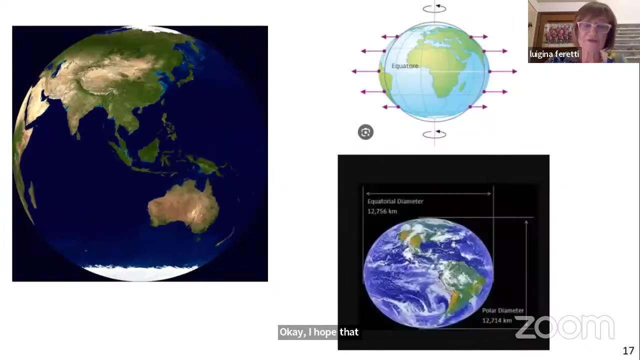 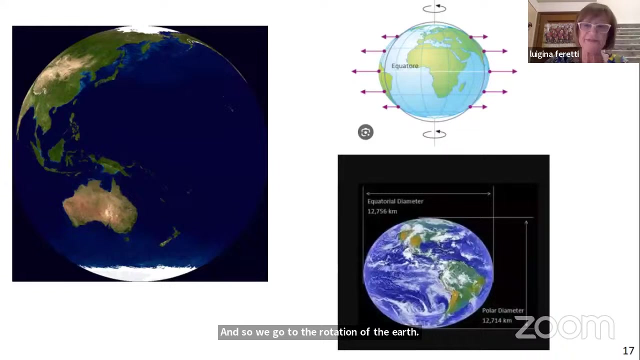 additional fictitious force, the centrifugal force, which he invents to explain the motion of the ball in his frame of reference. Okay, I hope that this is clear, And so we go to the rotation of the Earth. Rotation of the Earth is rotating. 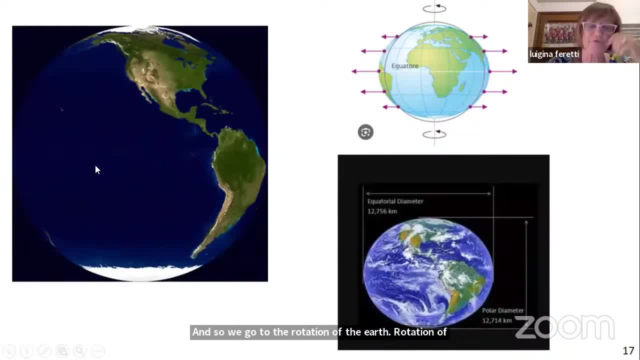 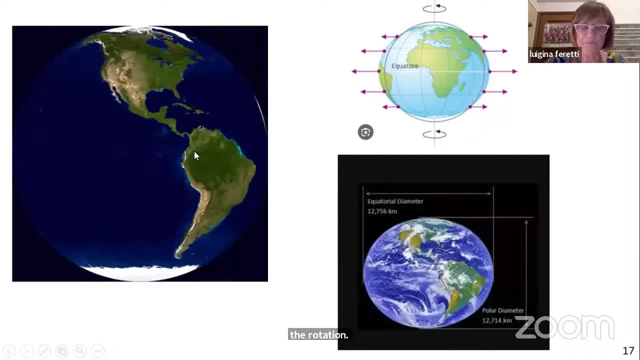 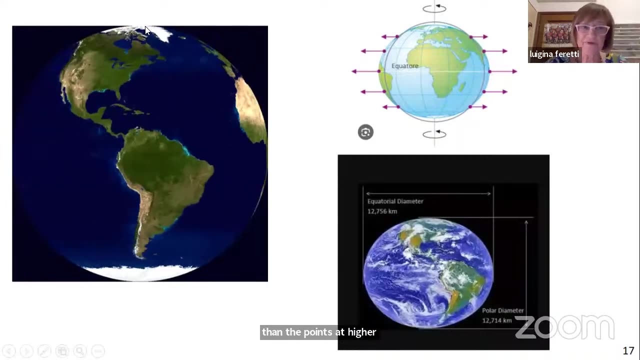 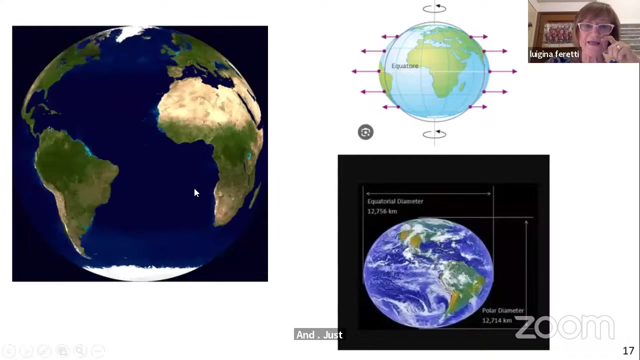 And due to what we said before, the rotation, the points at the equator are moving at higher speed than the points at higher latitudes and the pole is not moving, it's just a point, or moving very, very slowly. So you see the forces here. This is the force toward the 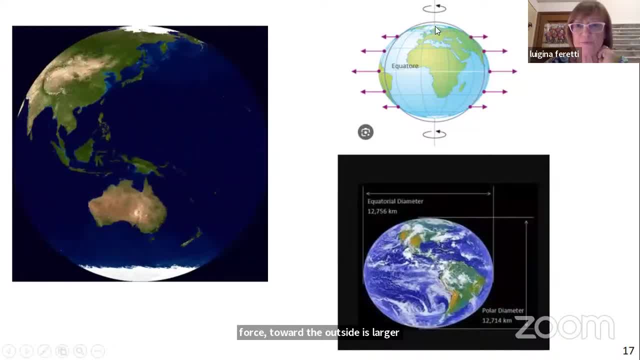 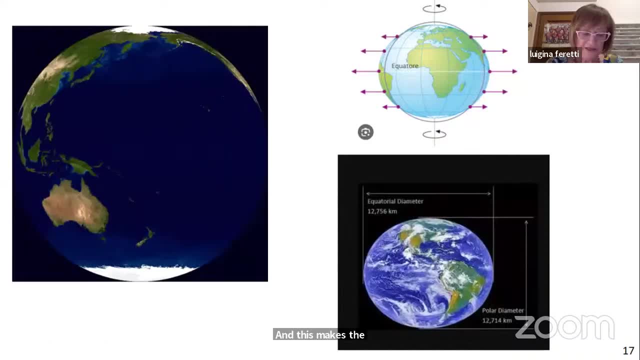 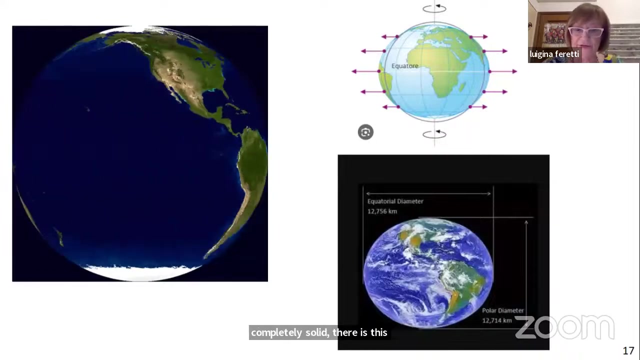 outside is larger at the equator and smaller, smaller going to the north, And this makes the Earth squashed into a slightly flattened sphere. So the effect actually is quite small. but since the Earth is not completely solid, there is this flattening of the Earth, And you see here the amount of the flattening. It is not big. 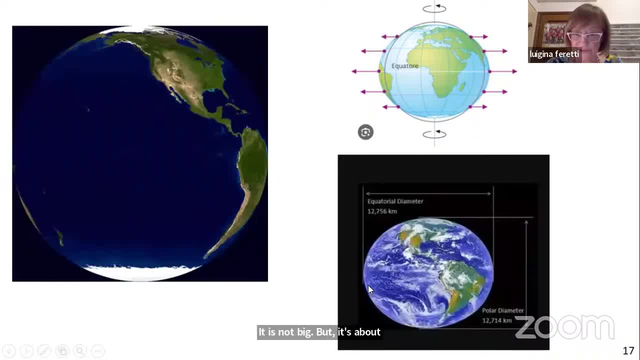 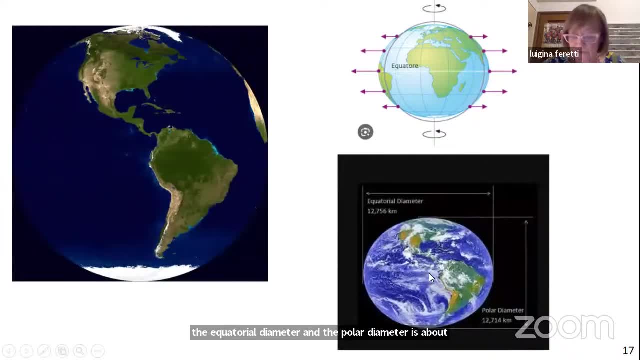 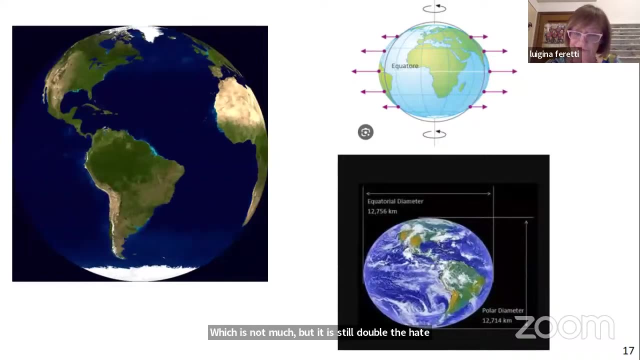 But it's about. the difference between the equatorial diameter and the polar diameter is about 42 kilometers, which is not much, but it is still double the height difference between the top of Mount Everest and the deepest point of the ocean, the Mariana Trench. 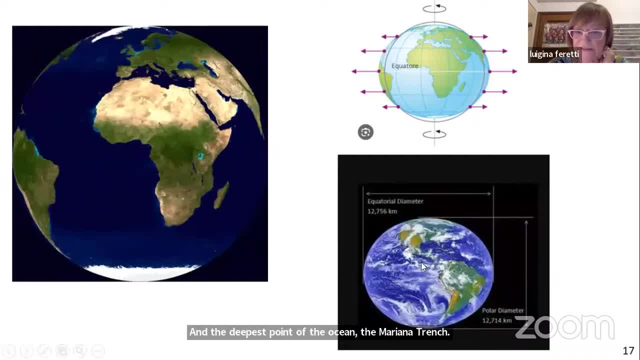 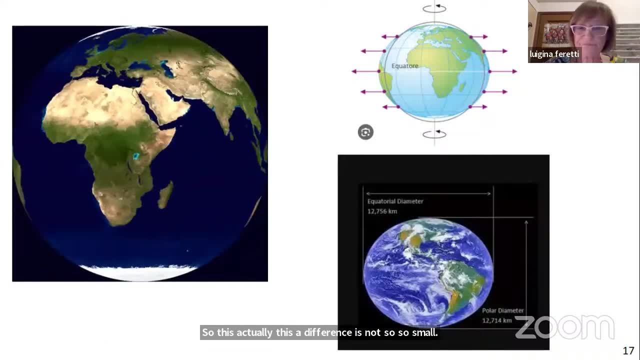 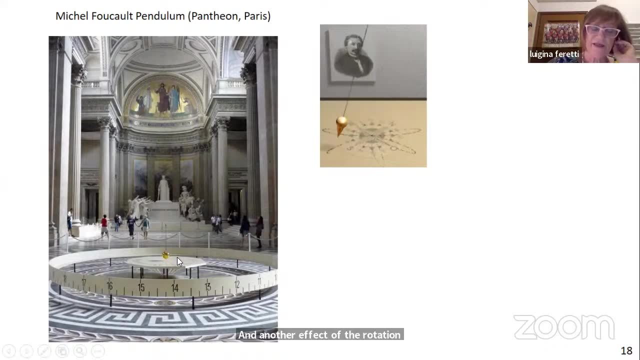 So this, actually this difference is not so, so small. I mean, it's completely discernable. Another effect of the rotation: the rotation of the Earth was demonstrated by M Foucault with the Foucault Pendulum. He demonstrated that the Earth was rotating by hanging a long pendulum. 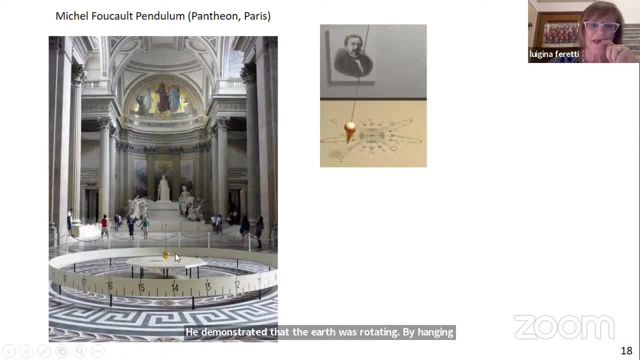 at the center of the Pantheon at Paris. GR K R He was hanging it at the center of Aparri. GR K R, He was hanging it at the center of Aparri. And since, according to the law of physics, 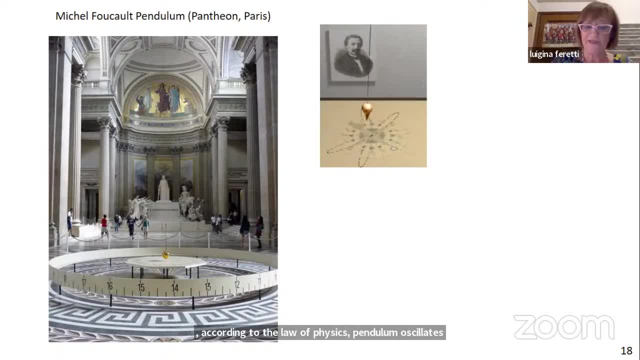 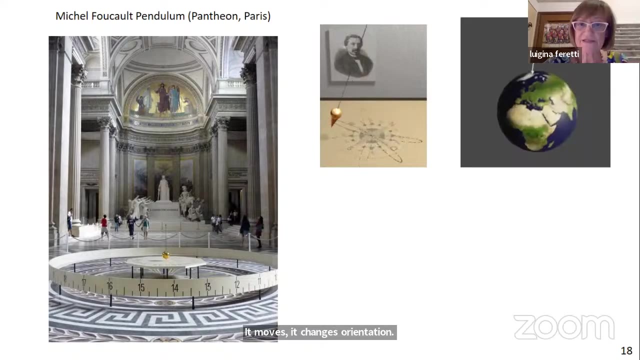 pendulum oscillates always on the same path, on the same plane. you could expect to see the pendulum always in the same plane. Instead, it does like this: It moves, it changes orientation. Why this? Because it is very simple to understand. 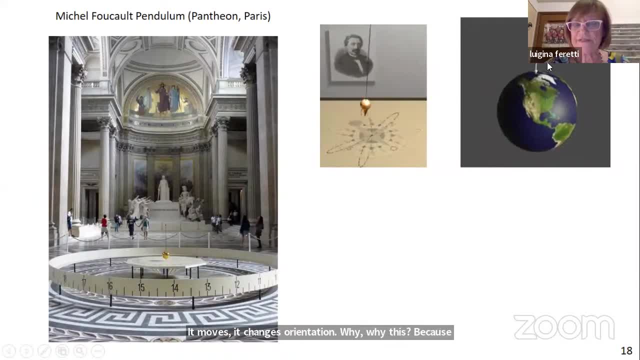 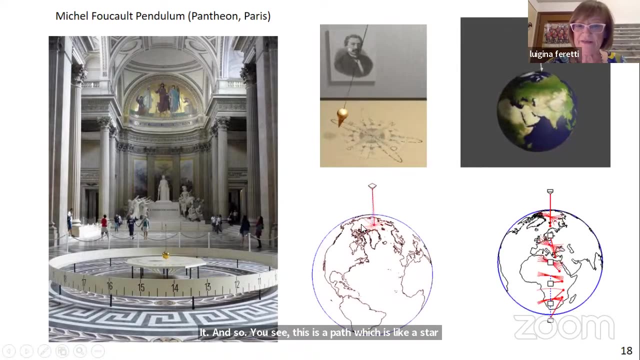 that the equator, the pendulum. the pendulum oscillates always in the same plane, but the Earth rotates beneath it, And so you see this path which is like a star, You see at the pole. it is very, very intuitive to understand. 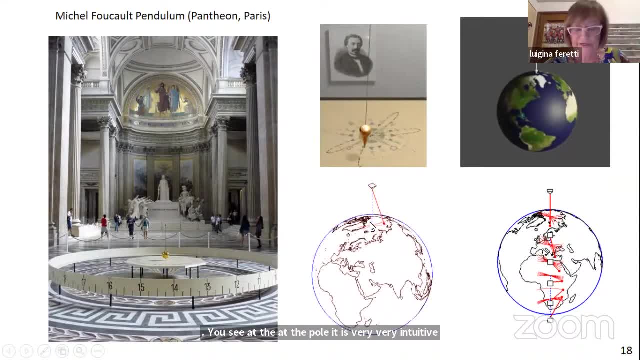 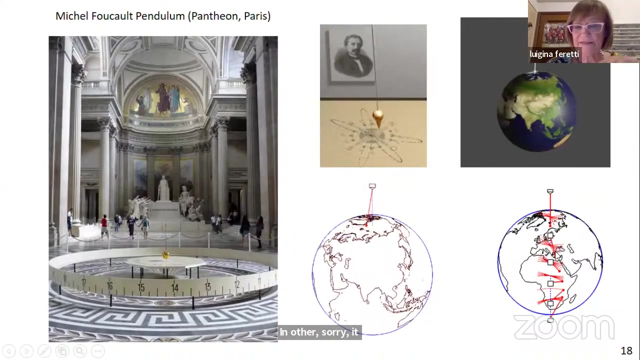 The Earth is rotating while the pendulum keeps always the same plane of oscillation. Oh dear In other. okay, I don't know why, let's see In other. sorry it doesn't work. In other latitudes the effect is not as big as at the pole. 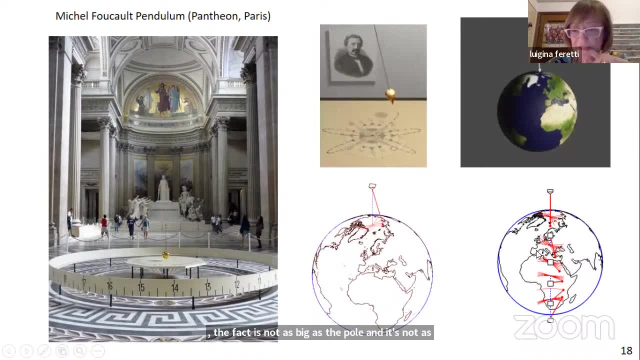 and is not as intuitive to understand as at the pole. But you have the same effect at several latitudes, except at the equator. At the equator The pendulum moves always in the same direction because the Earth keeps it in its rotation. 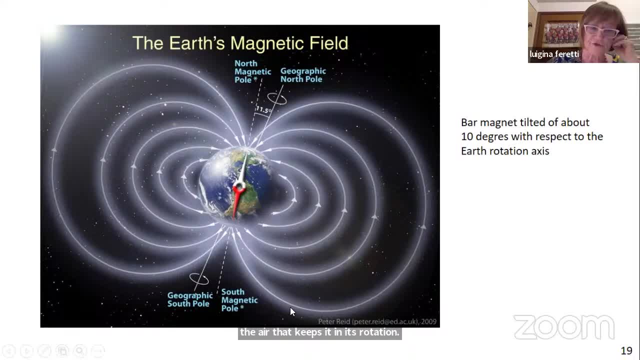 Another effect of the Earth rotation is the existence of a magnetic field. So the Earth behaves like a big compass with the northern pole magnetic pole and the southern magnetic pole, And these lines indicate the strength of the magnetic field, how it expands toward the space. 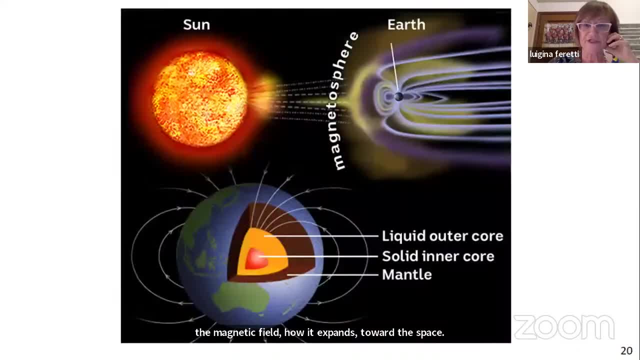 And it is very, very important because it shields the Earth. this magnetic field shields the Earth from the cosmic rays coming from the sun, from the radiation, the dangerous radiation, coming from the sun. So why is? what is the origin of the Earth? magnetic field? 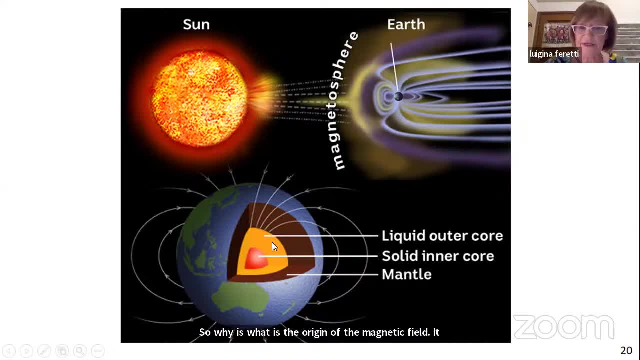 It is due to, due to the current which are in the liquid outer core, which is made of iron. The external part of the core of the Earth, which is here, orange, is dominated by iron, And so rotation of this core creates a current. 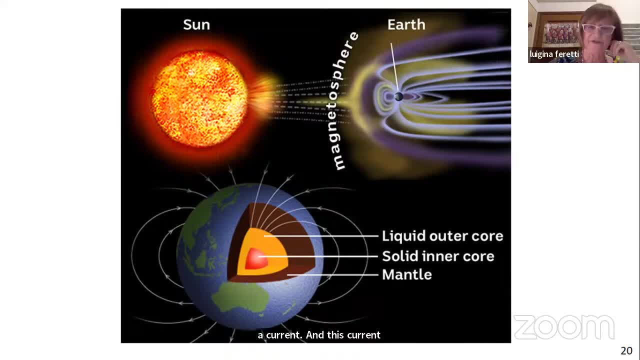 And this current creates the magnetic field, and this current creates the magnetic field. the magnetic field, the, the nucleus, these nucleus of of the earth, as well as other layers, rotate, change the rotation because of interaction with other layers, because of seismic activity, volcanic activity and also because of the interaction with the planet. 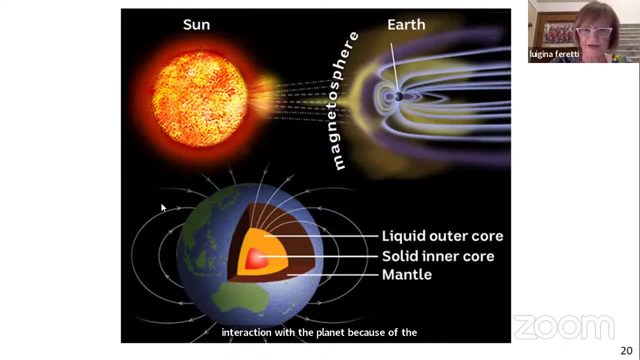 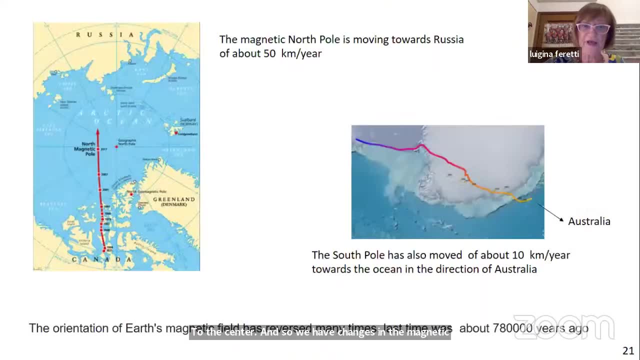 because of the gravitational forces which can arrive to the center, and so we have changes in the magnetic field. in particular, i can show you that the magnetic north pole is shown here- is moving toward russia of about 50 kilometers per year. you see, it was here in canada and now is close to the geographic pole. this is 2017. 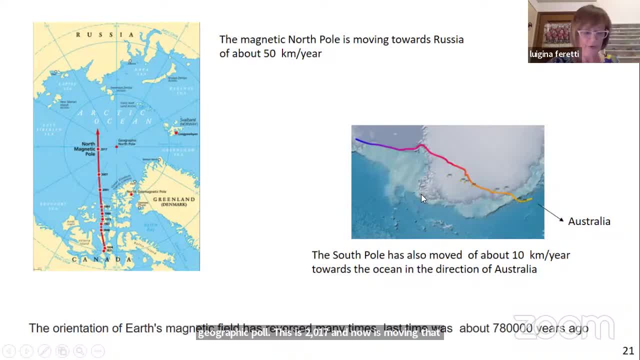 now is moving more, and also the south pole is moving slower, about 10 kilometers per year, but has moved toward through antarctica and is now in the located in the ocean in the direction of australia. and so these these changes are effect of the changes in the rotation of the. 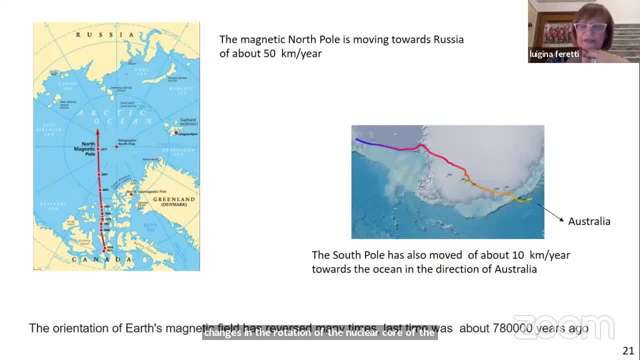 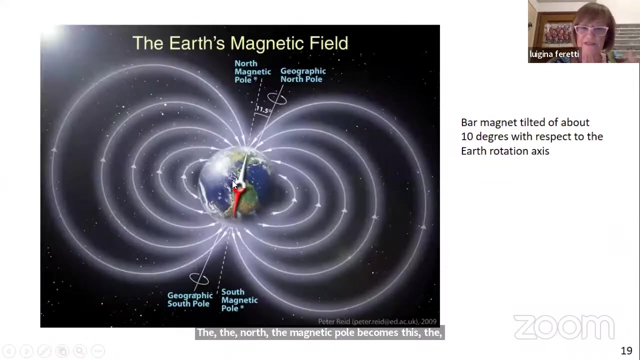 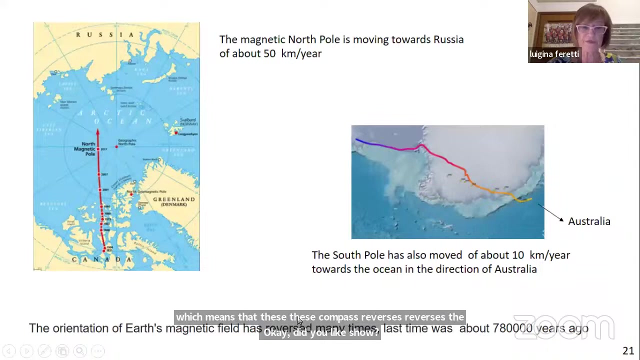 nuclear core of the earth. an extreme effect is a reversal of the two poles, that is, the north the magnetic pole becomes this, the southern magnetic pole, and the south magnetic pole becomes the northern pole, which means that these, these compass reverses, reverses the, the direction, and so reversals of the, of the magnetic poles of the earth have happened several times. 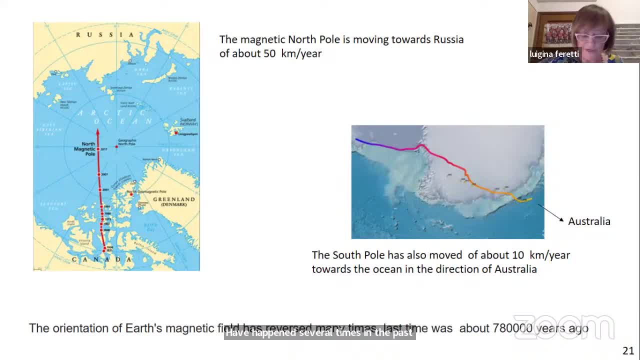 in the past um, but always, uh, irregularly. so they are not um irregular times and they. there have been about 200 reversals in 80 million years and there were 20 reversals in the last 5 million years. the last reversal occurred seven, eight hundred thousand years ago. 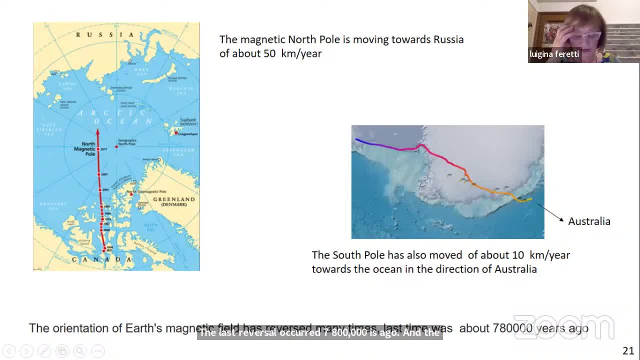 and it is still debated how long it took the reversal to take place. it seems that it took, okay, between two thousand years and twelve thousand years. so the reversal of the polarization of the earth magnetic field is a really a very slow process. we do not expect a flip. 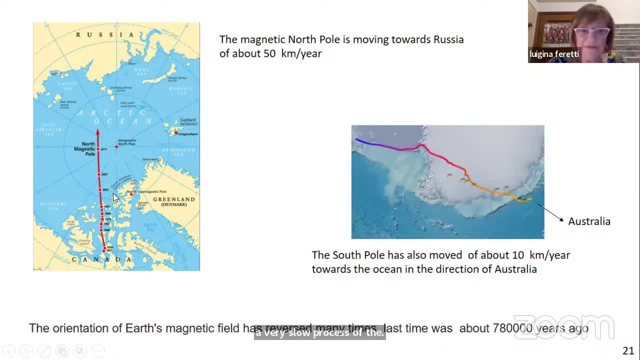 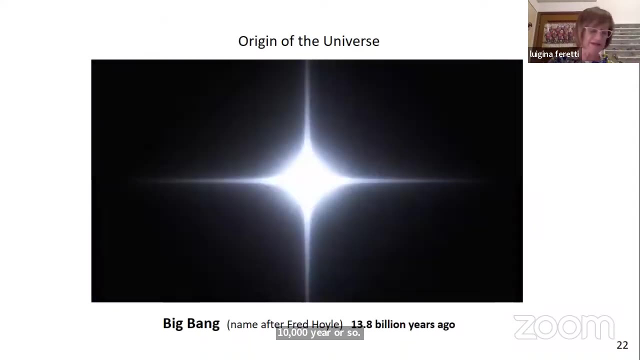 see what happens. it is very, very slow. so maybe this motion that i showed are just the beginning of a slow reversal that will take place in 10 000 years or so. and now i i want to show you some, to give you some information about the origin of the universe. 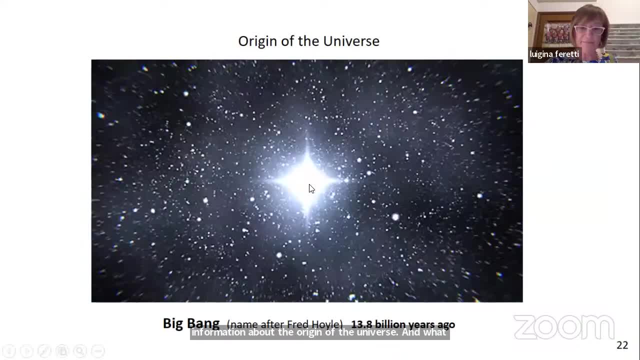 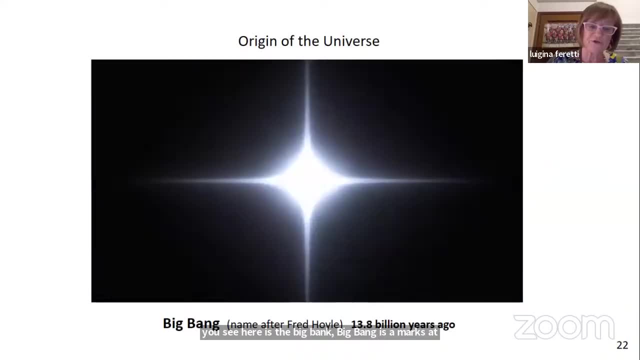 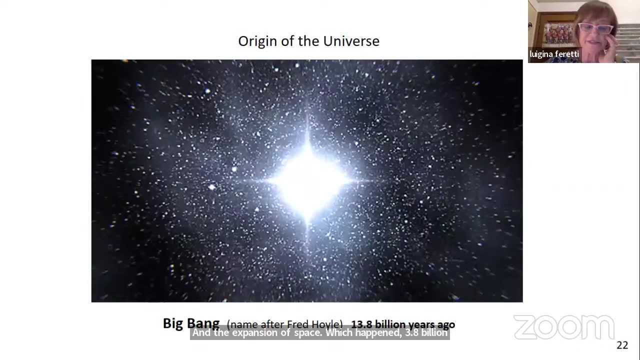 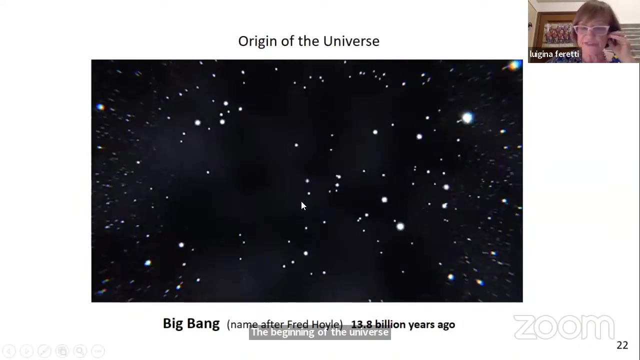 and what you see here is the big bang. big bang is marks the birth of time and the expansion of space, which happened 3.8 billion years ago. this is the beginning of space and time, the beginning of the universe. universe, um, it cannot be this. the physics cannot describe what happened in the first. 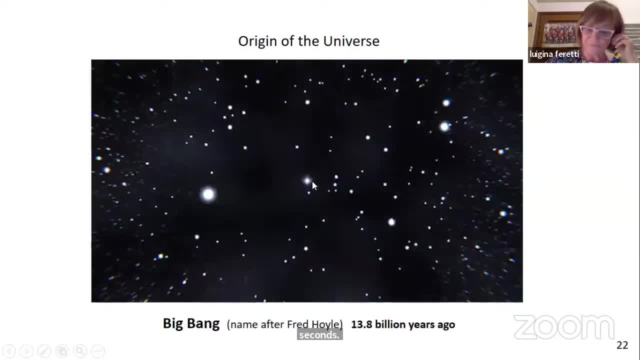 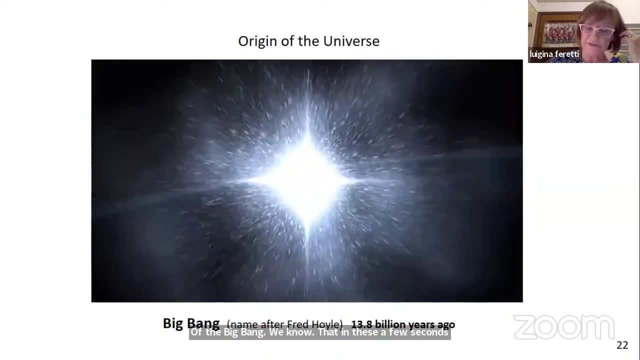 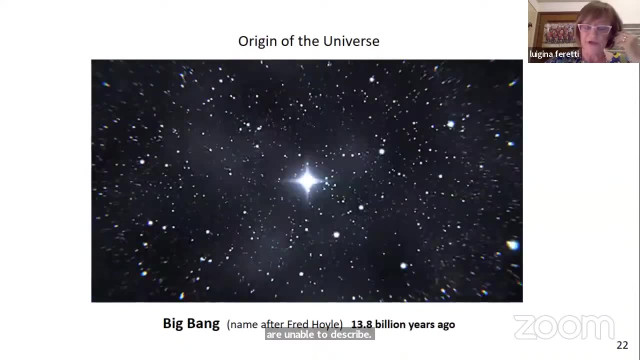 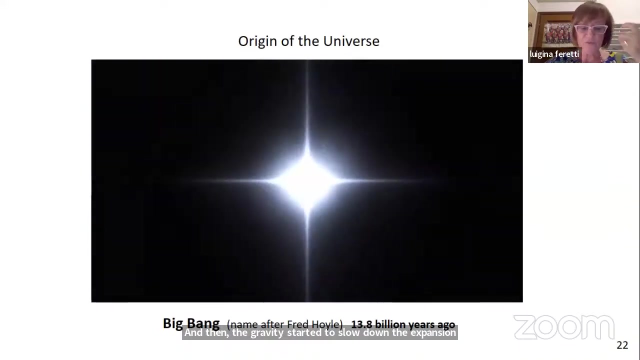 seconds of the big bang. we know that in these a few seconds there was a big, big expansion, at the velocity that we are unable to describe, and then gravity started to slow down the expansion, the temperature decreased and the elementary particle start to be created, and we have 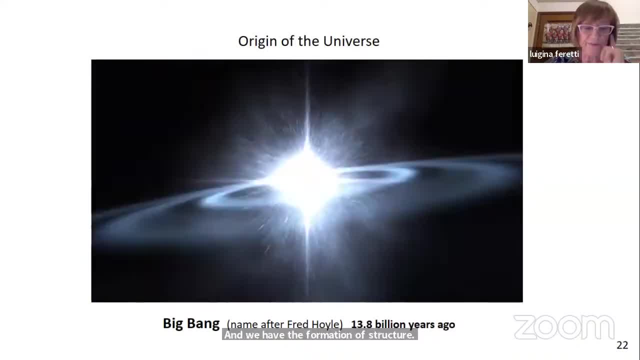 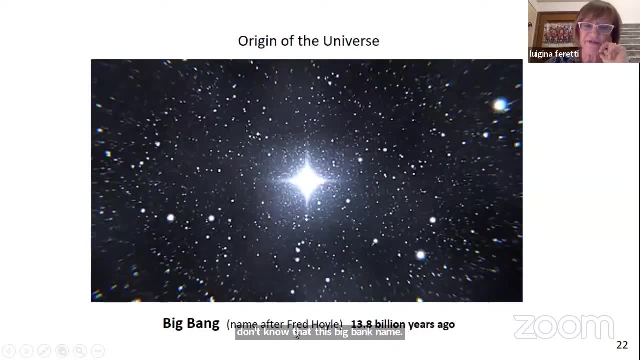 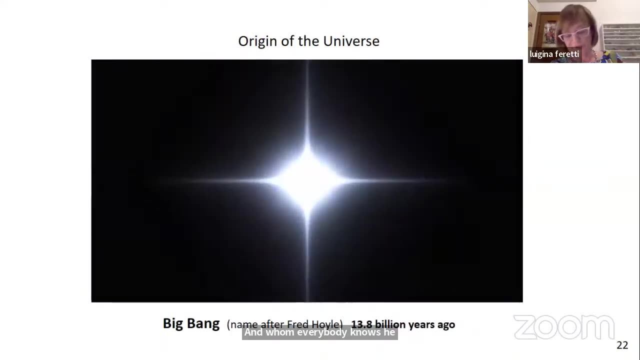 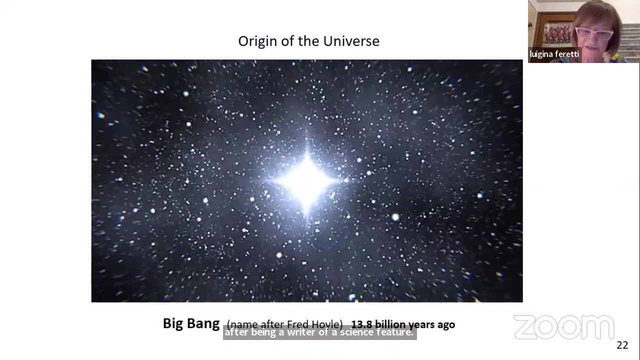 the formation of structure. maybe people don't know that this big bang name was given by fred hoyle, whom everybody knows. he was an astrophysicist, but after being a writer of science fiction, uh, he was also an astrophysicist and he he was against the big bang theory. so when? 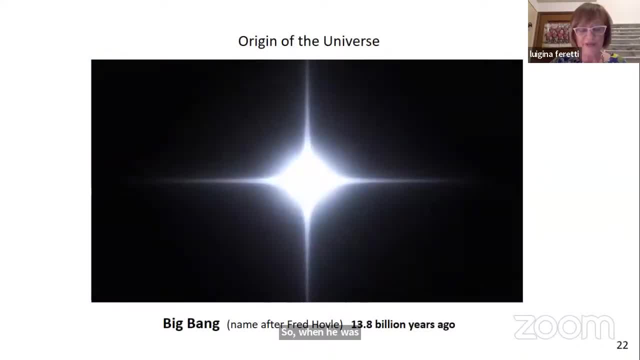 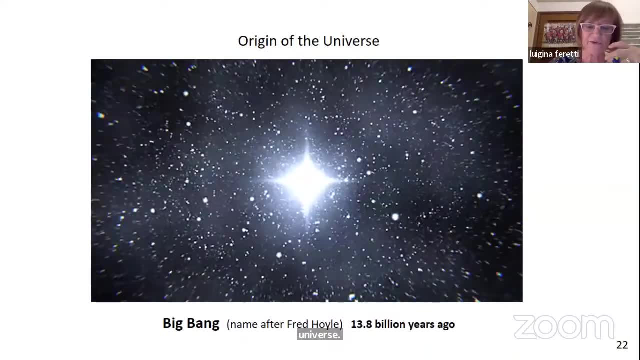 he was interviewed, he was against the big bang theory. so when he was interviewed, he was against the big bang theory. so when he was interviewed by the bbc to explain his idea of the universe, he mentioned the big bang, used the term big banger to, with the derision to the, to describe the theory that he did not accept. 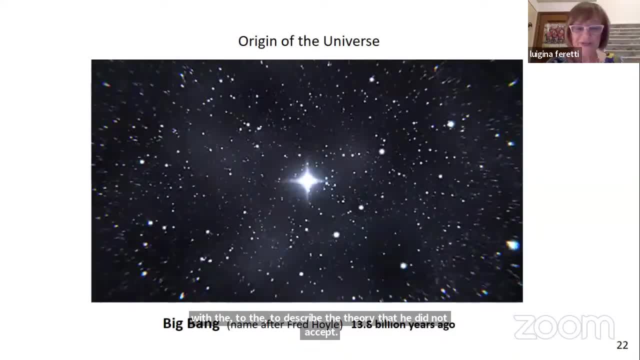 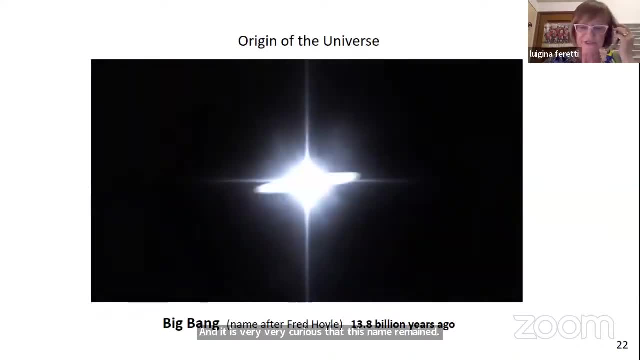 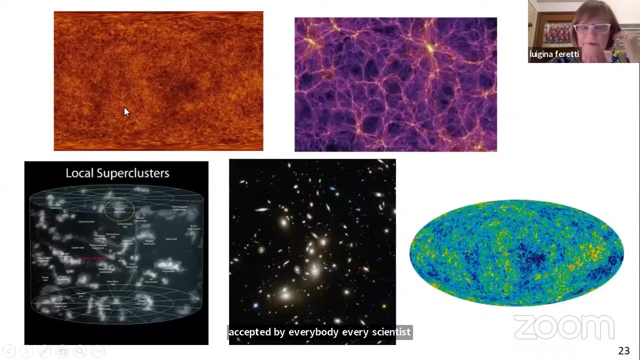 and that it is very, very curious that this name remained to, to, to characterize the model of universe that now is commonly accepted by, by everybody, every scientist, so the. after the big explosion, the structure started to, to, to form because all the particles were attracted, and we know that matter was not uniform. it was not uniform, there were small. 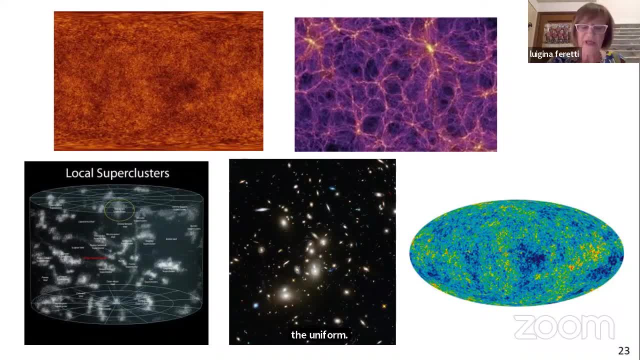 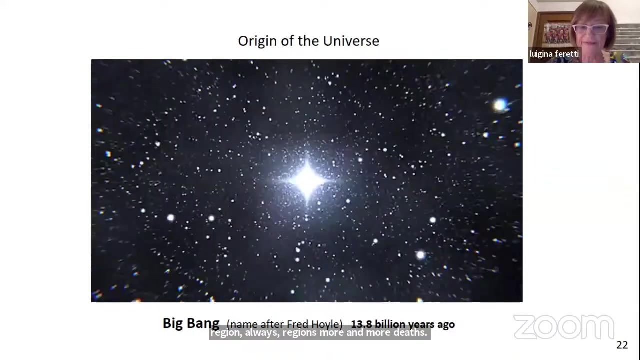 small pieces of these, these homogeneities, and if the particles were motionless, they could. all the particles would simply fall one into the other and go to dance a region to dance a region, always regions more and more dense. but we know that they were, they had a. 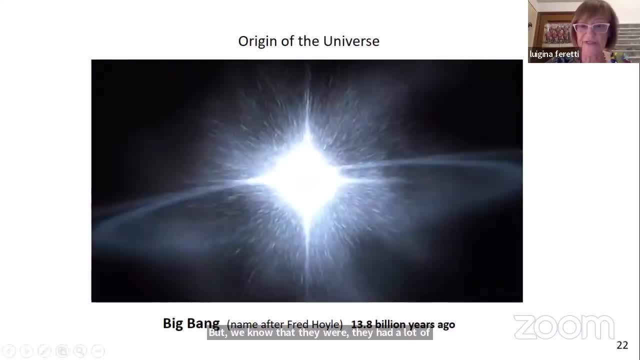 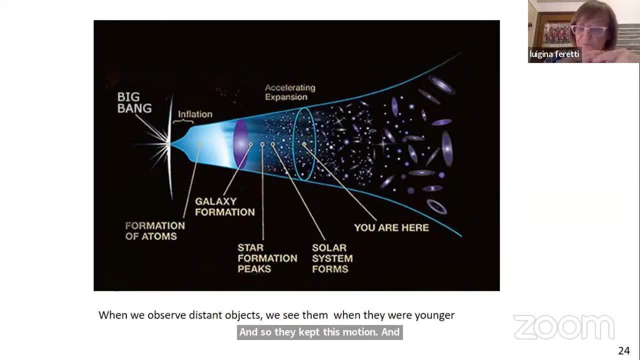 lot of motion of the particles, as you see in in this cartoon, and so they kept this motion, and gravity turned this motion into orbital motions. that's why every object in the universe move, rotates, because the particles that were created at the big bang had a linear motion, and gravity turned this linear motion into orbital, into orbital motion. so 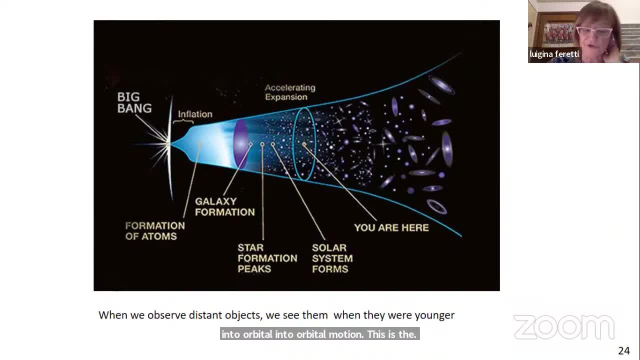 So this is the explanation of the formation of stars, galaxies and various objects that had some in physics we call angular momentum, so the capacity of rotate. This is a scheme, a cartoon of the Big Bang. You see the big explosion here, quick expansion, and then the matter starts to aggregate. 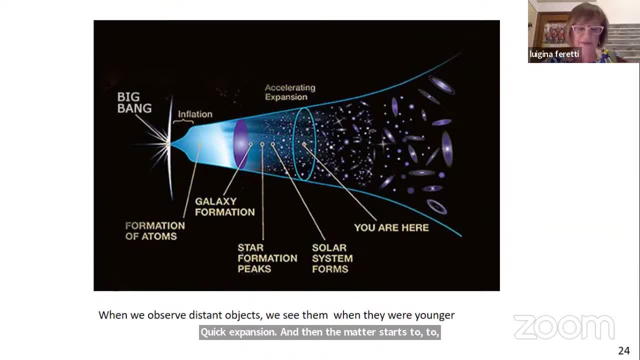 and objects more and more big are formed. The process is very slow. We are now here About Here, And the universe is now expanding again, So it has accelerated its expansion. It's not going at the same velocity, but it is accelerating. 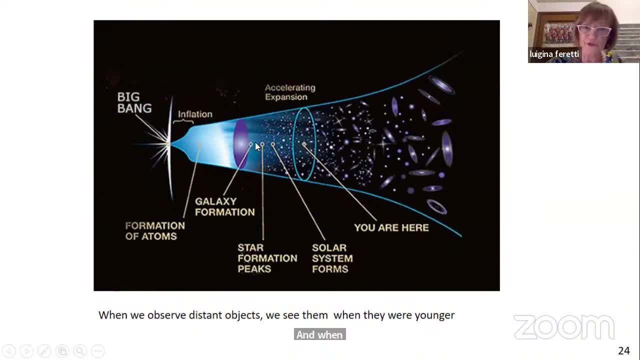 And when we are here and we observe the object far away toward the Big Bang, we see them when they were younger because we see them through the light that they emit. light has a velocity of 300,000 kilometers per second, but it's not the infinity. 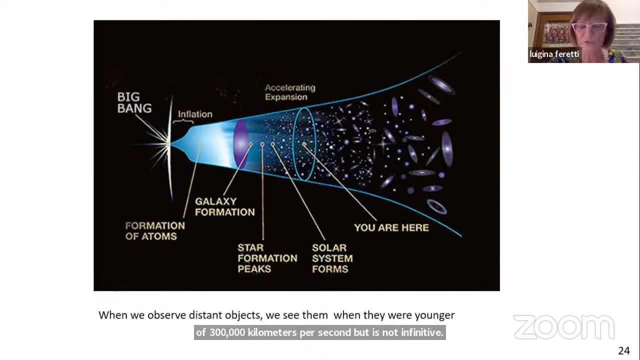 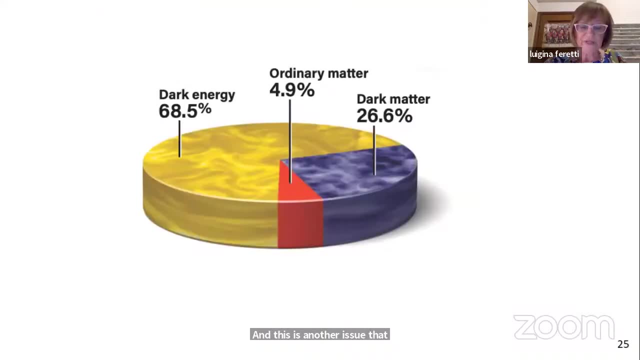 So it takes time for the light to cross the universe. So when we observe distant objects, we see them when they were younger, And this is another issue that maybe one doesn't think about. in the process of the formation of the universe- And an important- the dominant ingredient is the dark matter. is the dark matter? 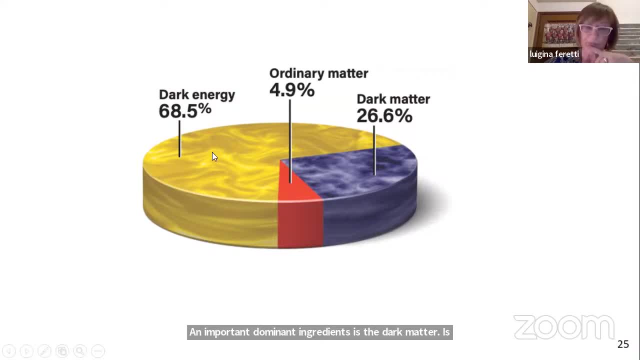 And that is the dark energy. Dark energy is the energy that is now producing an acceleration of the universe, While the dark matter is a matter that we don't know and is about 80% of all the matter in the universe. So the ordinary matter is 20% of all the matter. 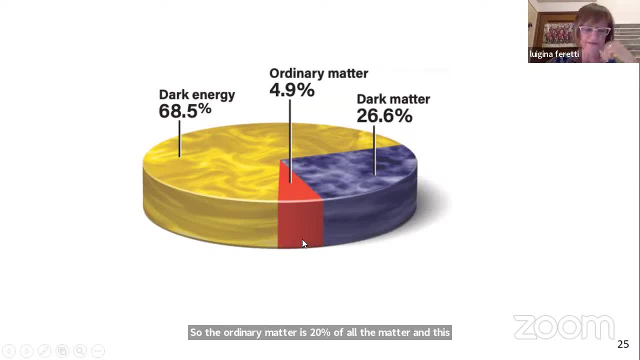 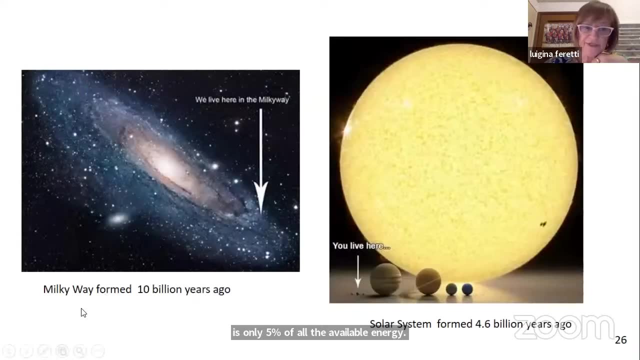 and is only 5% of all the available energy. Just to say that the Milky Way formed 10 billion years ago and we are here. so we are in an arm, we are not at the center, And here is a picture of the solar system. 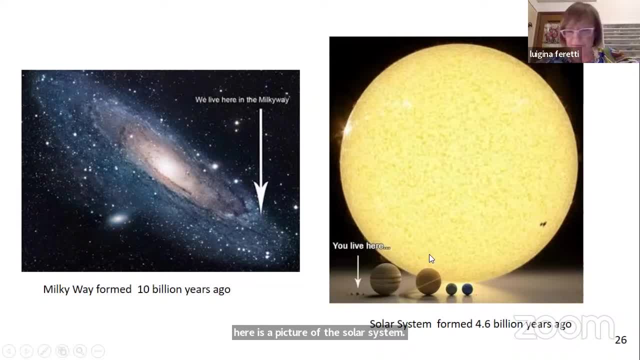 or not, the solar system of the sun and of the planets depicted into scale. So you see how small we are. The solar system formed much later than the galaxy, the Milky Way that we belong to. It formed 4.6 billion years ago. 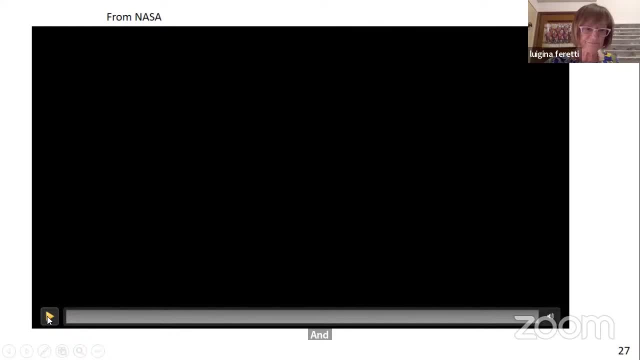 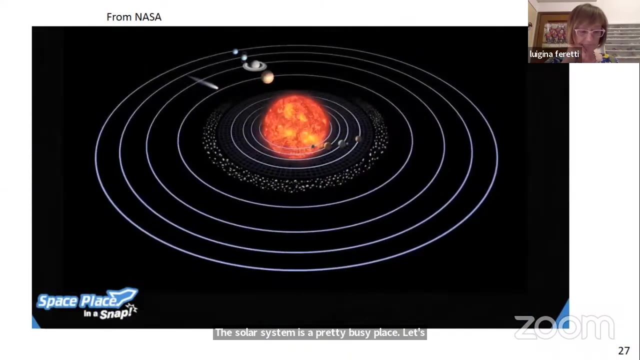 Another video about the formation of the solar system Space place. This is very, very simple, From NASA. How did our solar system come to be? The solar system is a pretty busy place. It's got all kinds of planets, moons, asteroids. 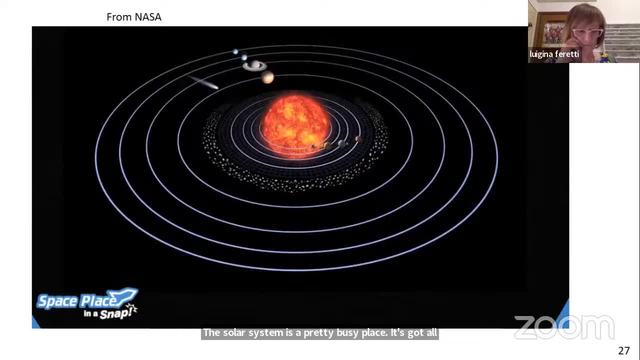 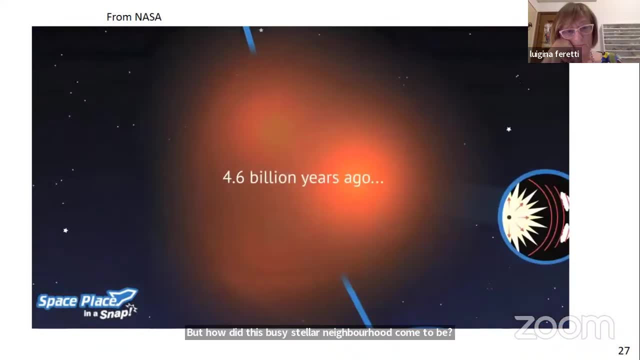 and comets zipping around on the sun. But how did this busy stellar neighborhood come to be? Our story starts about 4.6 billion years ago with a wispy cloud of stellar dust. This cloud was part of a bigger cloud. 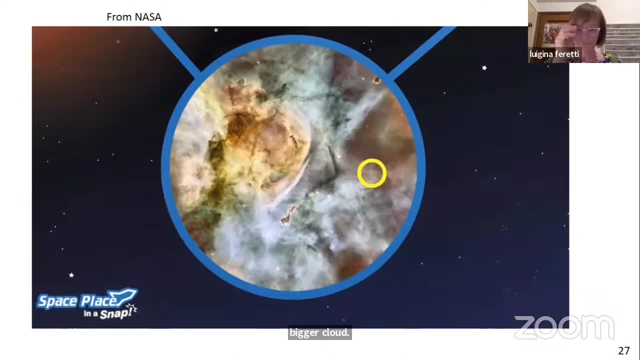 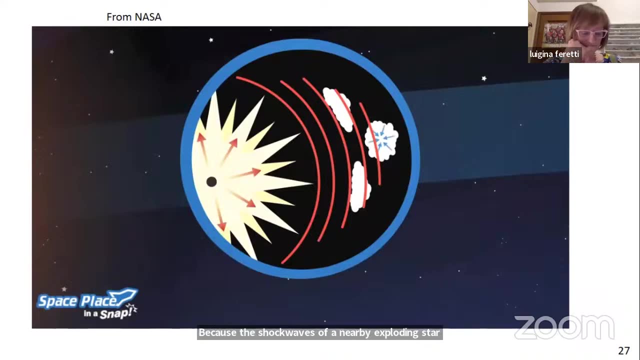 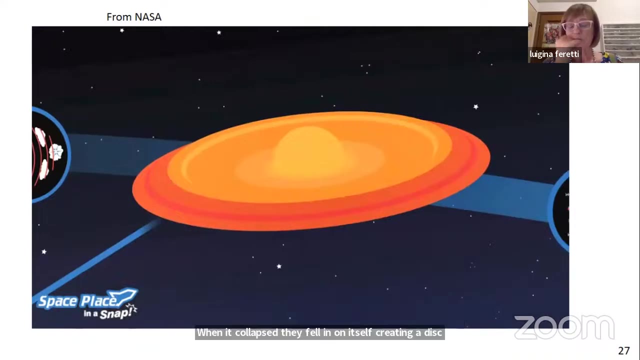 called a nebula. At some point, the cloud collapsed, possibly because the shockwave of a nearby exploding star caused it to compress. When it collapsed, it fell in on itself, creating a disk of material surrounding it. Finally, the pressure caused by the material was so great. 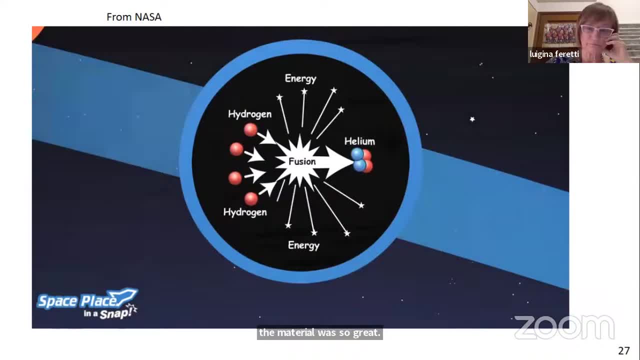 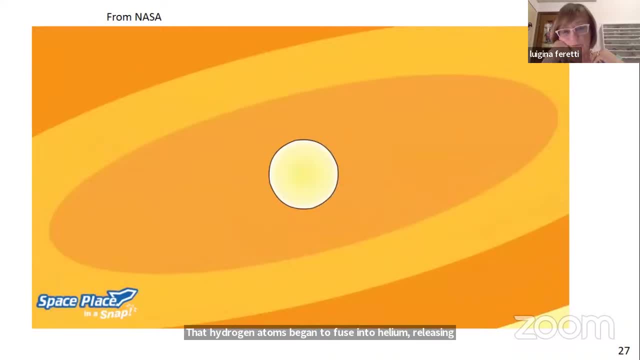 that hydrogen atoms began to fuse into helium, releasing a tremendous amount of energy. Our sun was born. Even though the sun was so bright. it was still so bright, Even though the sun gobbled up more than 99% of all the stuff in this disk. 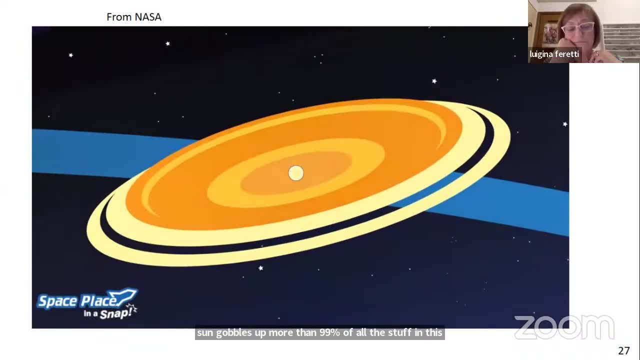 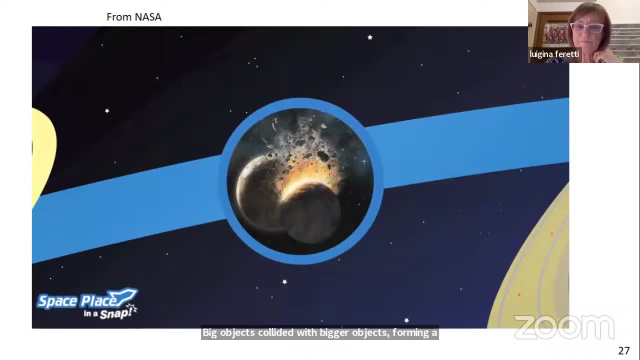 there was still some material left over. Bits of this material clumped together. because of gravity. Big objects collided with bigger objects, forming still bigger objects. Finally, some of these objects became big enough to be spheres. These spheres became planets, dwarf planets. 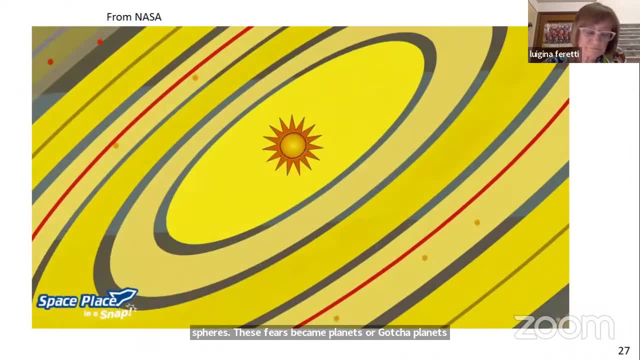 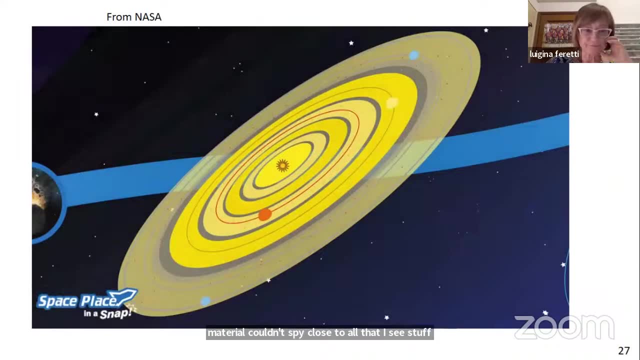 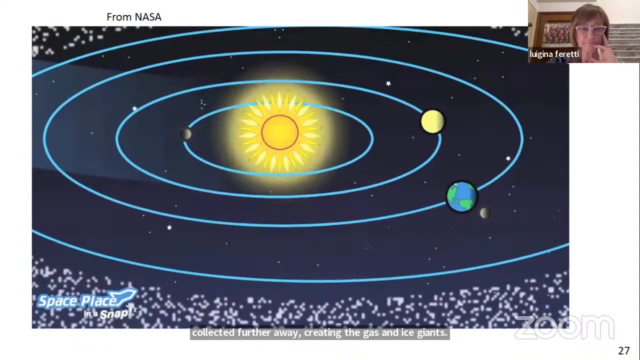 Rocky planets like Earth formed near the sun because icy and gaseous material couldn't survive close to all that heat, Gas and icy stuff collected further away, creating the gas and ice giants, And like that the solar system as we know it today was formed. 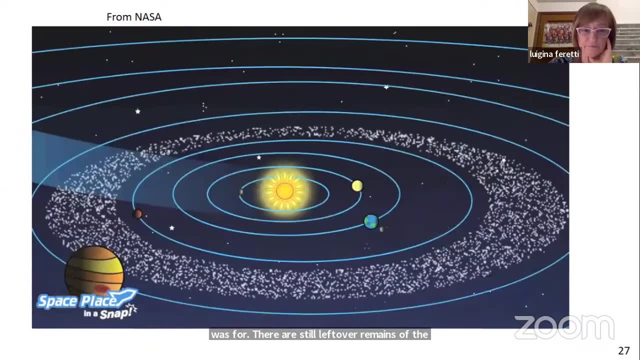 There are still leftover remains of the early days, though. Asteroids in the asteroid belt are the bits and pieces of the early solar system that can never quite form a planet. Way off in the outer reaches of the solar system are comets. 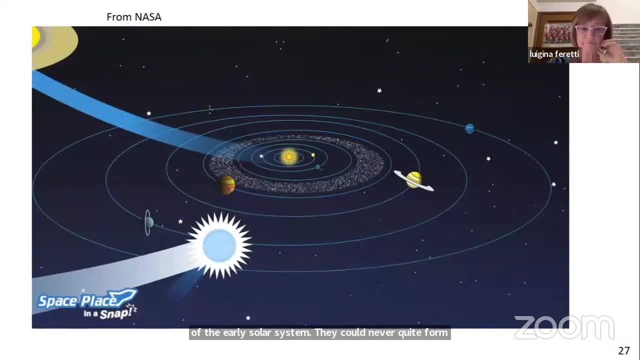 They can never quite form a planet. Way off in the outer reaches of the solar system are comets. These icy bits haven't changed much at all since the solar systems formation. In fact, it is the study of asteroids and comets that allows scientists to piece together this whole long story. 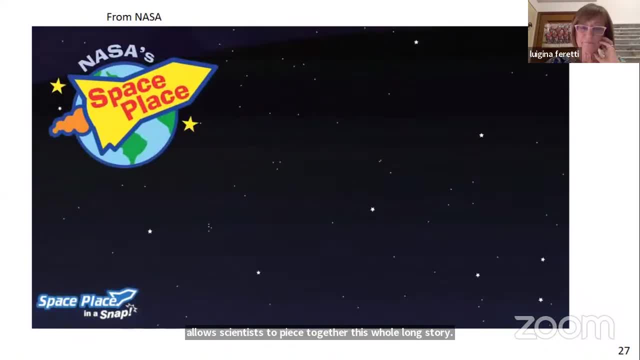 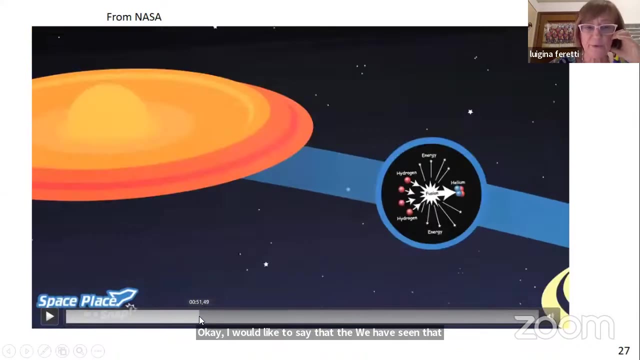 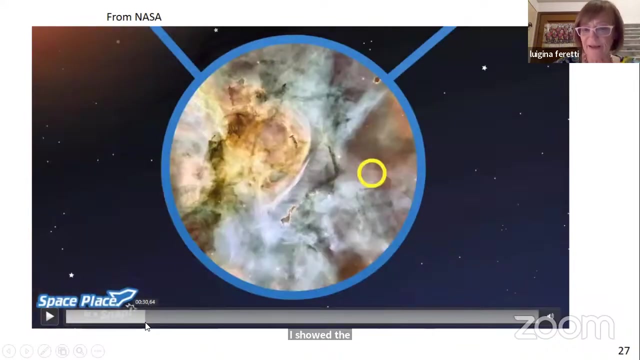 Brought to you by Nasa Space place. Okay, um, I'd like to say that the eh we have seen when I showed, uh, the gravitation works on larger scales. I showed some of the nebulae that are a cradle. 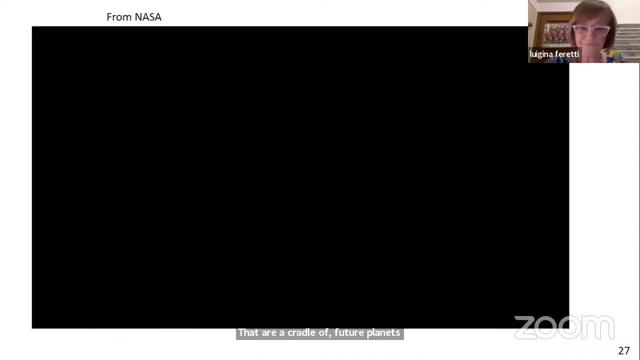 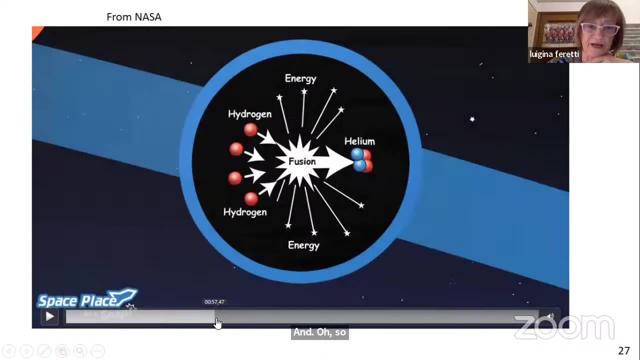 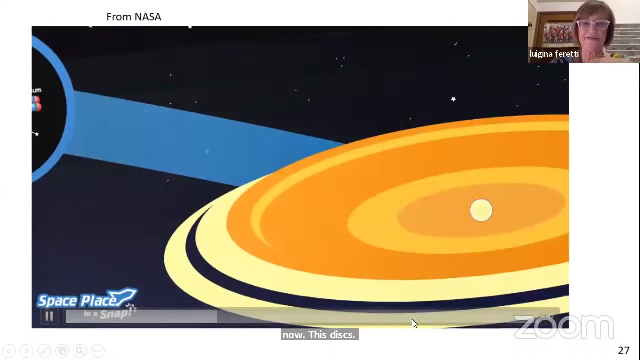 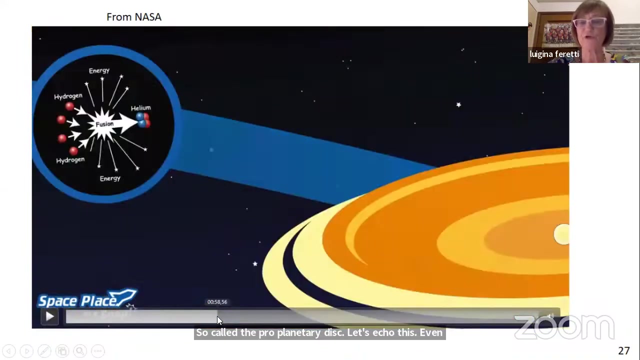 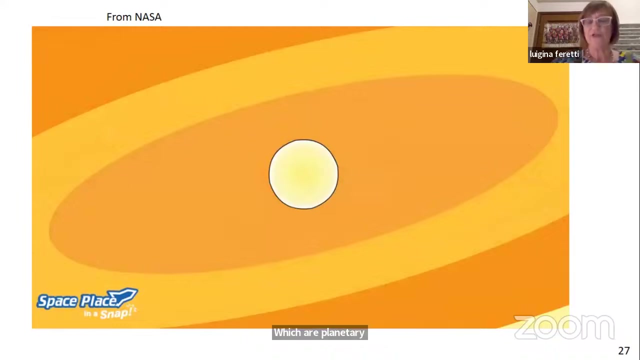 of future planets. And also, I'd like to point out that we are observing now these disks, so-called protoplanetary disks. Let's echo this: It is possible to observe disks around the stars, which are planetary systems in formation, All of them. 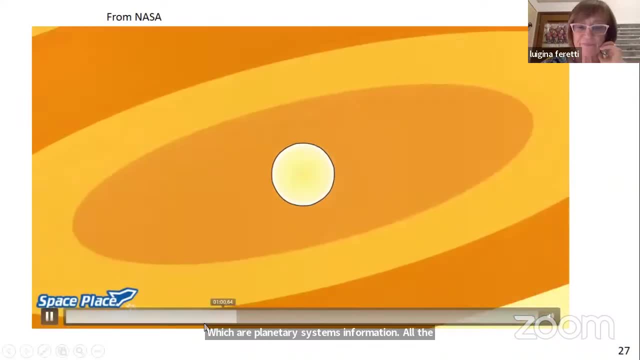 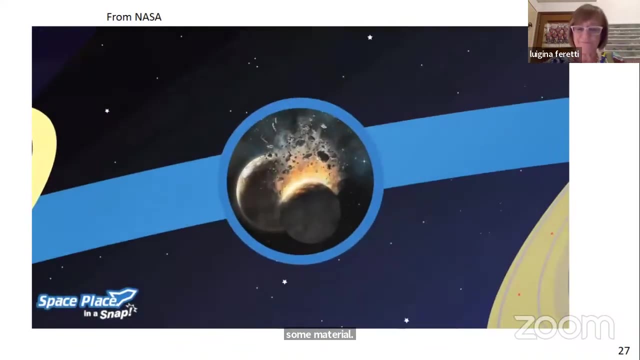 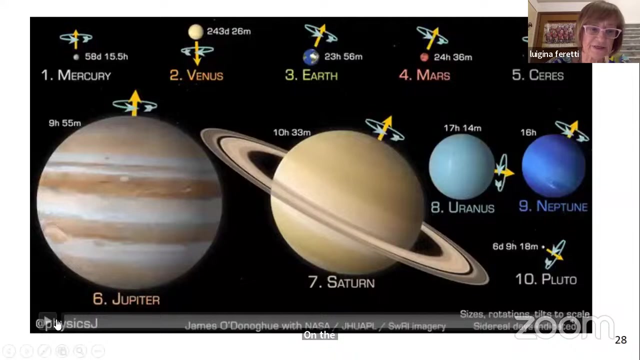 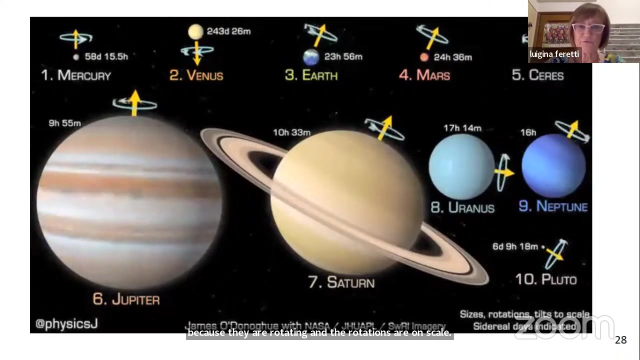 There are several things in this. This is a protoplanetary disk and they are commonly observed in the universe, So this is a picture of the planets I like, because they are rotating and the rotations are on scale, So you see those who rotate very quickly. 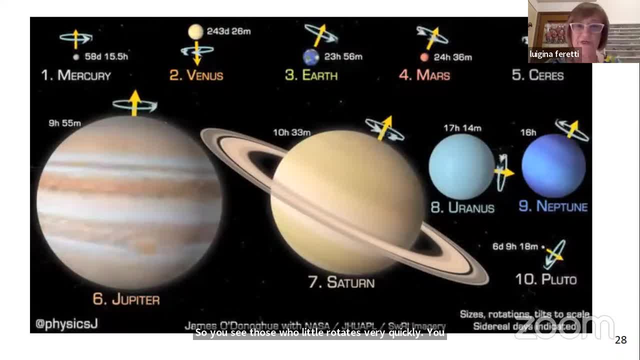 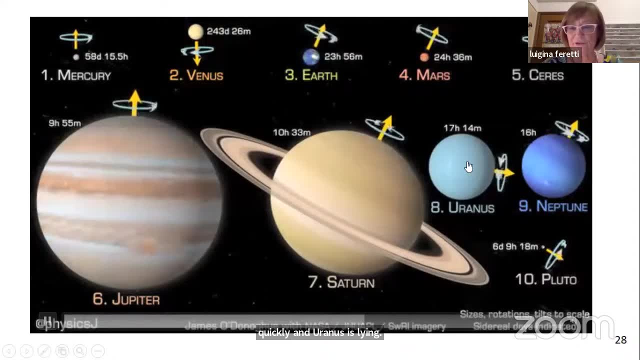 You know, Jupiter is very, very big and rotates very, very quickly, And Uranus is lying on the orbit so it rotates around the direction of the motion, And these Mercury and Venus are too slow so they are not shown rotating. you see these? 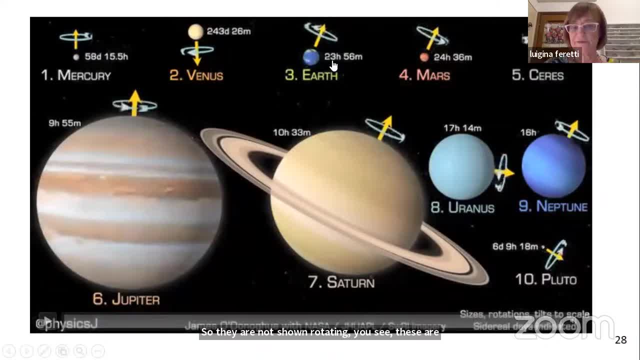 243 days while they are rotating. So you see those who rotate very quickly. You know, Jupiter is very, very big and rotates very, very quickly. Earth is 23 hours, So we have seen in the movie how the planet forms. 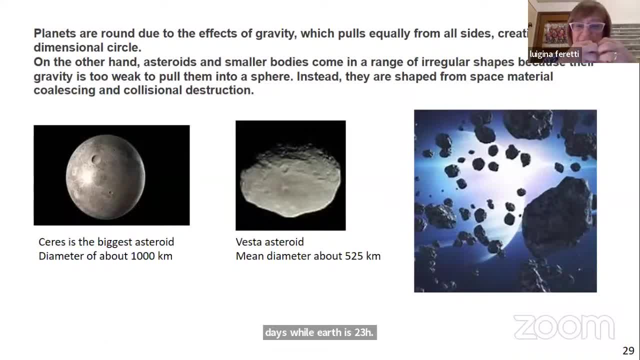 And again I wish to stress that the planets are round due to the effect of gravity, which pulls equally from all sides, creating a three-dimensional sphere, not a circle. On the other hand, there are in the solar system asteroids and stars and planets, and 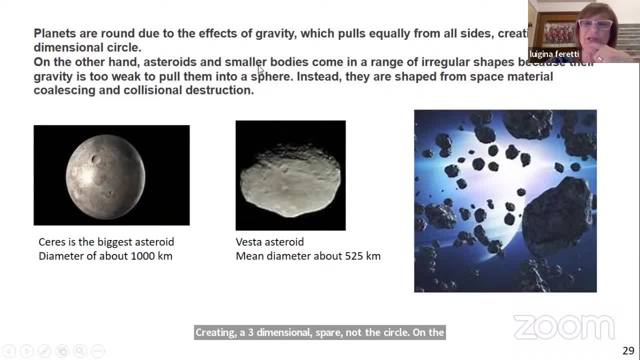 planets, asteroids and smaller bodies that come in a range of irregular shapes because their gravity is too weak to pull them into a sphere. So the sphere is the shape of the big objects due to gravity and they are spherical due to the gravitation. But the smaller bodies have irregular shapes because the gravity is not strong enough to give them a spherical shape. 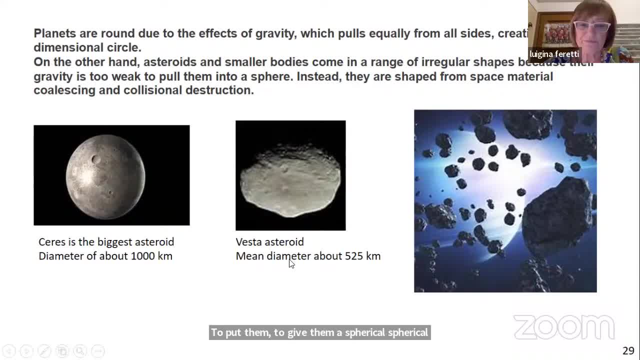 So this is the Vesta asteroid, which has a mean diameter of 500 km and is irregular. While the Vesta is irregular, Ceres, which is the biggest asteroid, has a diameter of about 1000 km and it is round. 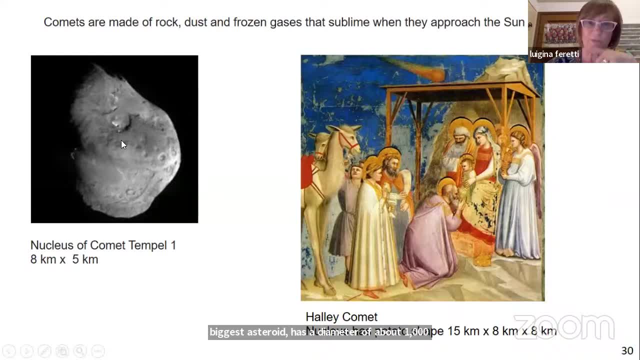 While Vesta is not round. And again, comets are made of rock and they are quite small. The cores of the comets are quite small. This is the nucleus of a Tempel 1, which is 8 times 5 km. 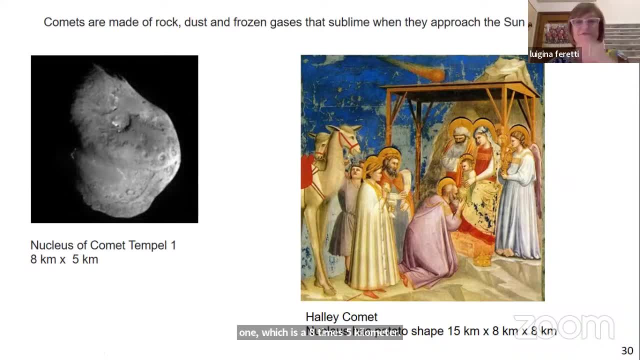 So too small to make a comet, So too small to make a comet And the Halley comet. I didn't find a photograph of the nucleus. The nucleus has a potato shape: 15 km times 8 times 8.. So I put a picture of Giotto. 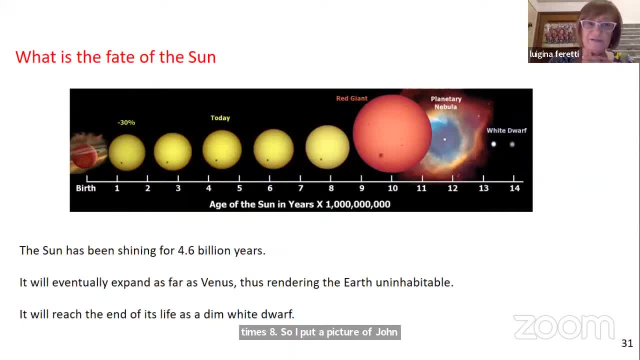 And going to the Sun. what is the fate of the Sun? The Sun has been shining for 4.6 billion years. The Sun has been shining for 4.6 billion years And today is the year. this is the birth of the Sun, as you have seen in the video. 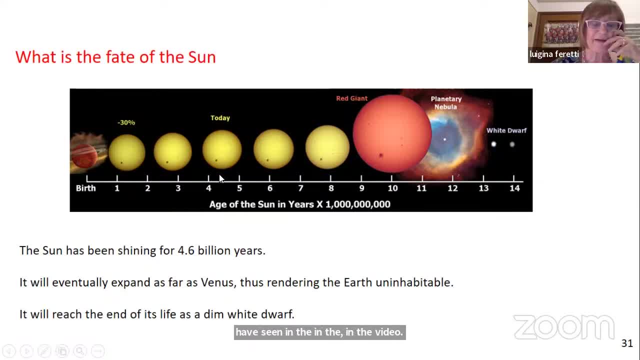 And now today we are almost here, 4.6 billion years. The fate of the Sun is to expand, It is to continue the activity in the center, the nuclear reactions in the center, And then at a certain point, about 4 billion years from now. so we are not worried about this. 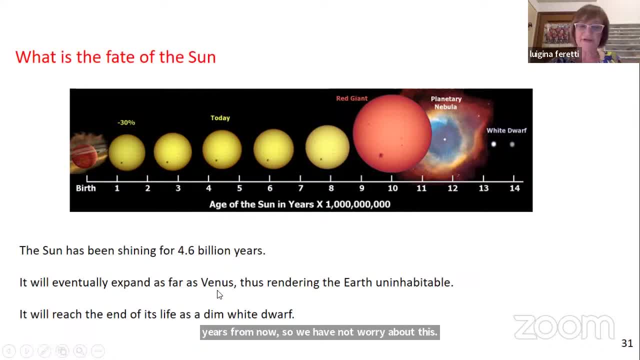 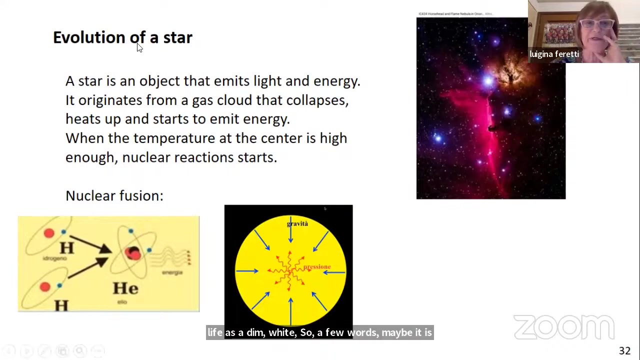 it will expand as far as Venus, thus rendering the Earth inhabitable. So it will expand, So it will expand, And then it will reach the end of its life as a dim white dwarf. So a few words. maybe it is useful to say a few words about evolution of a general star, not just the Sun. 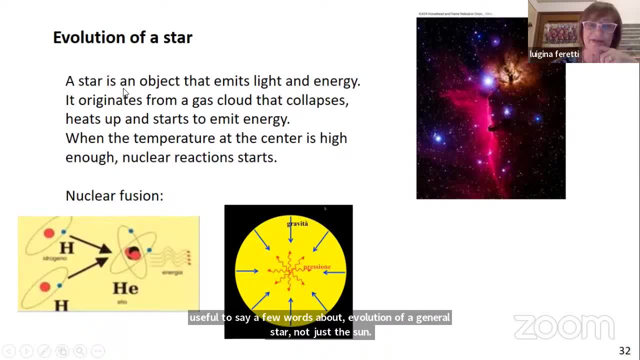 The star we know emits light and energy, And these light and energy originate from from a nuclear reaction at the center. At the center there is the hydrogen that fuses together with the reaction, which is the nuclear fusion. Two atoms of hydrogen fuse together to give an atom of helium. 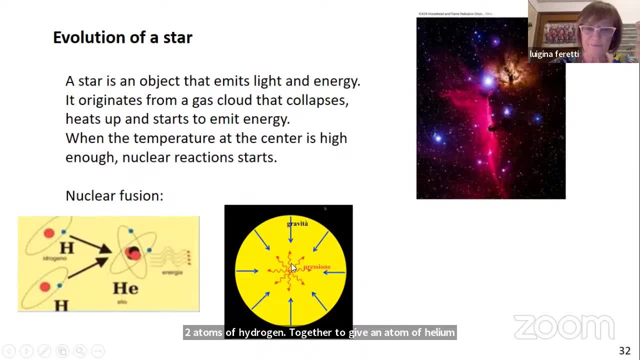 And this reaction at the center provides enough pressure to counterbalance the gravity. And this reaction at the center provides enough pressure to counterbalance the gravity. So the Sun is stable. So the Sun is stable, It doesn't collapse before of gravity, It doesn't expand because of the pressure of the nuclear reaction. 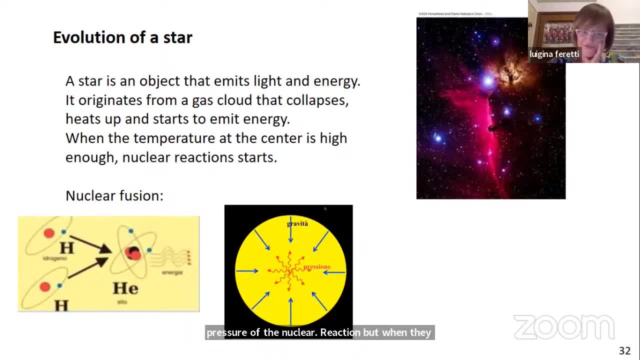 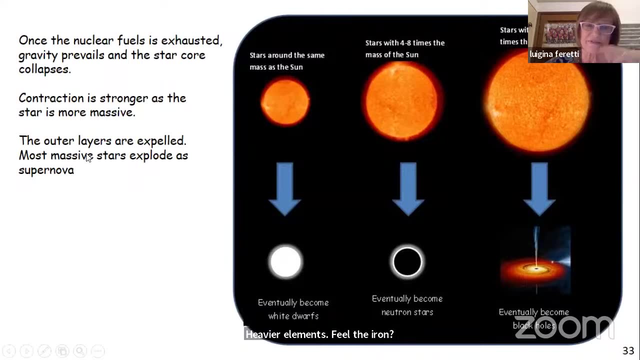 But when the hydrogen will finish, there will be other nuclear reactions involving heavier elements till the iron. But when the hydrogen will finish, there will be other nuclear reactions involving heavier elements till the iron. But when the hydrogen will finish, there will be other nuclear reactions involving heavier elements till the iron. 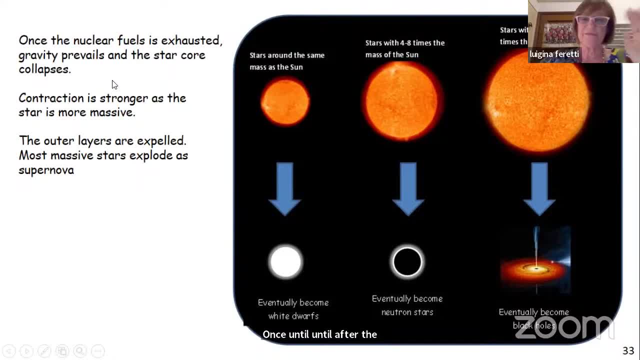 After the iron nuclear reaction. the nuclear fusion doesn't produce energy anymore, So the reaction stop And at this point the nuclear fuse is exhausted, Gravity prevails And the star core starts to collapse. The star core starts to collapse, while the outer layers will be expelled. 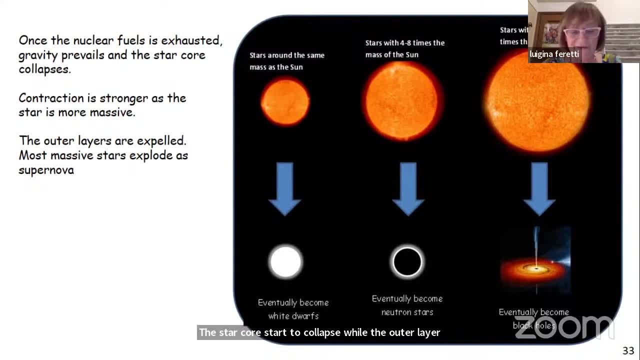 And this is why the Sun will expand up to at least the orbit of Venus. The contraction is stronger as the star is more massive. We will have stars as small as the Sun, which will become, as I said before, white dwarfs. 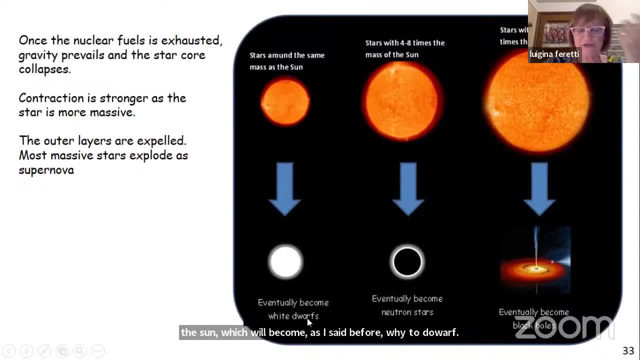 Which are cold stars which are not emitting any radiation. Stars with 4-8 times the mass of the Sun will become neutral stars And they will explode as a supernovae, And stars with more than 8-10 masses of the Sun will collapse with the extreme force of gravity. 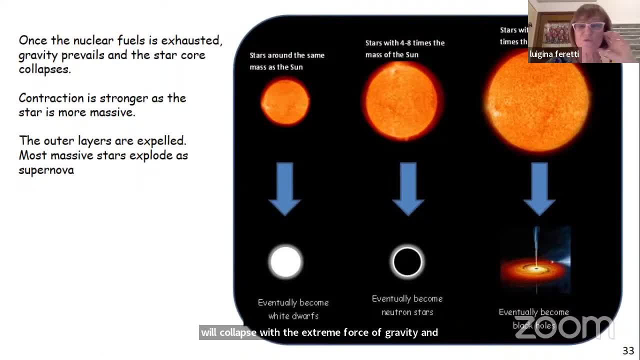 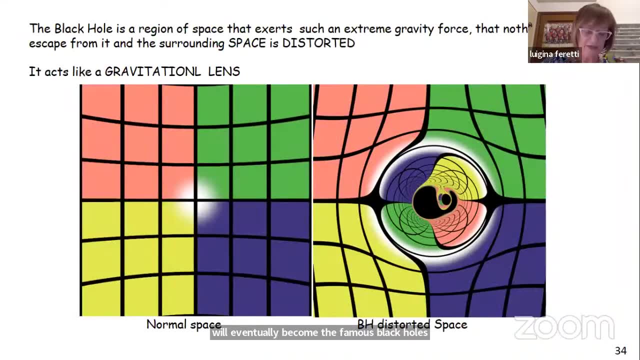 And will eventually collapse And will eventually collapse And will eventually become the famous black holes. So, Adriano is it. Can I have 5 more minutes to say something about the black holes? Yes, yes, of course The director is fantastic. 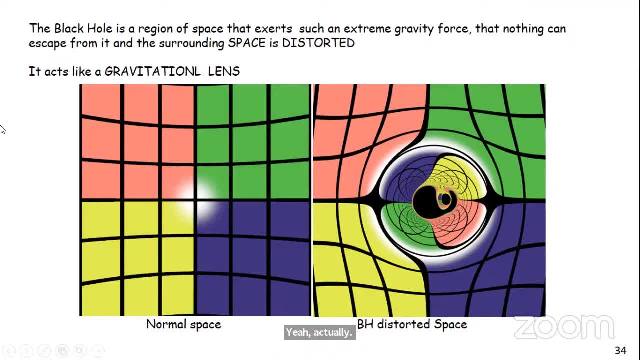 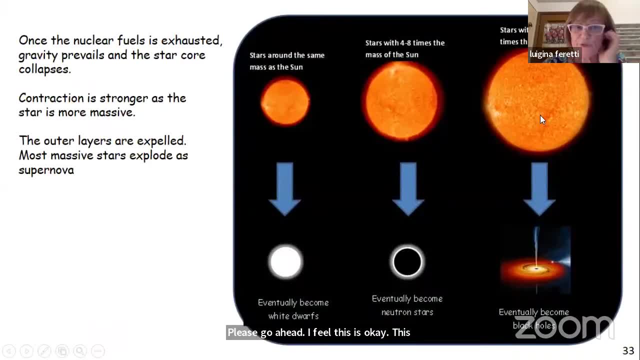 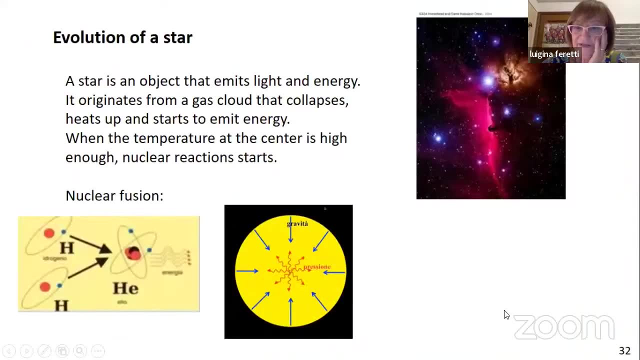 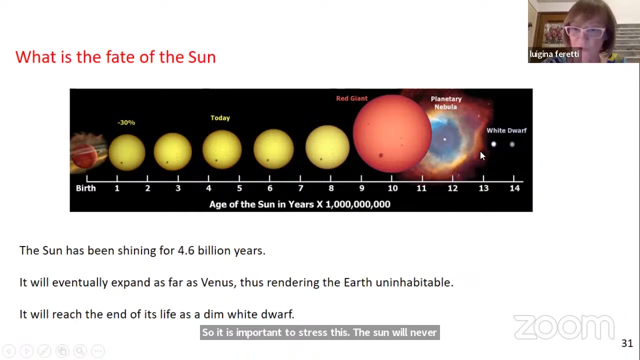 And we don't want to cut you. Please go ahead. Yes, finish it simply. So the black hole is produced at the end of a star much more massive than the Sun. So it is important to stress this: The Sun will never become a black hole. 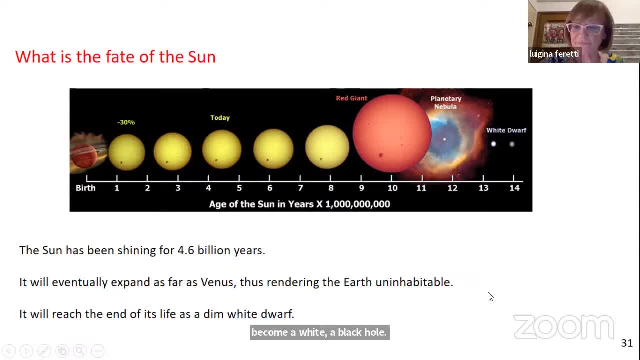 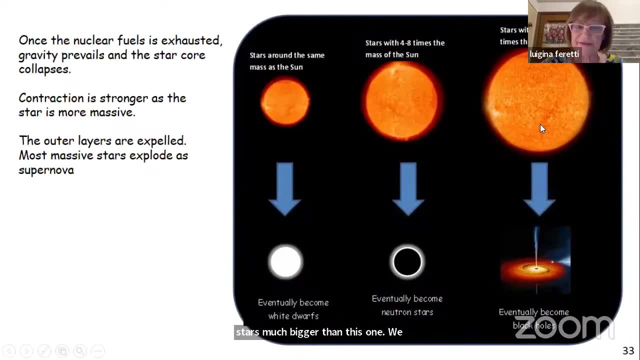 It will become a white dwarf. But stars much bigger than the Sun will have Such a big gravitation that will collapse and become black holes. Black holes are the extreme, Are the extreme status of matter, Is the more condensed matter possible It's. 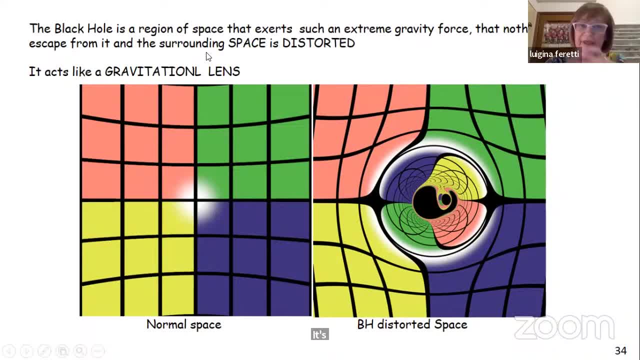 They are so, So condensed That they exert such an extreme gravity force That nothing can escape from the black hole, Not even the light. Indeed, we do not see the black holes Because even the light cannot escape. Not only, but the space around the black hole is distorted. 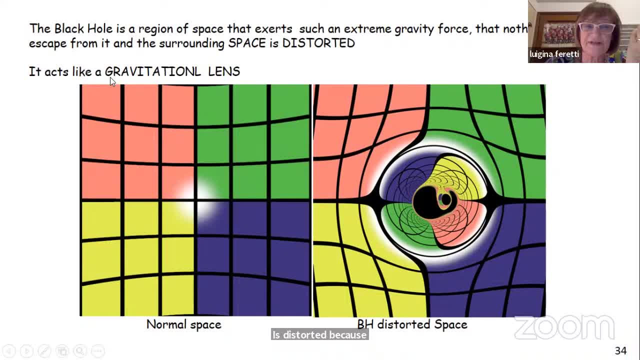 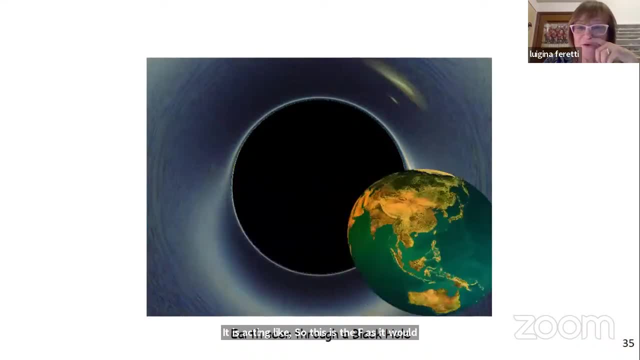 It's distorted because it acts like a gravitational lens. So gravity again is so strong, Then it acts. It is acting like a lens. So this is the Earth as it would be seen through the black hole. So completely, Completely distorted. 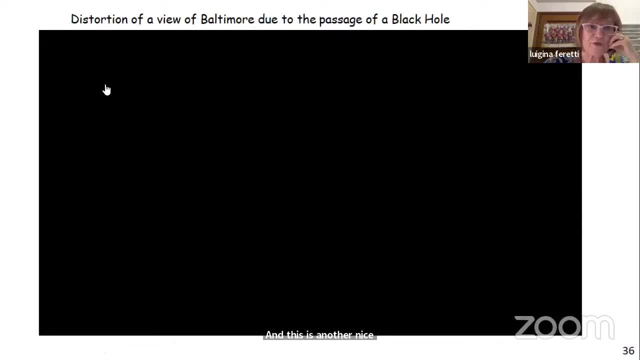 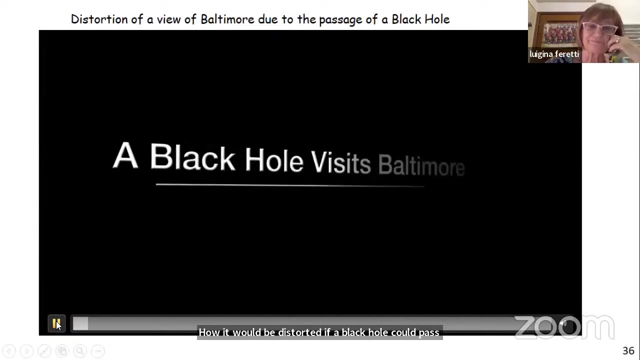 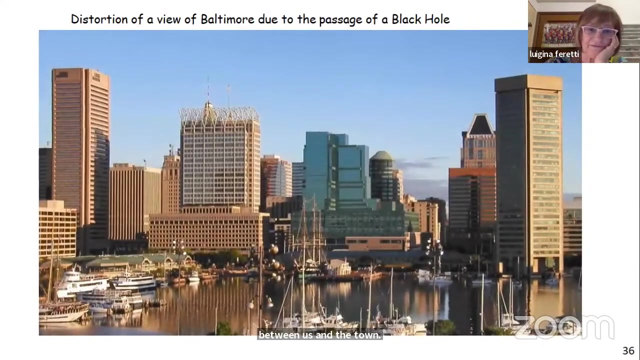 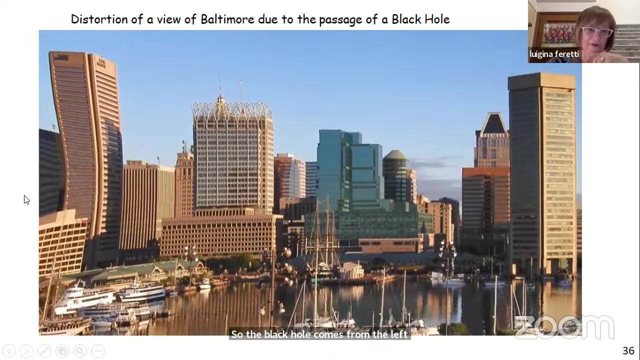 And this is another nice video showing a view of Baltimore, The town of Baltimore, How it would be distorted if a black hole Could pass between us and the town. So the black hole comes from the left And you do not see it. 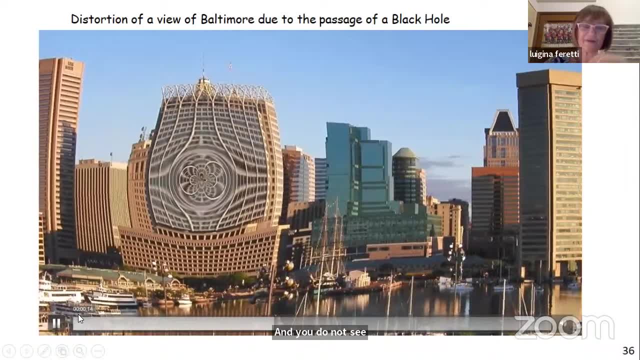 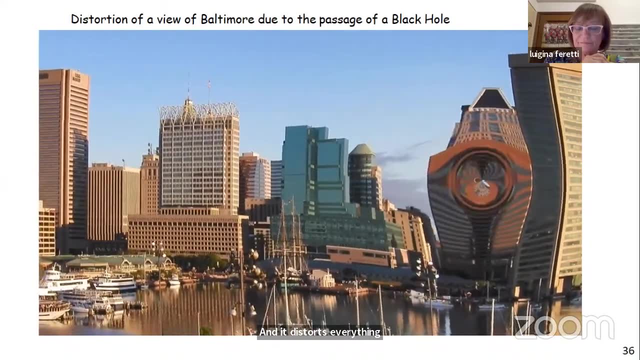 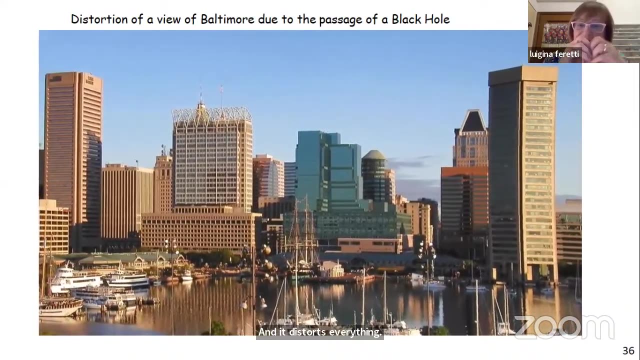 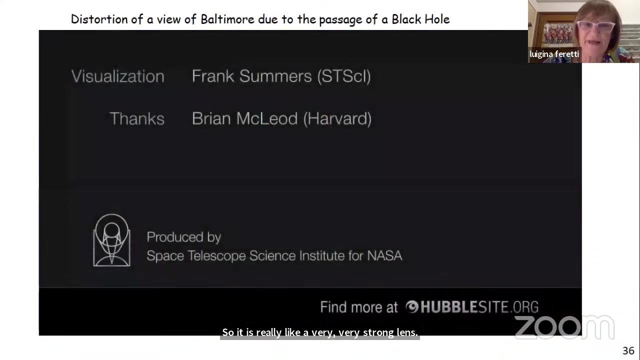 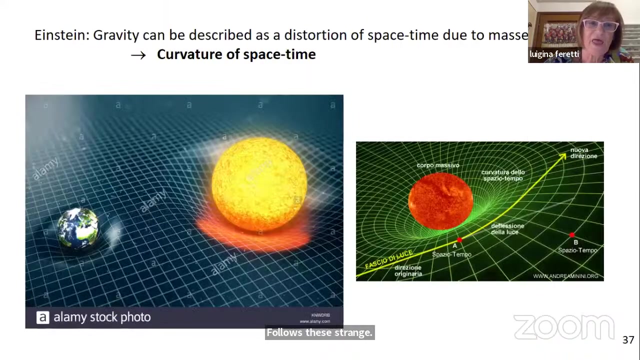 It's just a point And it distorts everything. So it is really like a very, very strong lens: Everything is distorted, What you see is distorted, The light follows this strange path And then, finally, we can arrive to the view of Einstein. 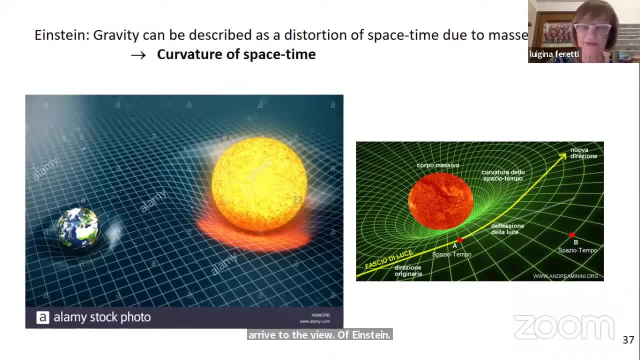 About, About, About the gravitation. The classical dynamics developed by Newton was revised by the theory of relativity of Einstein, Who said that gravity can be described as a distortion of space-time due to masses, Exactly how we have seen in the video before. 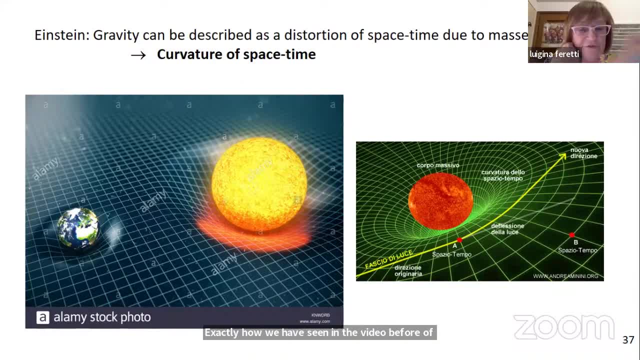 Of this black hole which is distorting the view of a town. Actually, the, The, The gravity, the masses distort the universe And the universe changes its geometry. So we are talking of a curvature, A curvature of space-time. This was the view of 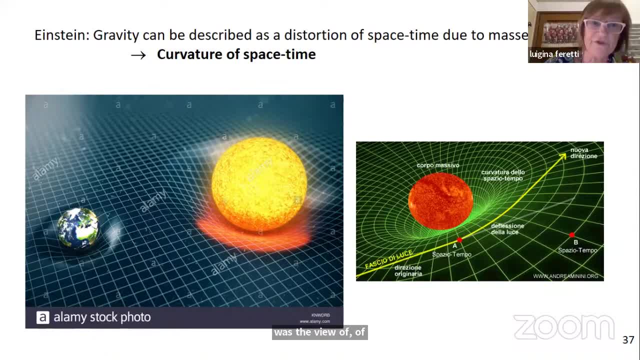 Of the modern, The modern vision of gravity. So the universe is similar to a soft carpet. Can be, Can be considered, I mean visualized as a carpet, Soft carpet. I think that in English you can say a trampoline. 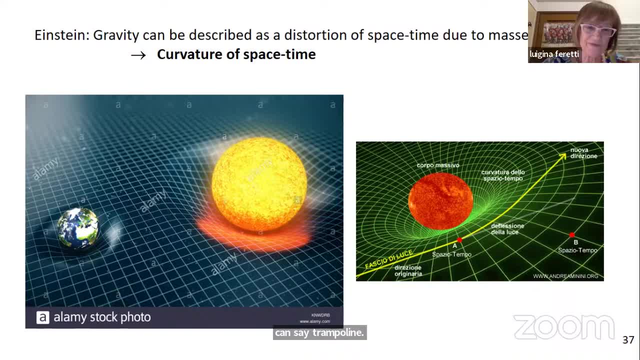 With elastic, Something which is elastic, And if this is the universe, which is elastic, which is a trampoline, The earth with its mass creates a distortion And this is the distortion that makes the moon rotating around it. The sun creates a distortion which is a bit larger. 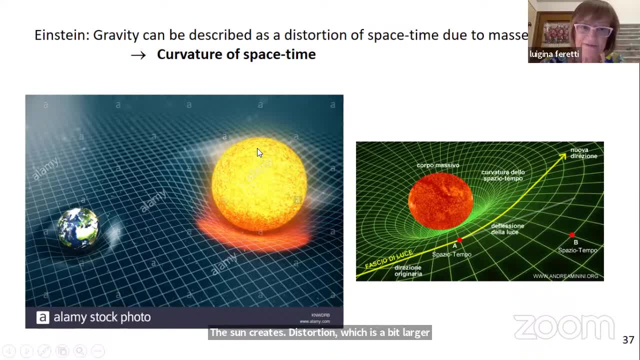 Because the sun is bigger than the earth And you see the distortion of this trampoline And all the objects rotating because of this geometry. And this is This image is in Italian, But the concept is the same: A massive object creates a distortion of the space-time. 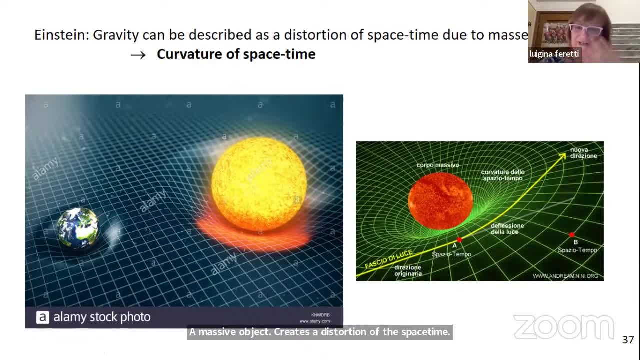 So the geometry of the universe is changing And you can see that also the light, which is the yellow line here, changes. its direction Is distorted by the curvature of the space-time. So Einstein equations are very, very complex And they are also presented in a compact form that is quite difficult to understand. 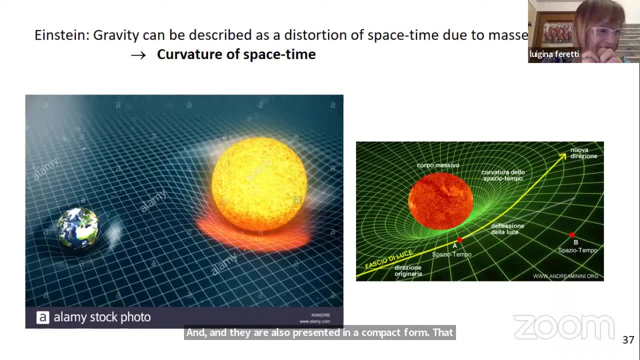 But we can say that Einstein equations tell us that the geometry of the universe depends on the masses, Which means that it depends on gravitation, And this is quite a new concept with respect to the classic physics And to the Newton theory of gravitation. 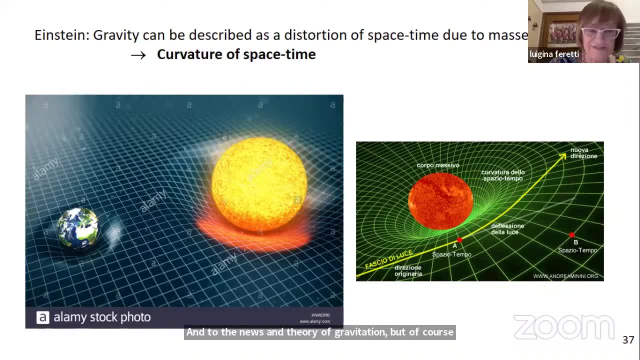 But of course, the law of Newton still applies. These are, I mean, this view is approaching the problem in a more complete way, Involving the space and the time, But, in conclusion, masses follow, the deformation of the space-time producer. 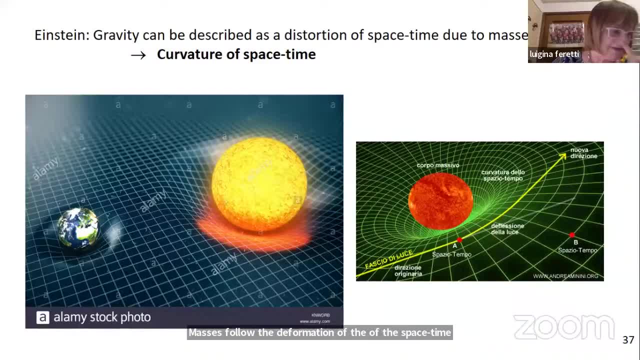 Produced by the big masses. The matter tells to the space-time how to deform And the space-time tells the matter how to move. And this is the view of Einstein of gravity, which is quite complex, But it is just to give an idea that. 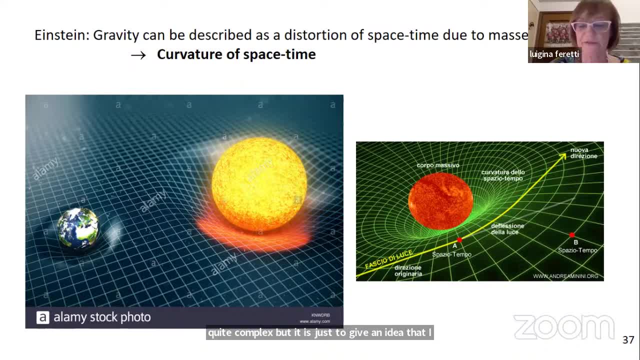 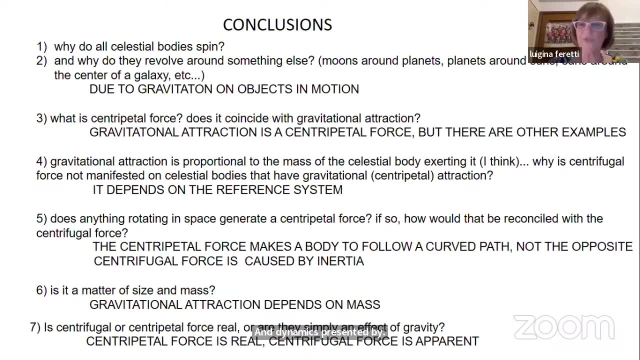 I mean there are more modern concepts with respect to the classical dynamics Presented by Newton. So I think that I come to the conclusion. I put in my conclusions the questions that were presented to me at the time of When we decided to do this webinar. 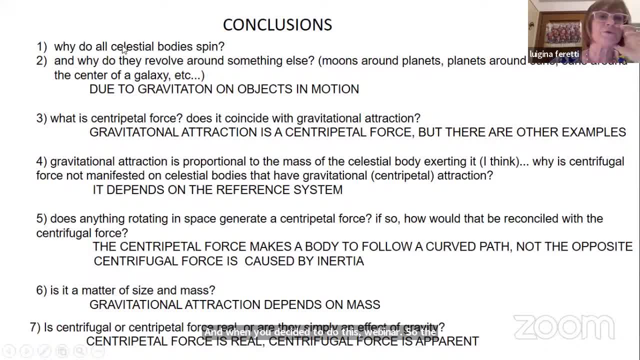 So the question is: why do? The first question was: why do all celestial bodies spin And why do they revolve around something else? Moons around planets, Planets around suns, Blah, blah, blah, And the answer is now very clear and simple, I think. 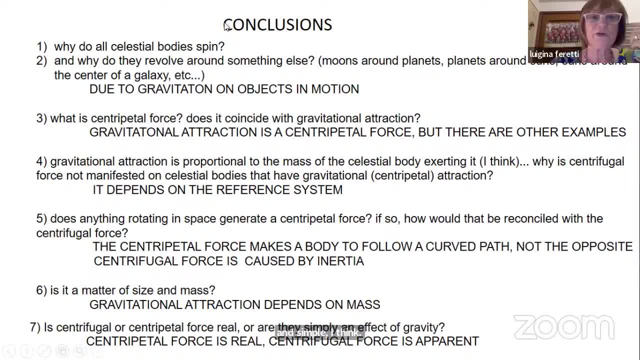 I hope that it was clear. It is due to gravitation on objects in motion. Big bang has given motion to the objects And the gravitation has done the rest. What is the centripetal force? Does it coincide with gravitational attraction? 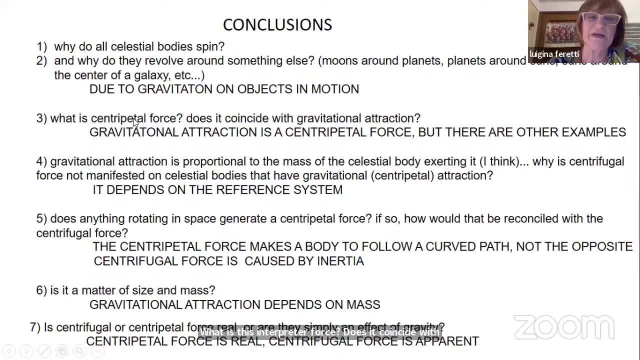 Actually it is the opposite. Gravitational attraction is a centripetal force, But there are other kinds, Other examples of centripetal forces, Like the carousel, The stone, The car Which is going in a circle, and so on. 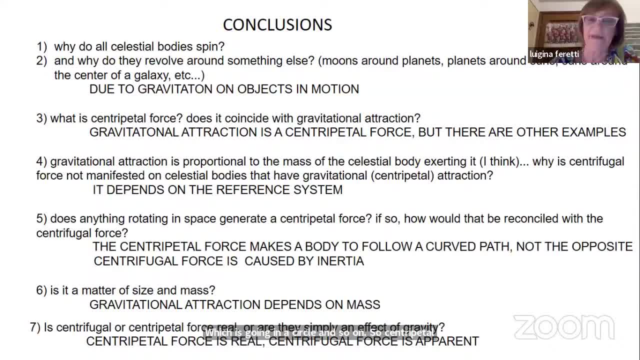 So centripetal force is something that is described by the dynamics of Newton. Another question: Gravitational attraction is proportional to the mass of the celestial body. Why is centripetal force manifested on celestial bodies that have gravitational attraction? Actually, I hope that also this was clear. 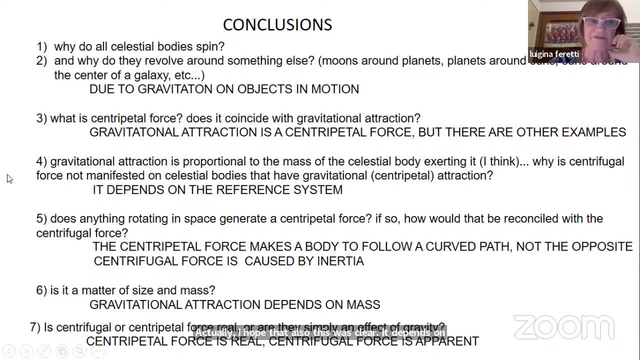 It depends on the reference system. Centripetal force is an apparent force. Actually, what is manifested is the tendency of the bodies to go in a straight line If there was no force. If there is force, they do not go straight. 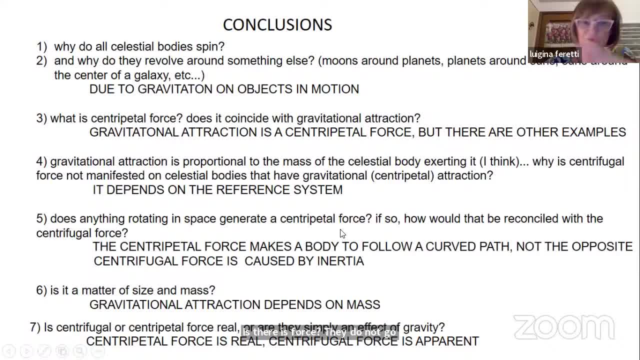 And you feel the centrifugal effect. Does anything rotating in space generate the centripetal force? So again, we are saying very similar things. So we say that as an answer: the centripetal force makes a body to follow a curved path. 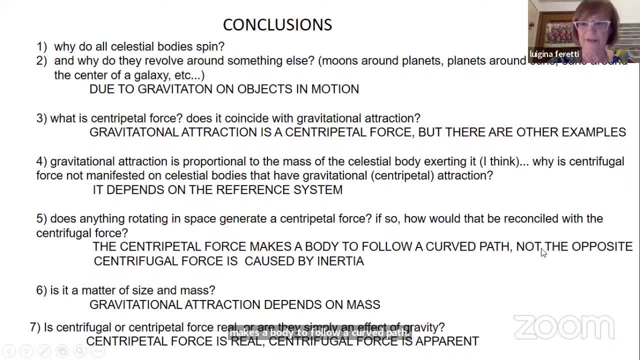 And Not the opposite. So it's not the rotating body that generates a centripetal force, But it's the centripetal force that makes a body to follow a curved path, And centrifugal force is caused just by the inertia When you feel you against the chair of the car on a turn. 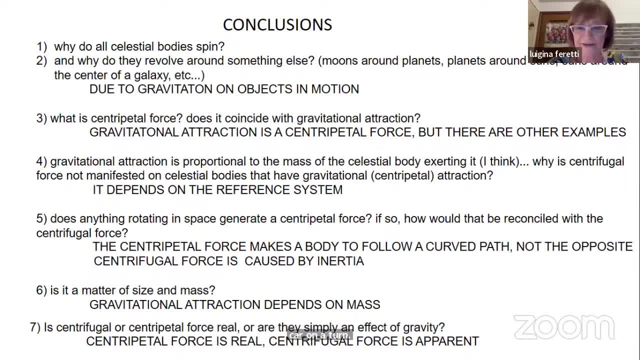 This is because your body tends to go straight, But instead the centripetal force makes you change the direction. What is it a matter of size and mass? Yes, of course, Gravitational attraction depends on mass. Is centrifugal or centripetal force real? 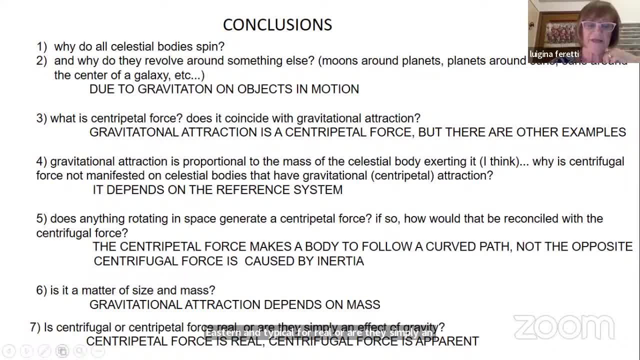 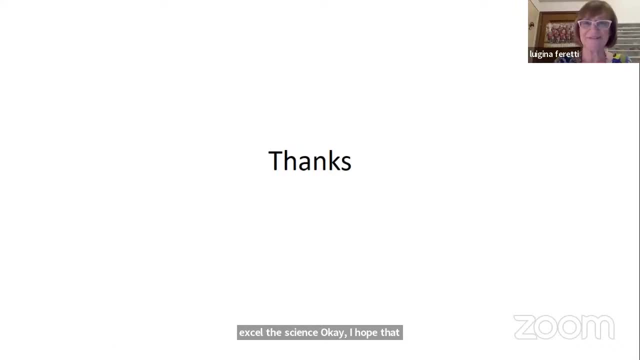 Or are they simply an effect of gravity? So centripetal force is real. Centrifugal force is apparent. It's a pseudo-science, Pseudo-force. Okay, I hope that something will remain. I hope that it was not too difficult. 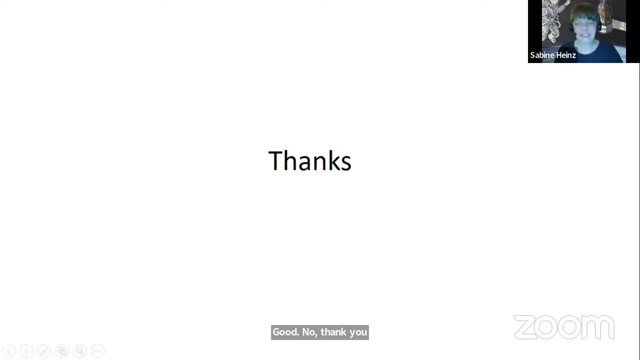 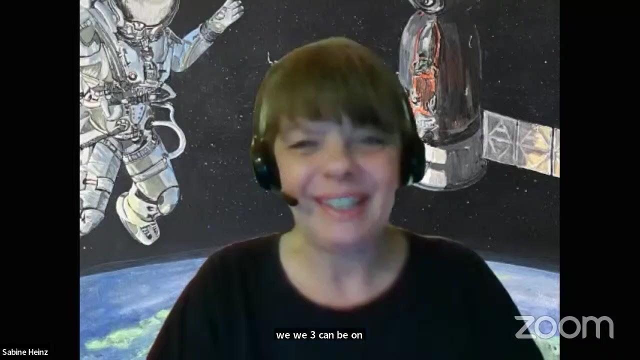 No, thank you so much. It was a really, really interesting lecture and well explained And I'm really glad that. Could you please stop sharing the screen so we three can be on the Yes And Yes. Thank you so much. 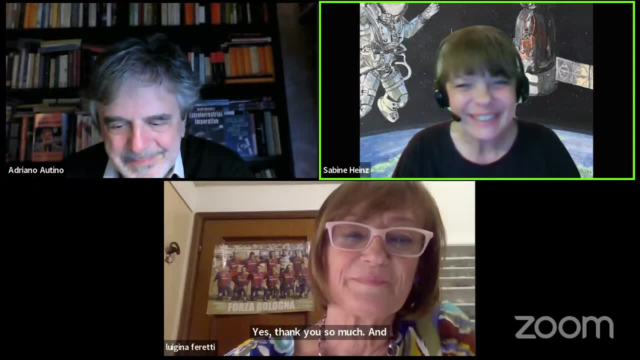 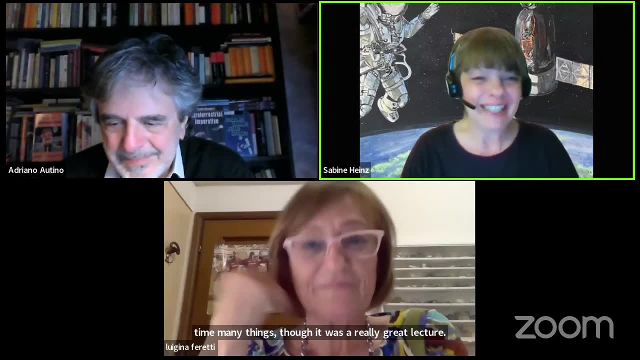 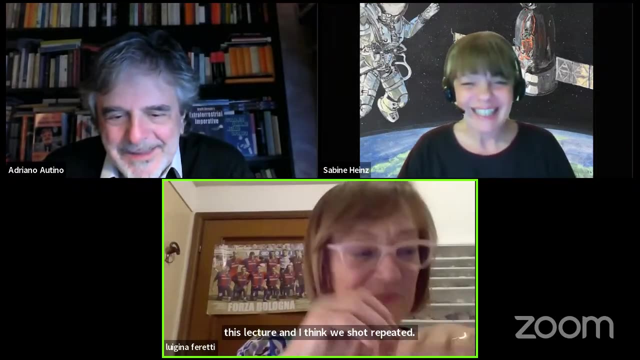 And I really understood the first time many things, So it was a really great lecture. Yeah, It was a good idea from you, Adriano, to initiate this lecture, And I think we should repeat it. I mean, they are not easy concepts. 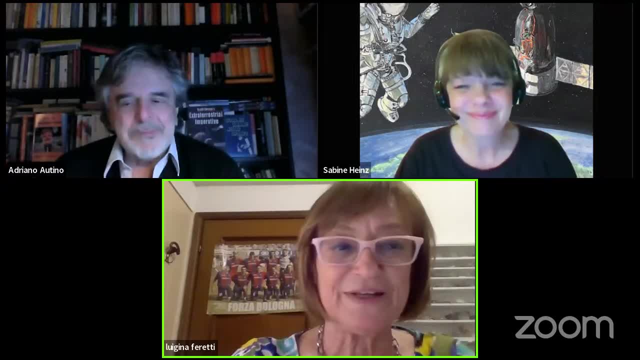 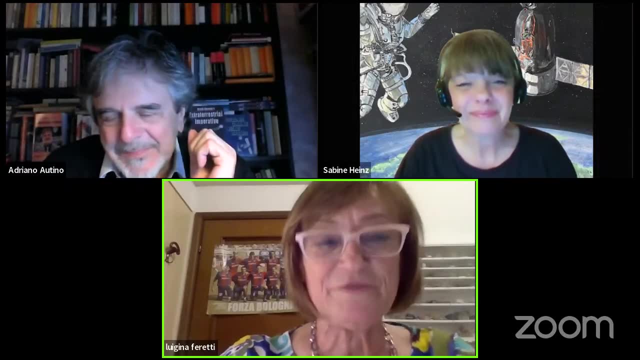 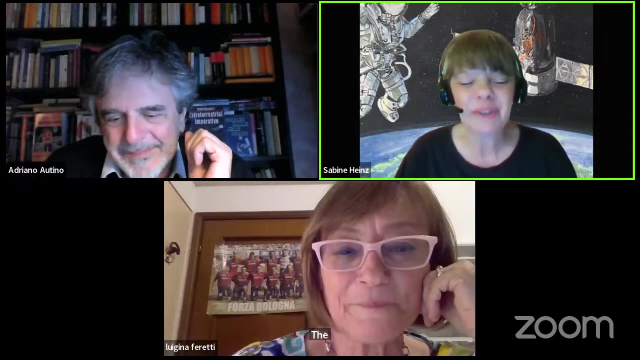 And so If there is something not clear, it is. I mean, it is reasonable, Especially the centrifugal force. I talked to a student who is studying engineering. Yes, But it was interesting And I could understand. you made it really clear. 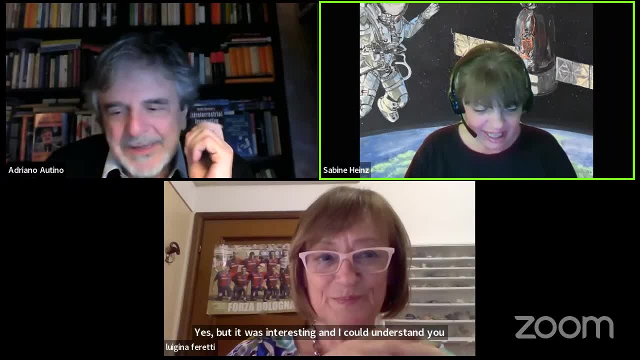 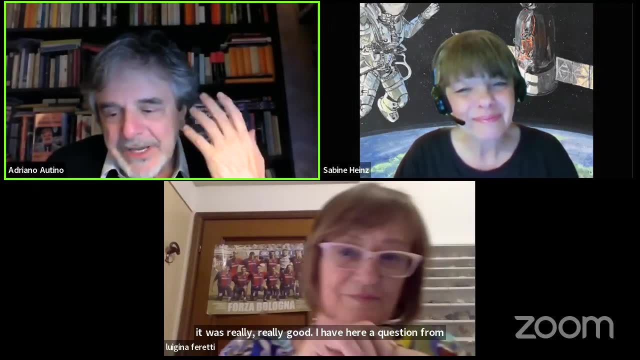 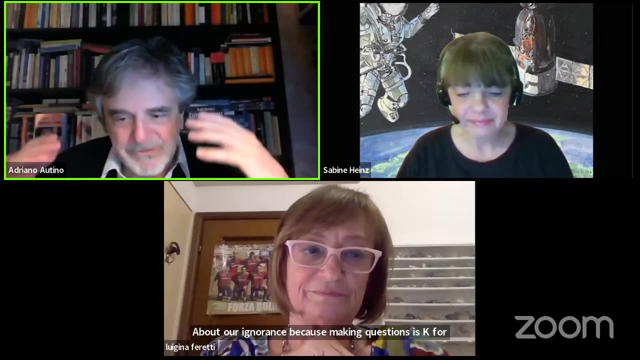 So it was really, really good. I have here a question from: It's always better, let me say it is always better, not to feel shame about our ignorance, Because making questions is key for anything that we want to do. We have to make questions. 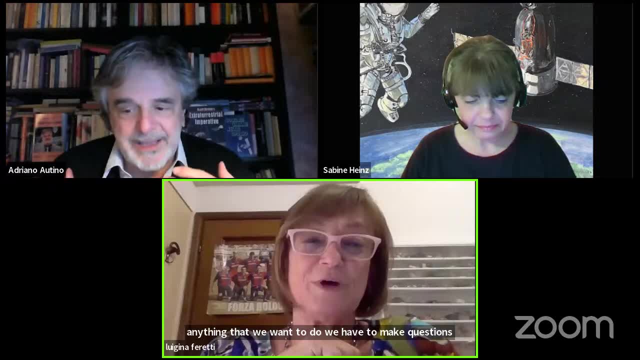 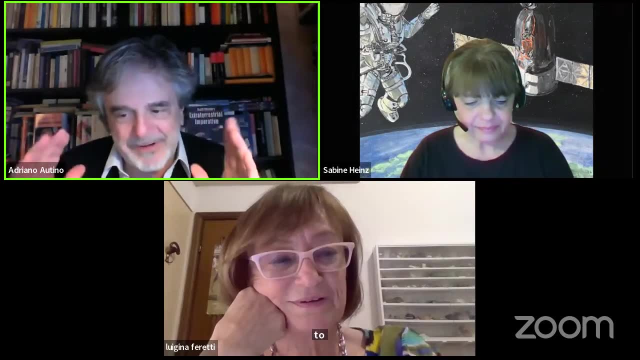 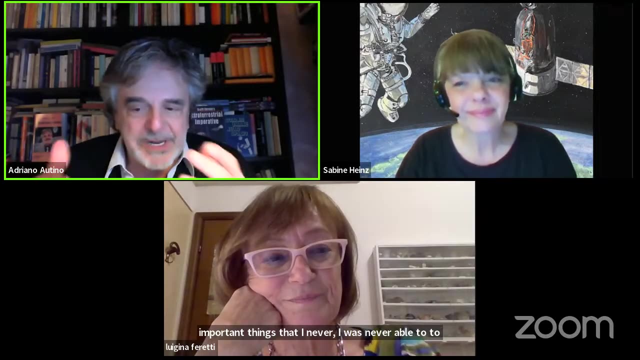 We have to make questions, And Yeah, It's what Umberto Eco said: I have to. Yes, I have to confess that today I learned a couple of very important things that I never I was never able to get before, Because today it was explained in a clear way. 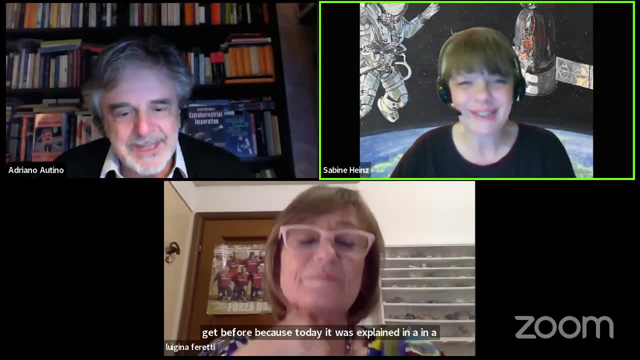 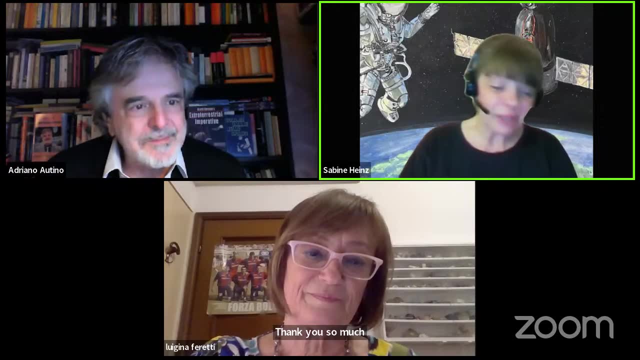 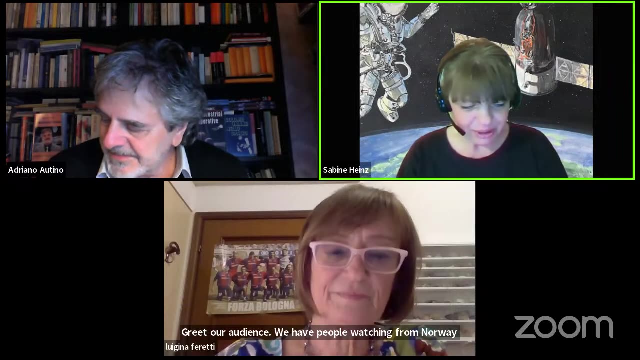 And it's easy to understand. Excellent, I have to agree with Adriana. I'm glad. I'm glad, Yes, Yes, I have here a question from. I would like to greet our audience. We have people watching from Norway, from Spain, from Germany. 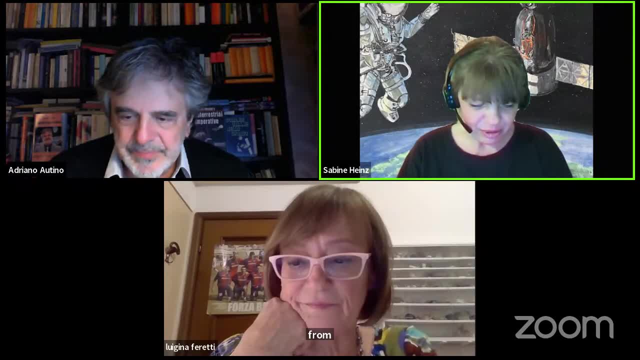 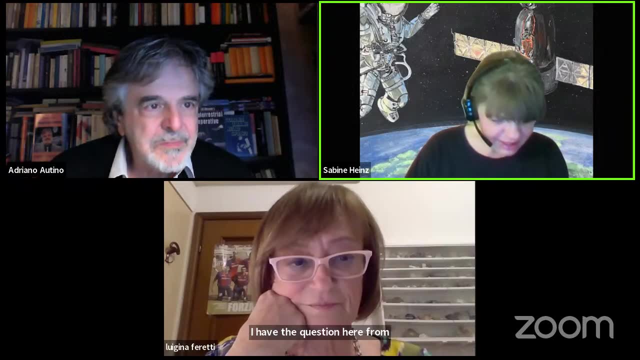 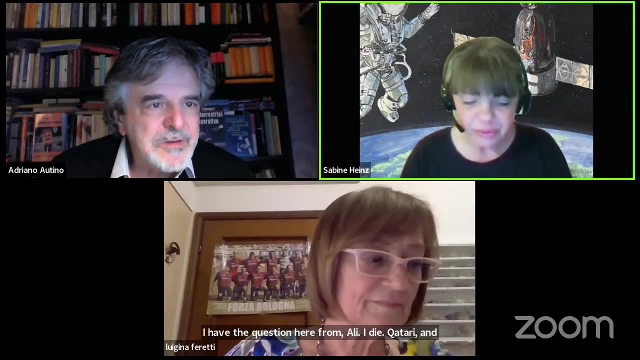 Yeah, From different countries, From France. And I have a question here from Alai Alai Jai Kotari And he's asking: what are the chances? What are the chances that the last pole reversal was responsible for the Holocene period? now, 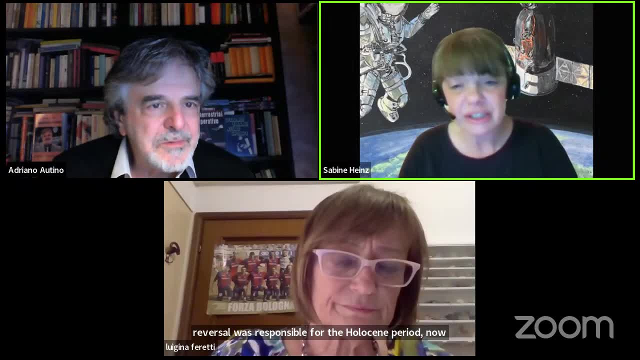 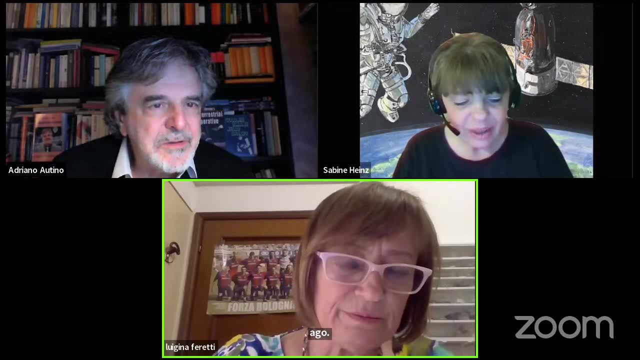 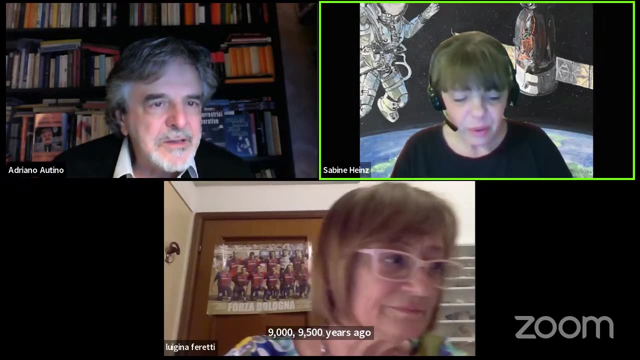 which also began about 9,500 years ago- 900.. When was it 9,500 years ago? Can you say again what happened? Yes, So what are the chances that the last pole reversal was responsible for the Holocene? 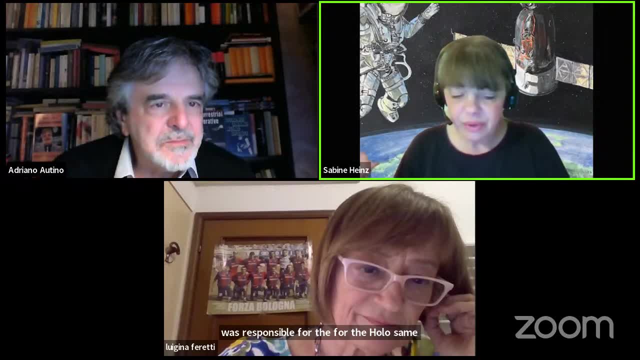 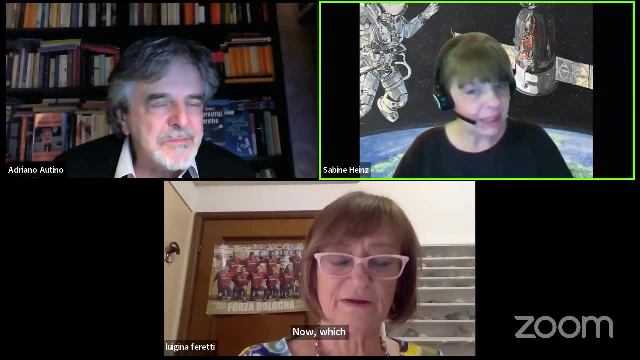 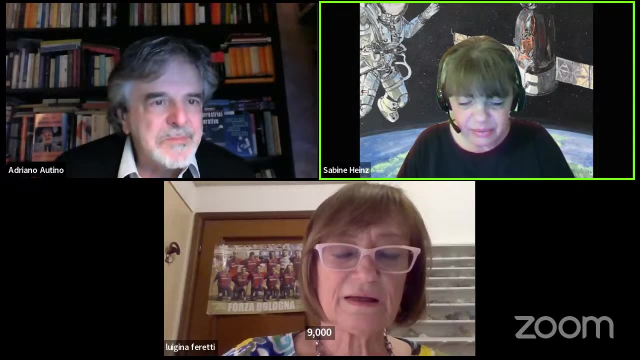 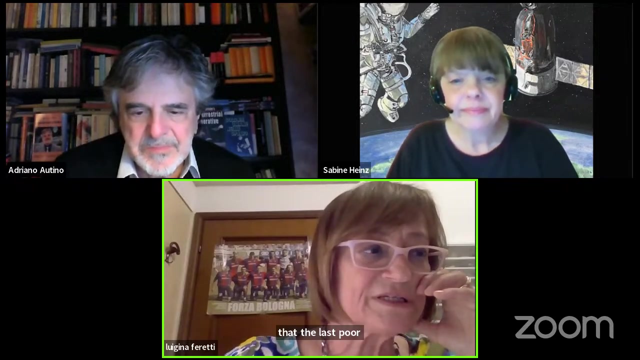 for the Holocene period now, which also began about 9,500 years ago. as the Holocene period began, Holocene 9,500.. Yeah, And what are the chances that the last pole reversal was responsible for this? Actually, the last reversal was 780,000 years ago. 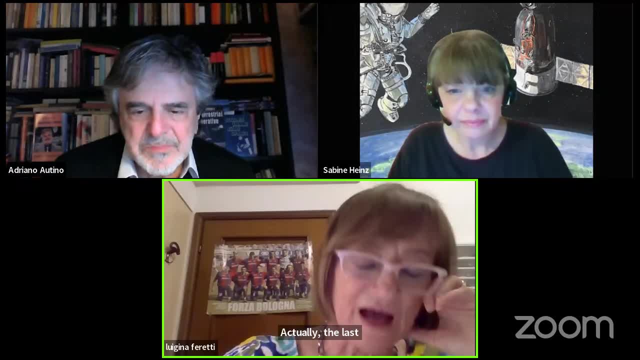 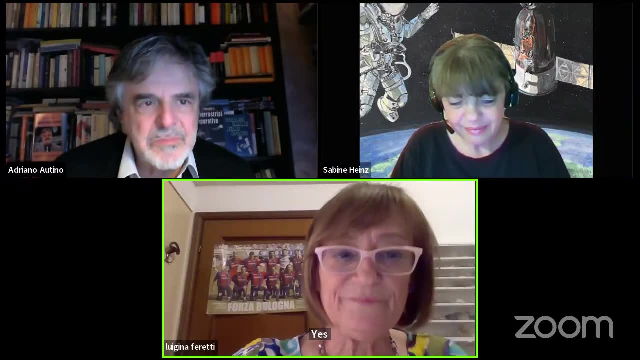 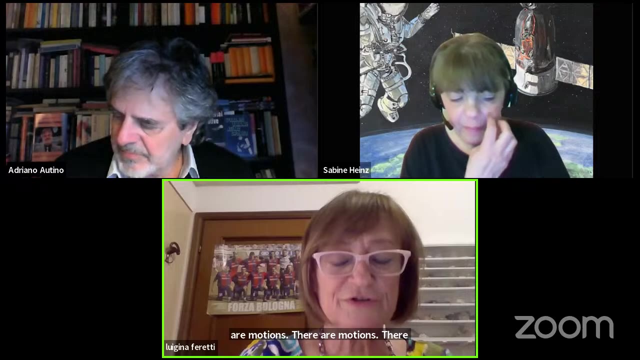 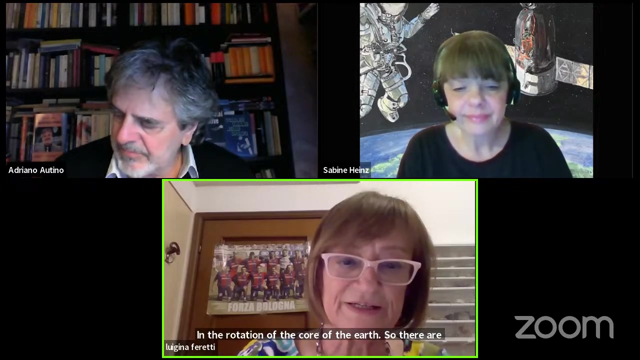 Yes, Yes, Yes, Yes. So it has more, So much, much, much, much more distance. Certainly there are motions. There are motions, There are changes in the rotation of the core of the Earth, So there are changes in the direction of the magnetic field. 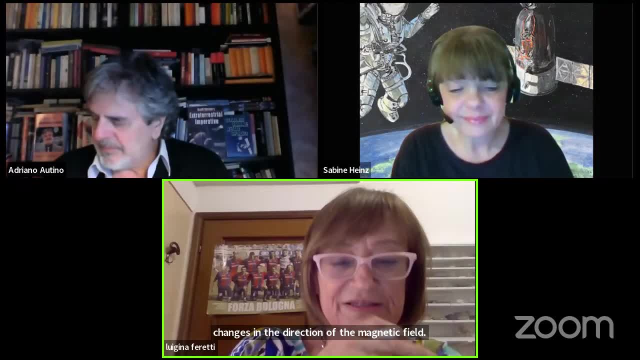 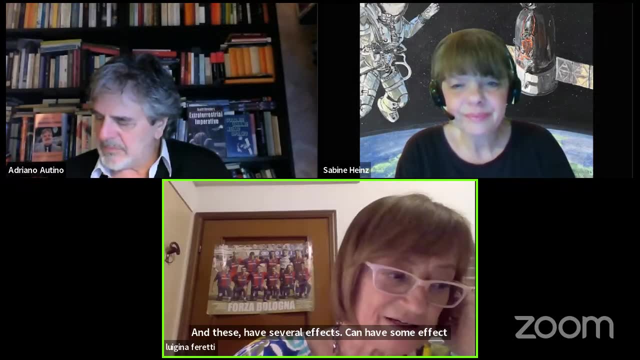 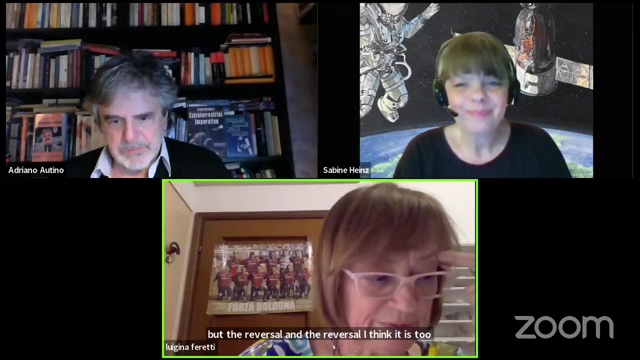 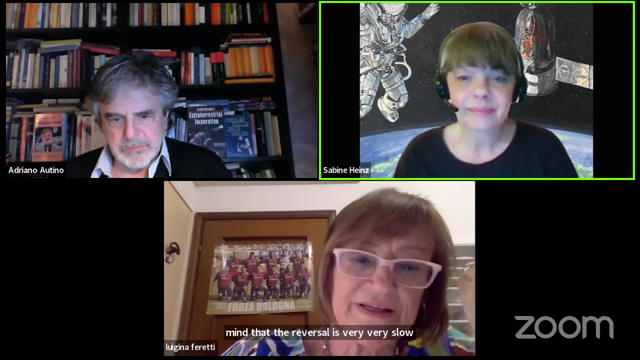 And these can have several effects, Can have some effects, But the reversal, I think it is too long ago And also keep in mind- we have to keep in mind that the reversal is very, very slow. Yes, It takes about 10,000 years to develop. 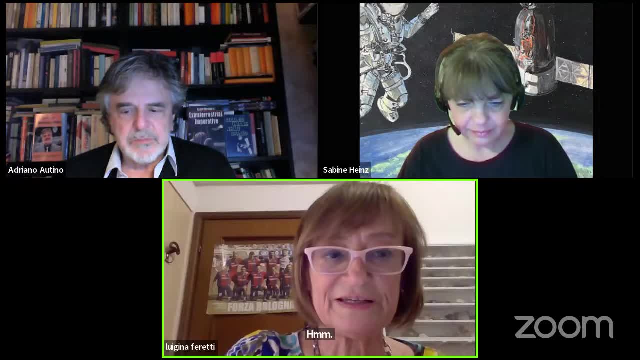 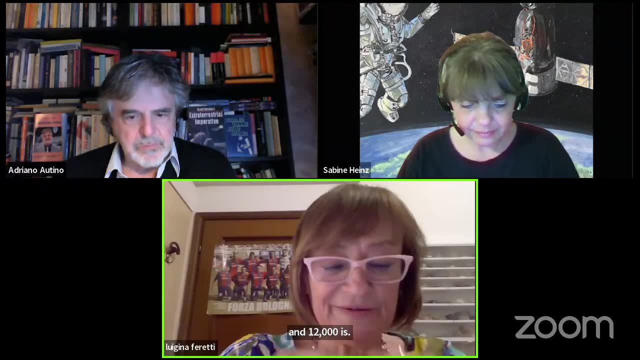 And it is. I mean, there is a big uncertainty. It's an uncertainty between 2,000 years and 2,000 years, Yes, Between 2,000 years and 12,000 years, But not less than 2,000 years and probably around 10,000. 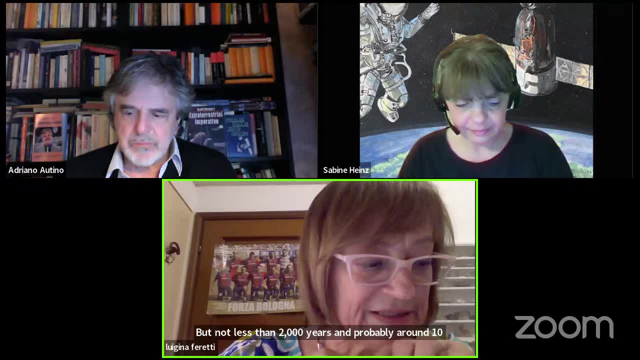 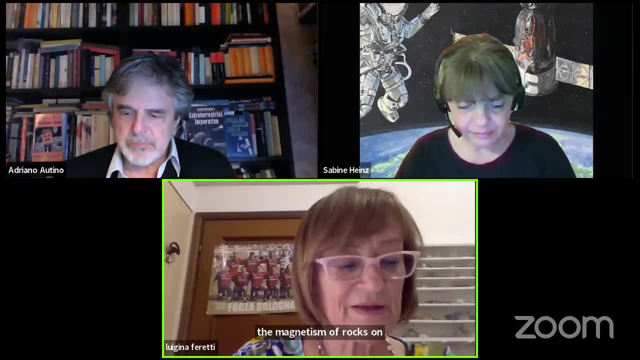 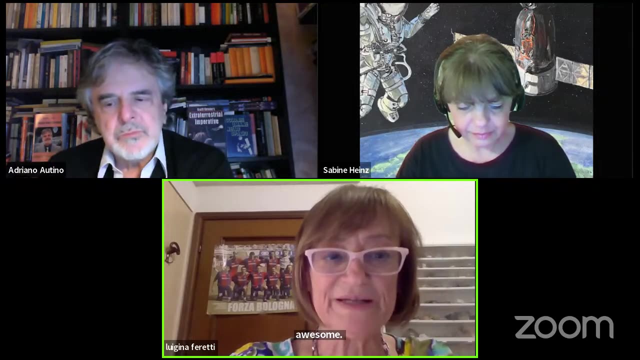 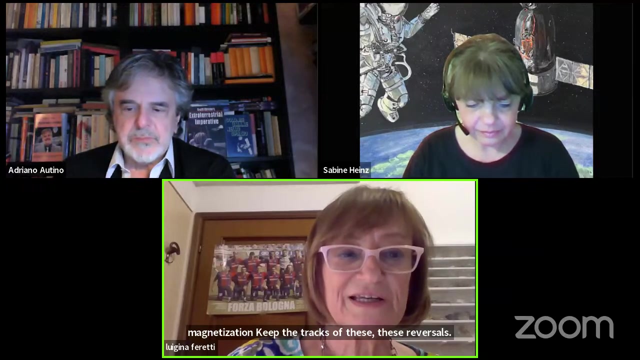 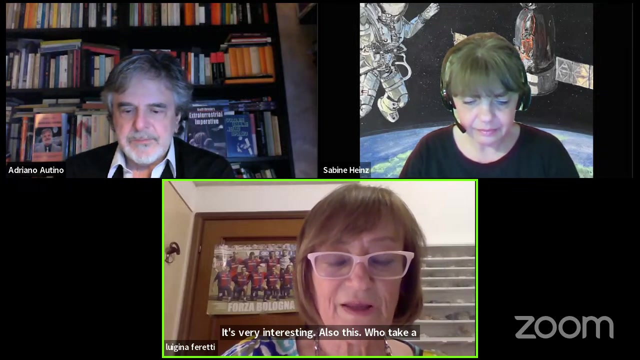 They make these measurements by measuring the magnetism of rocks on the bottom of the oceans. These rocks keep magnetized And they find that the magnetization keep the tracks of this reversal. It's very interesting. Also, this could take a complete seminar. 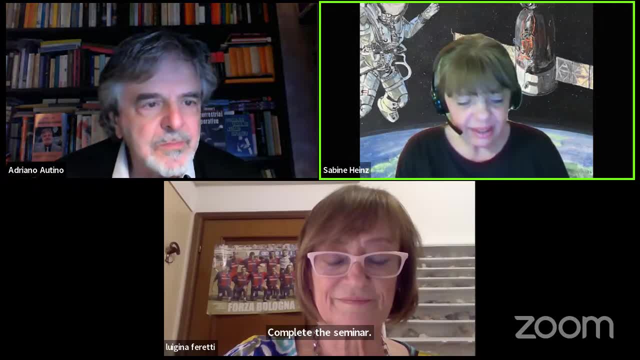 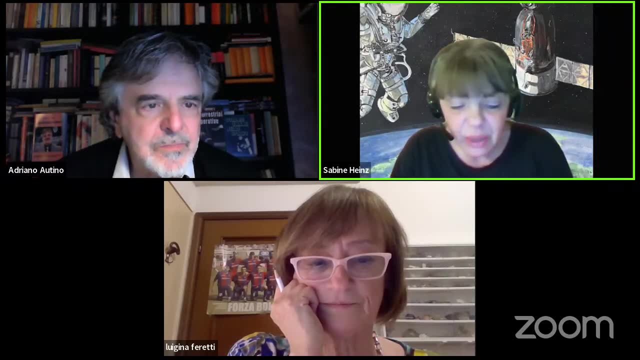 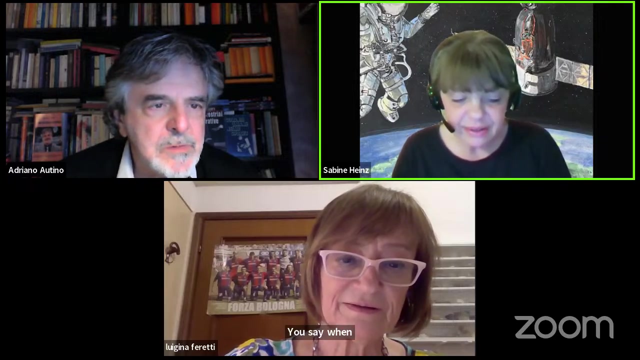 Thank you. Here's another question: When it goes to form into a mass singularity? so a black hole? Yes, You say when, When, When it goes? No, I don't think that Betelgeuse will go into a black hole. 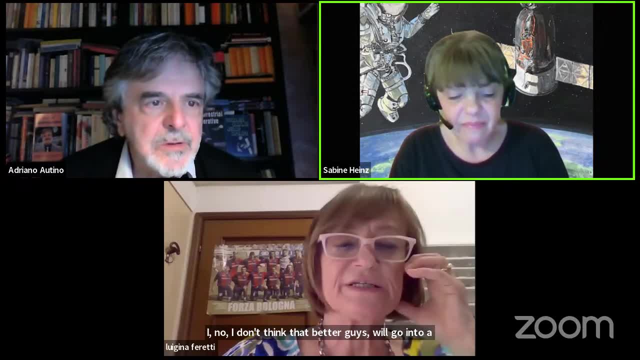 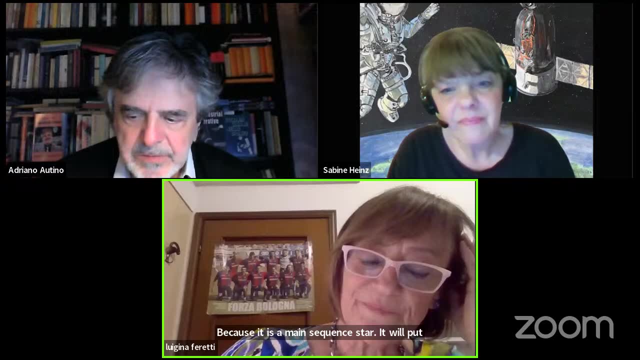 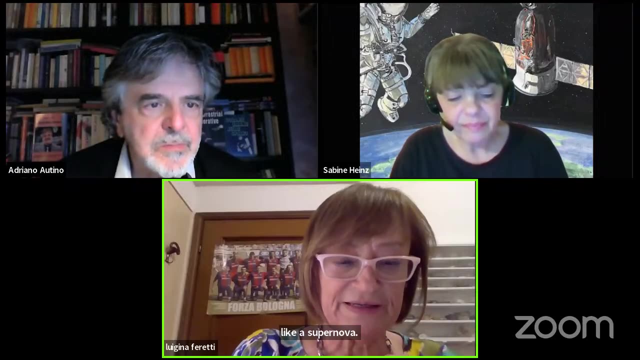 Aha, Because it is a main sequence star. It will probably- Well, I'm not sure, But I think it will explode like a supernova And then leave a neutron star, Neutron star, at the center. He means supernova. 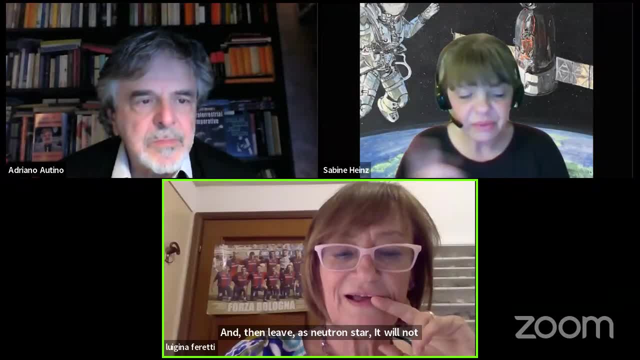 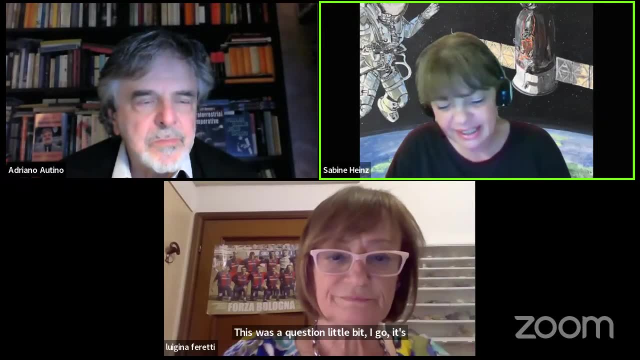 It will not become a black hole- Aha, This was a question with Betelgeuse- When it goes supernova to form into a mass singularity. Yeah, I didn't know what SN means. So Yeah, Yeah, Yeah. Okay, It will become a supernova When We don't know It is. It is very bright, It has shown variations in the brightness, And so we expect that it will happen, not in billion years, Not in a million years. 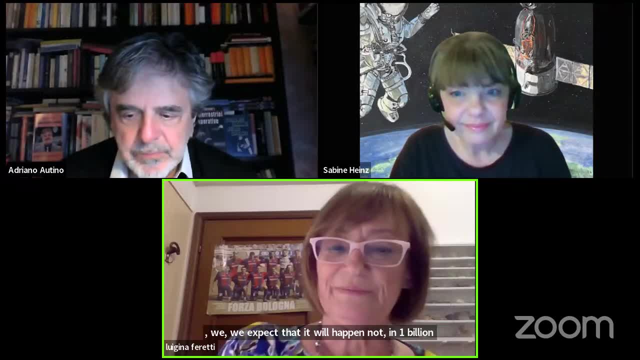 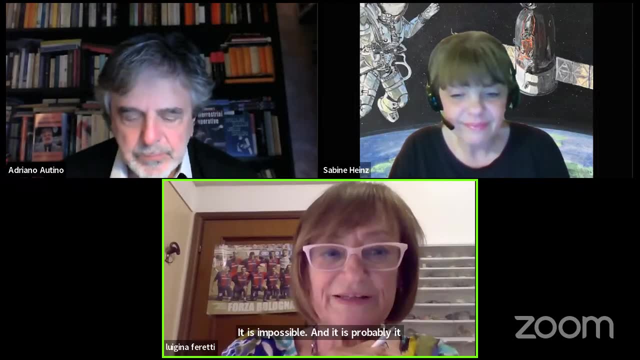 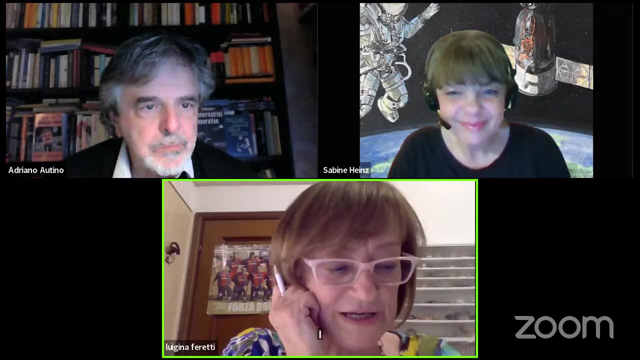 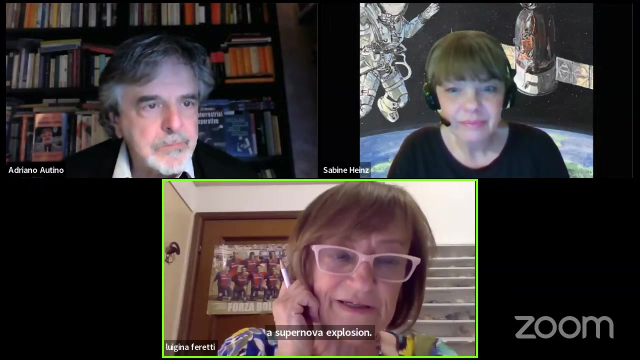 But it is really difficult to know It is In practice. it is impossible. It is Probably. it is the next one And we will see it. It will be very spectacular. I remember you that there was a supernova explosion in 1054 year. 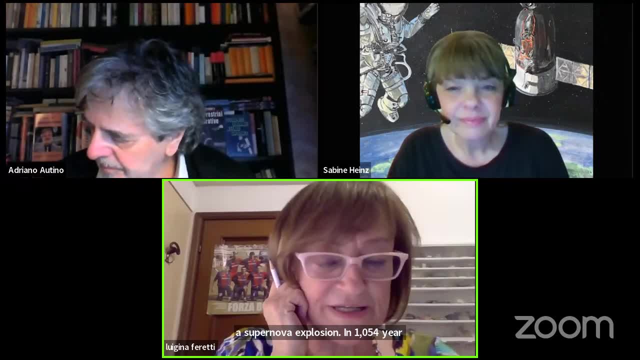 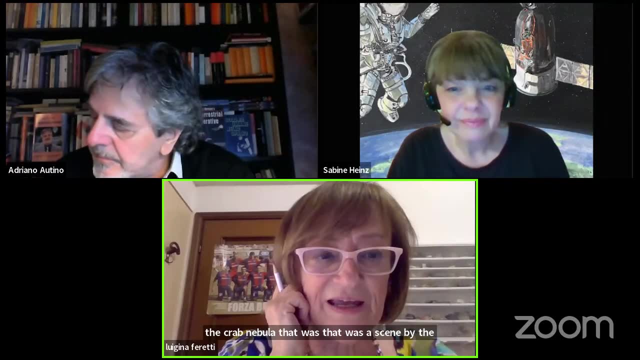 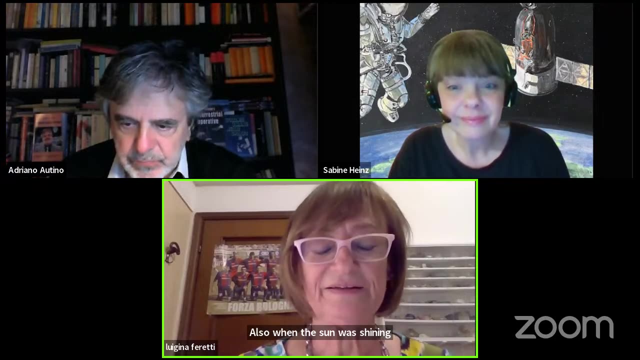 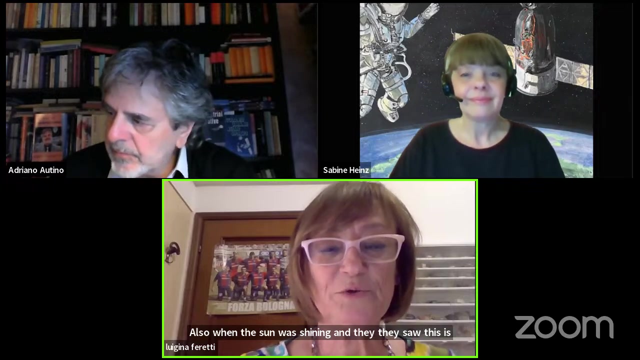 1054. Which is the Crab Nebula. That was That was seen by the Chinese And during Also during the day, Also when the sun was shining, And they, They saw this supernova for several days And it was shining. 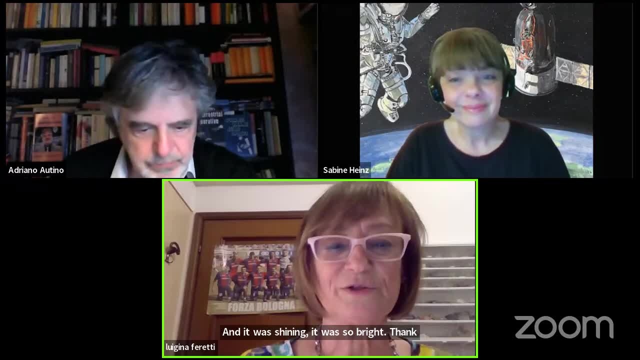 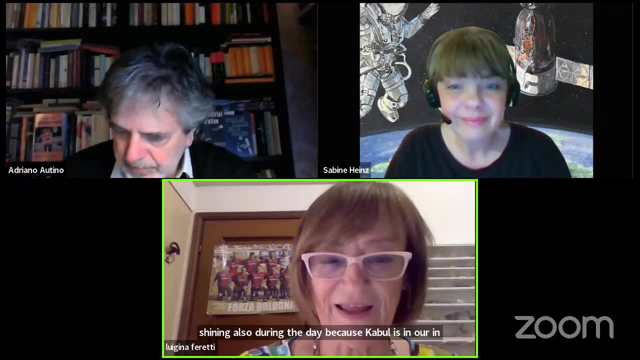 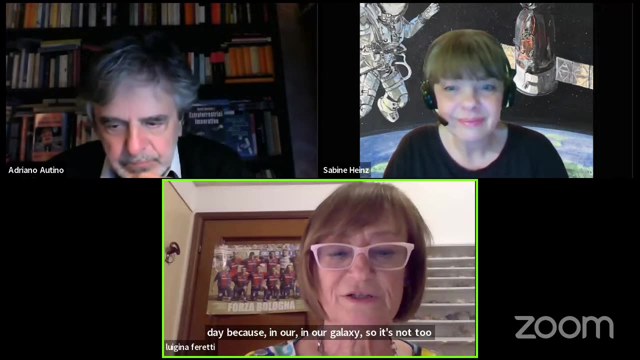 It was so bright that it was shining also during the day, Because Crab Nebula is in our, In our galaxy, So it's not too distant in the terms of cosmic distances. And also Betelgeuse: Betelgeuse is not too distant. 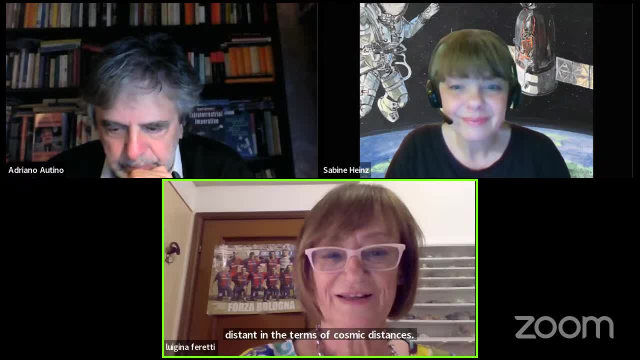 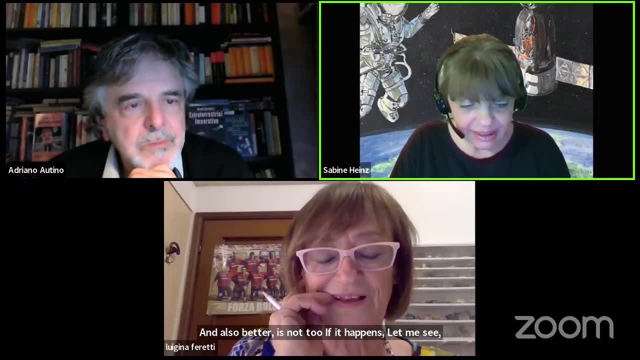 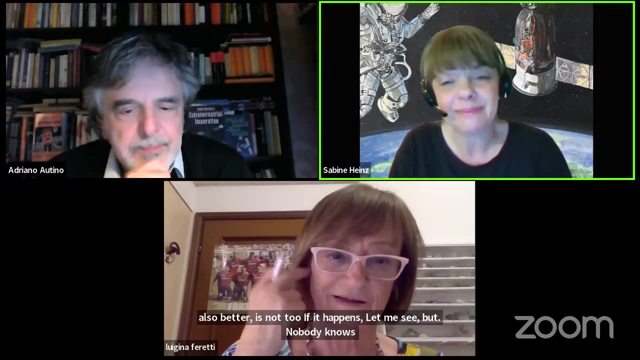 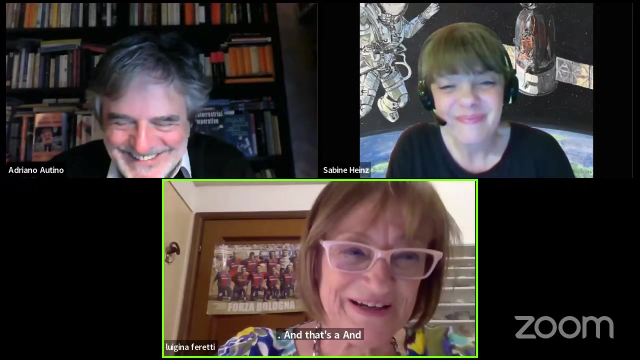 So we, If it happens, we will see, But nobody knows. Okay, And here's another question: Will humanity ever be able to actually know what was before the Big Bang? No, That's a very difficult question, But it is what we would like to know. 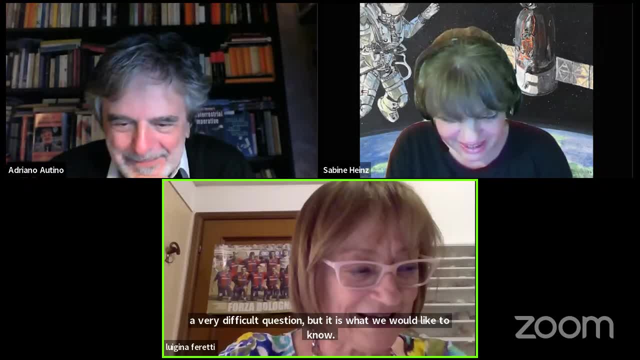 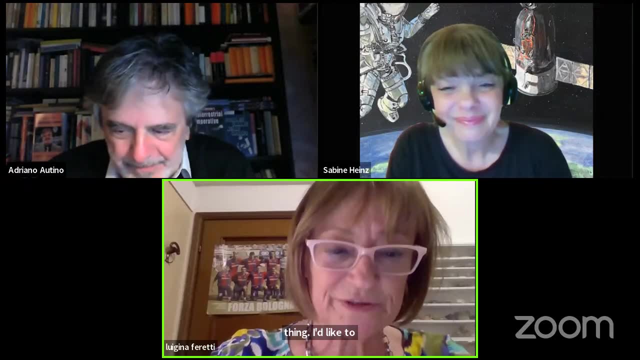 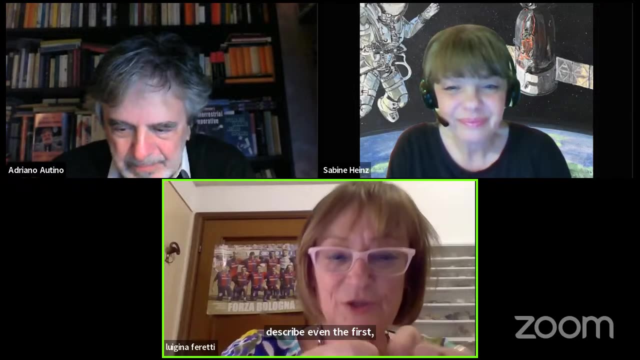 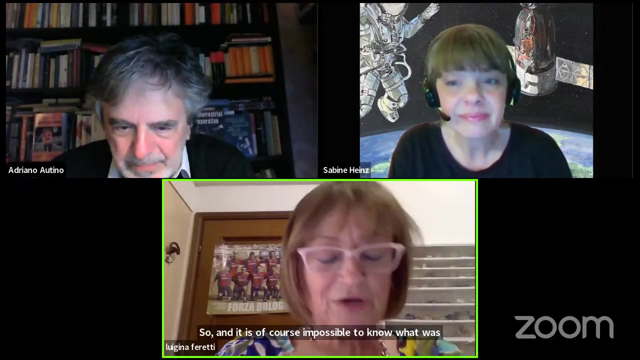 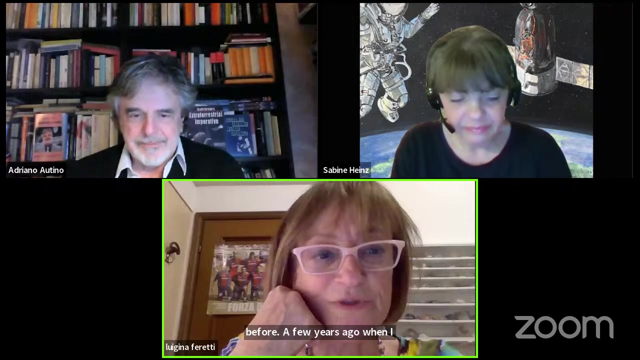 Everyone wants to know. Actually, just as a first thing, I'd like to say that physics is not able to describe even the first seconds of the Big Bang, So it is, of course, impossible to know what was before, But a few years ago, when I was at the beginning of my astrophysical career, there was a model of the universe that I liked a lot, which was the cycling universe. 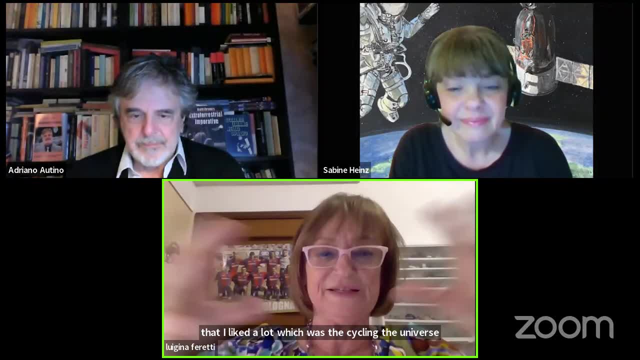 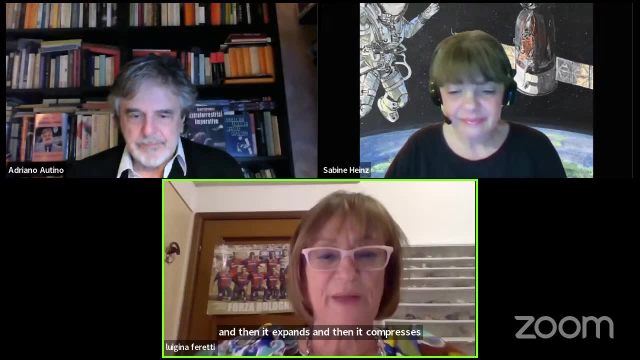 So universe that expands and then it compresses again, and then it expands and then it compresses So many cycles of this universe that expand and compresses. So you understand what before the Big Bang, Before the Big Bang, there was another universe that recompressed and then it exploded again. 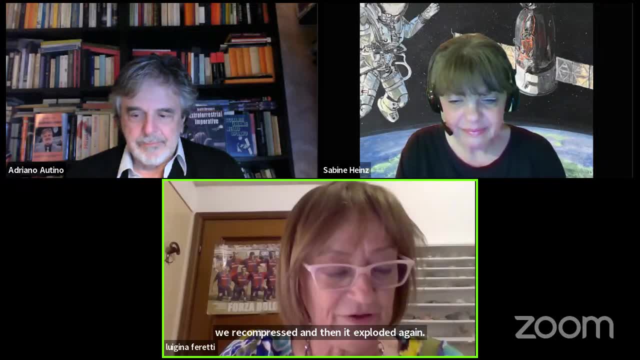 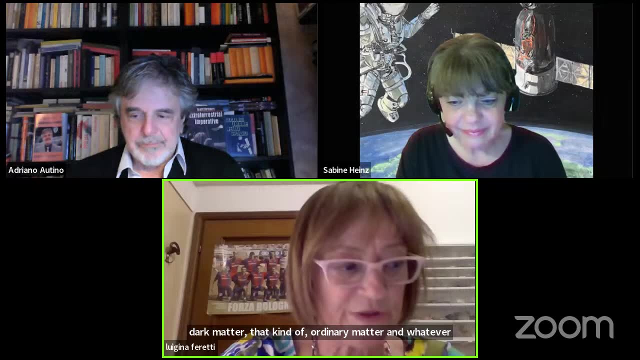 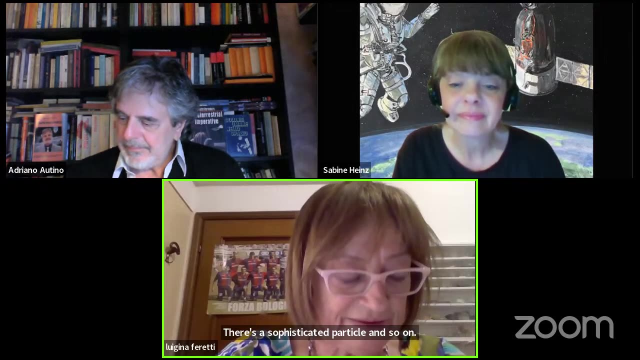 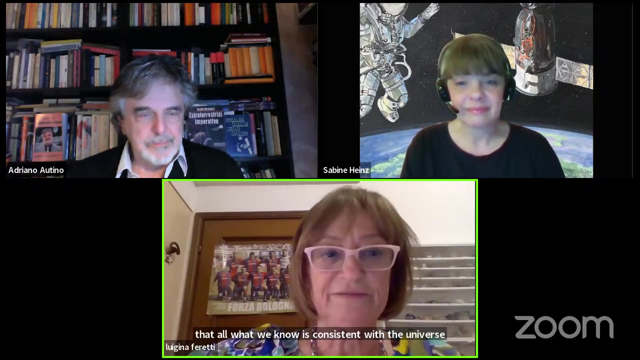 Now, with the knowledge that we have of the dark matter- dark energy, ordinary matter and whatever- and many more sophisticated particles and so on, we think that all what we know is consistent with the universe Going, expanding forever, Expanding forever, forever, forever. 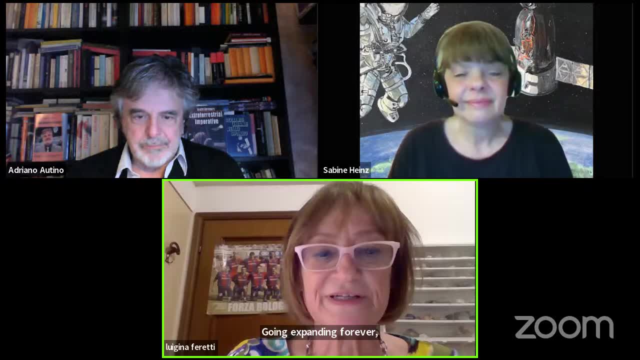 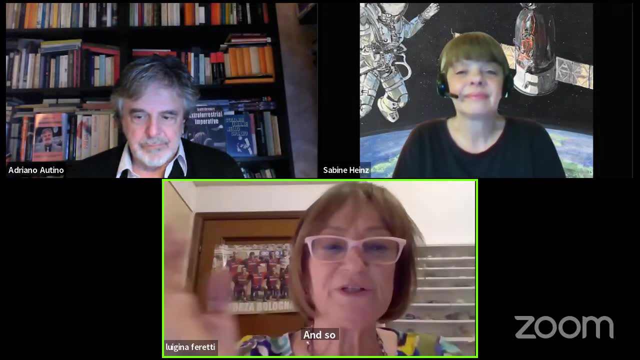 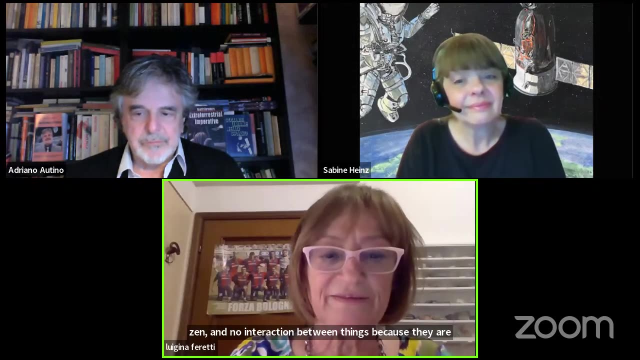 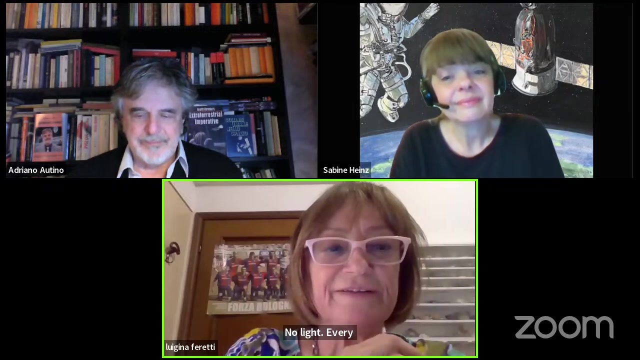 For other 20 billion years, And so becoming the so-called big freeze: All frozen And no interaction between things because they are too distant to interact. No light, Everything will turn off. So this is what. Yeah, This is the current theory. 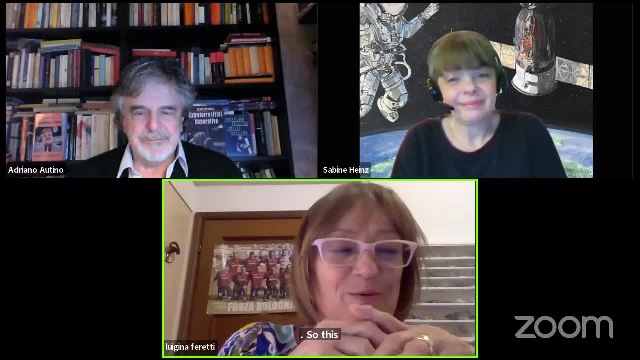 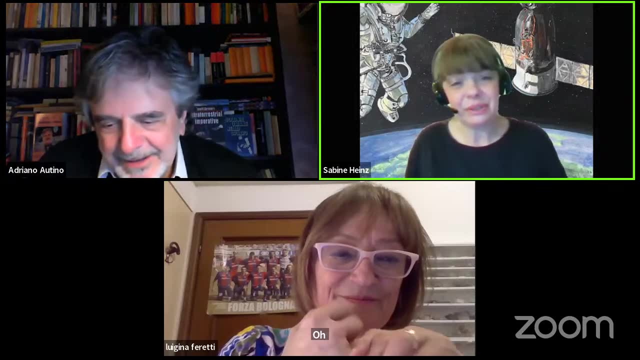 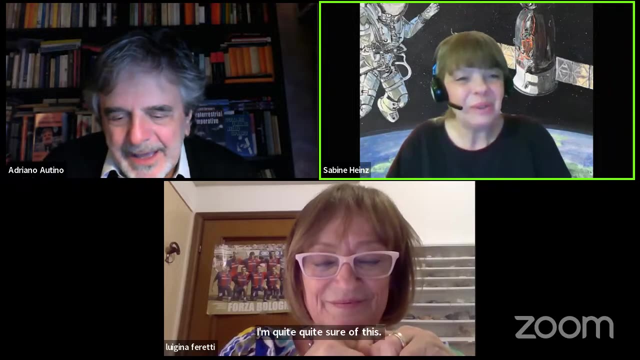 So to know what was before the Big Bang is really impossible. And who knows this? The person who will find it out will get the Nobel Prize. I'm quite sure of this. Adriano, do you have one question? One more question. 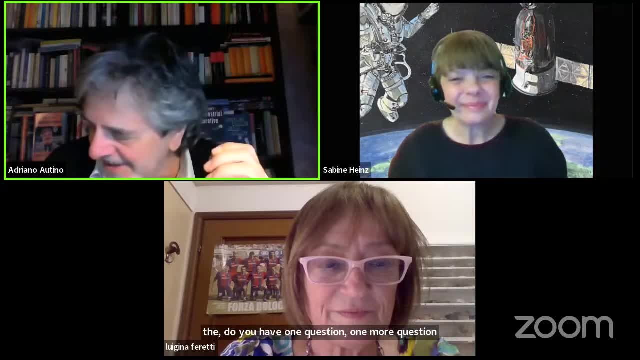 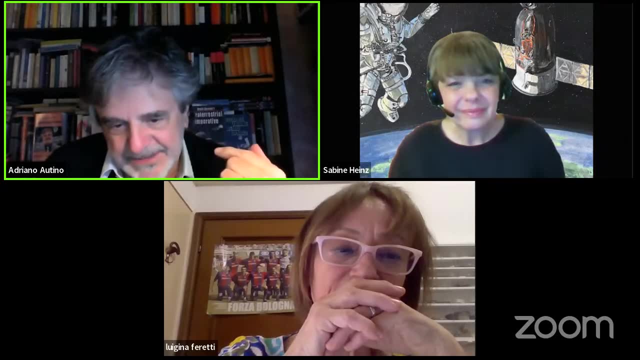 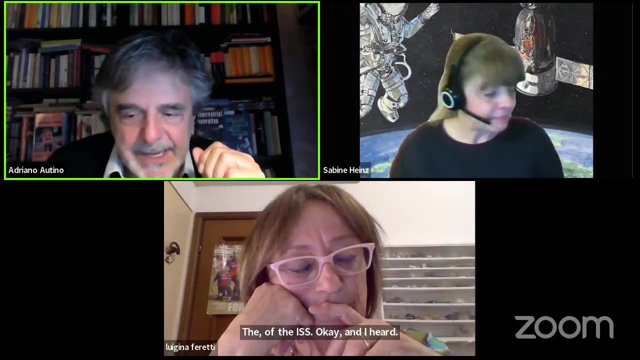 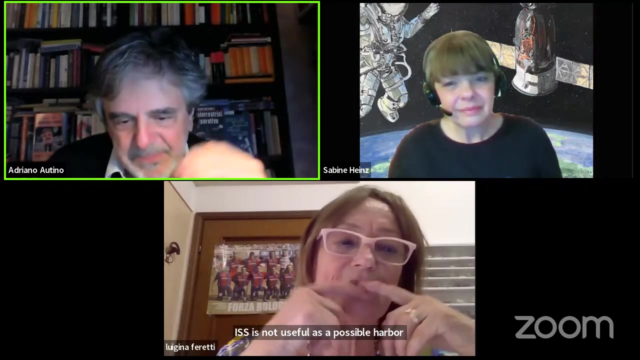 Yeah, a small question. I hope the answer will be quick as well. You have shown in one of your slides the orbit of the ISS, okay, And I heard some time ago that ISS is not useful as a possible harbor to start missions, space missions, from there. 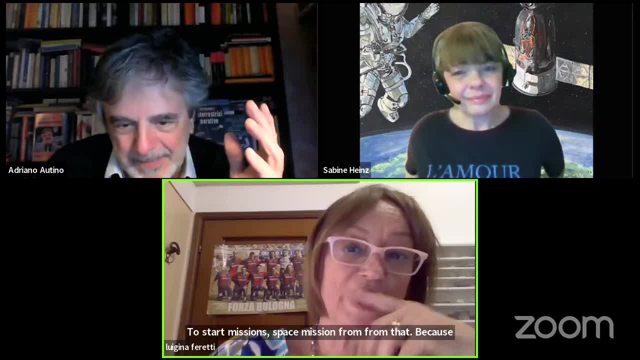 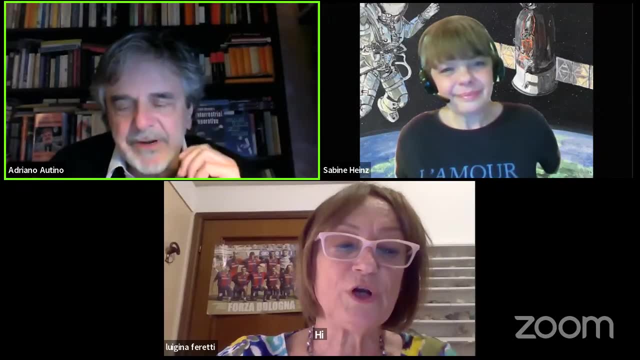 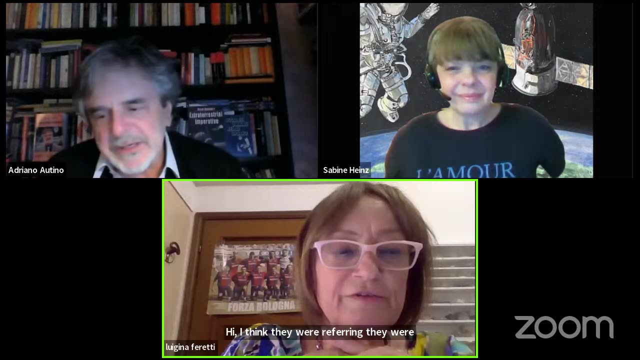 Because of the orbit. So why? Why it's too low? Why it is too low? I- I think they were referring It is too close to the Earth, So it is not of help. It's not of help starting from the ISS. because it's so close to the Earth. So that is the reason You better, Instead of sending a spacecraft to the ISS and then having it to start a mission from there, you just send from there. If you want, I can go back to. 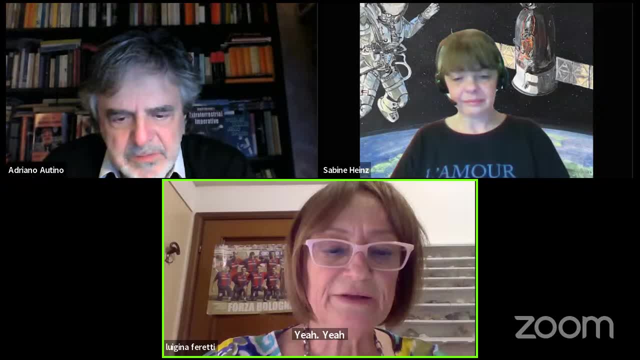 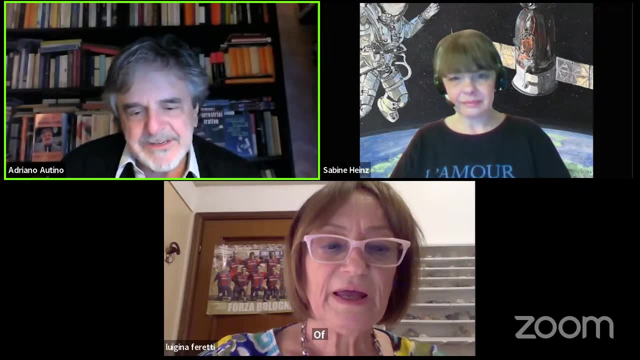 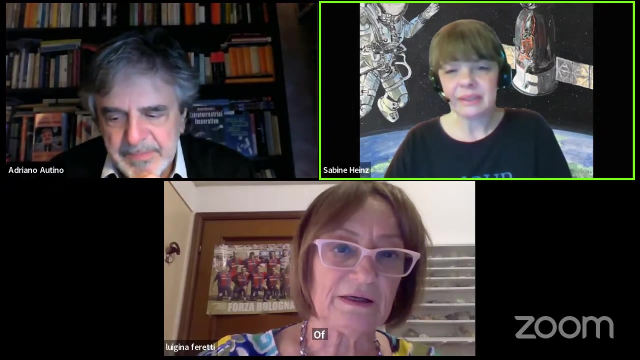 I can go back to the. I think they also referred to the particular inclination of the orbit, That is. I don't remember exactly, but I I think it was slice 11, something like this. So let's see if I am able to. 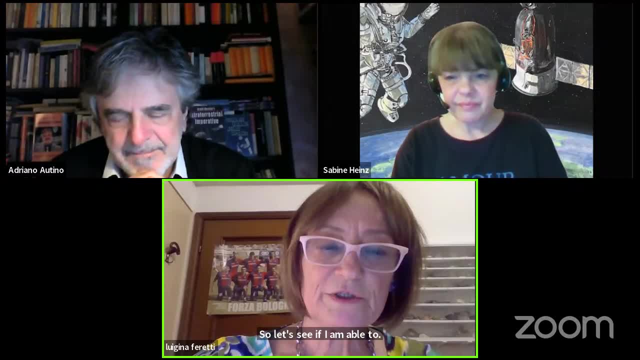 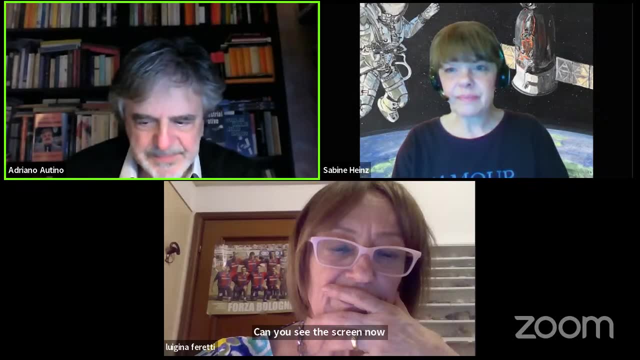 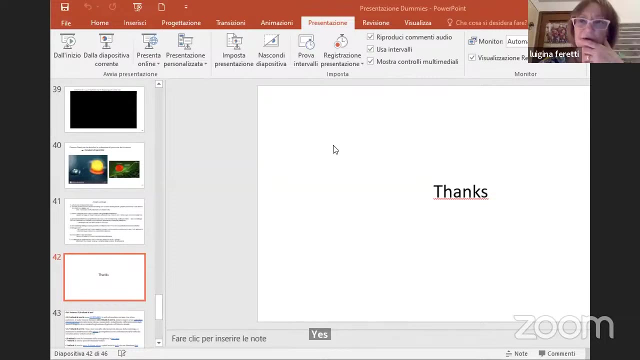 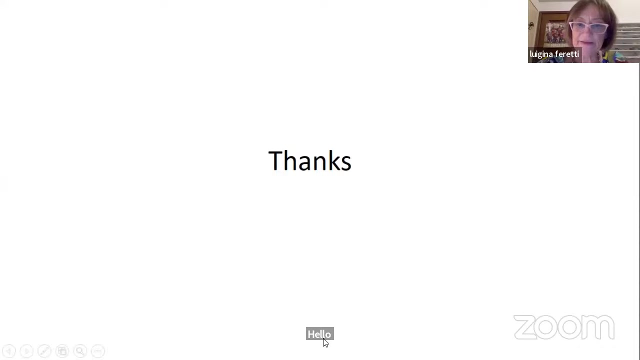 No, wait a moment, Then. Can you see the screen now, No, No, Yes, Now, yes, Yes, Yes, You see the screen, but I don't. Ah, yes, I do, So Let's go back. 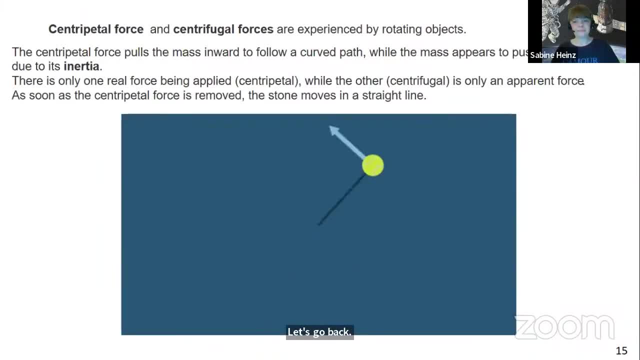 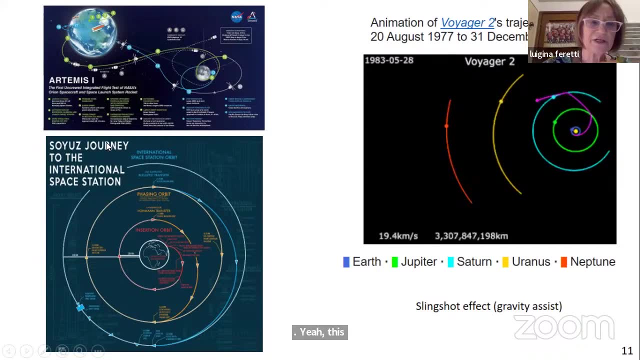 I think it was 11.. Yes, No, No. Yes, This is the SIOS journey to the International Space Station. So you see it's very complicated sending things, But there was the Earth, big Earth and the orbit. 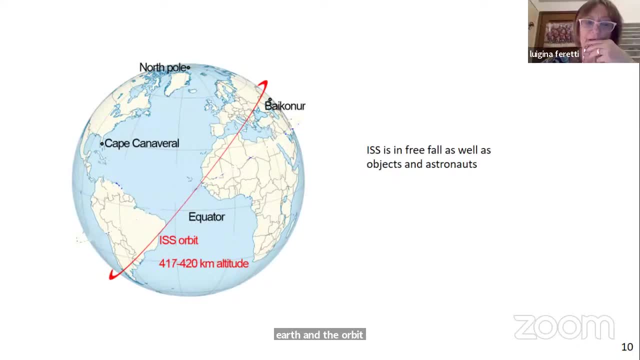 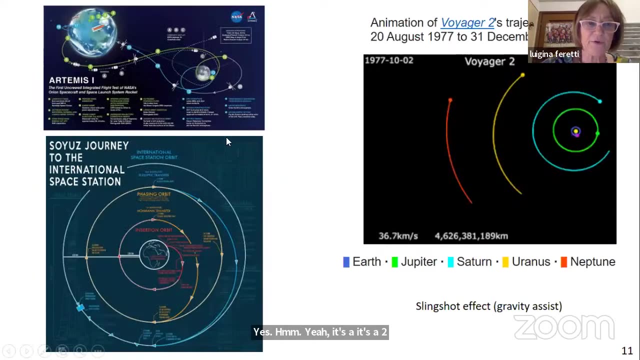 This one, This one, Yes, Yes, It was 10.. Okay, Yes, It's too close, I think. You see, when you go to the Moon, you have to run around the Earth and then go to the Moon. 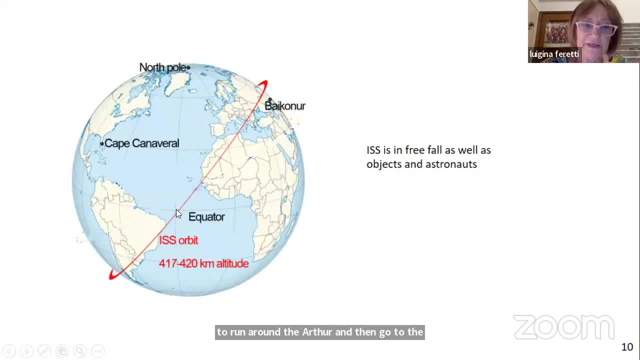 Starting from this small. This orbit is too low, It's not useful for this. This is my, So it's not a real advantage. It's not a real advantage because you are traveling at 27 km per hour, but that's not enough. 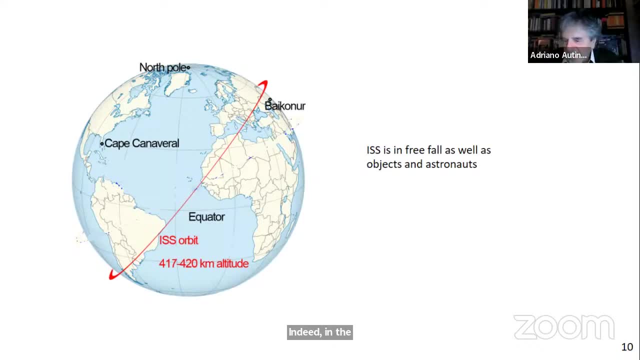 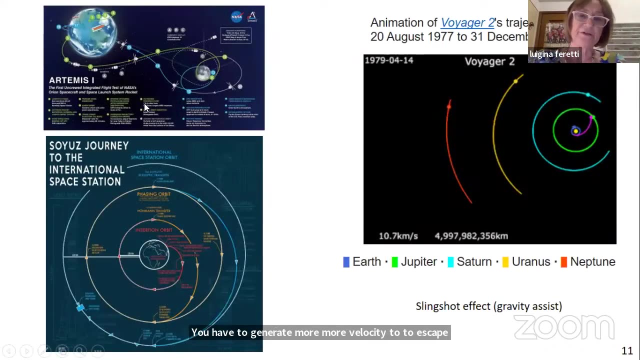 Indeed, Indeed. You have to generate more velocity to escape. Yes, Okay, So you better go directly at your target. Okay, Okay, Thank you, You know. Okay, May I Just as? Yeah, Yeah, Okay. 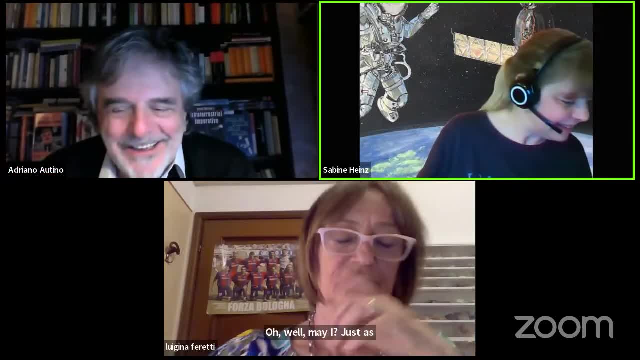 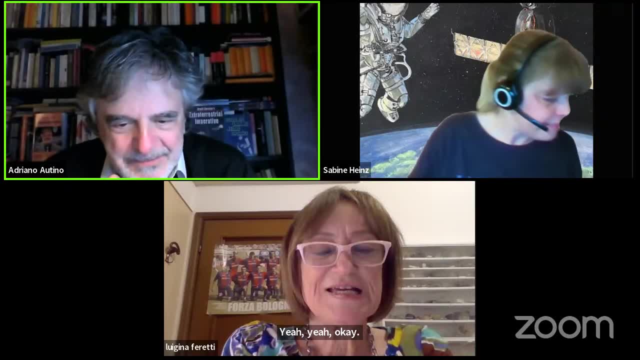 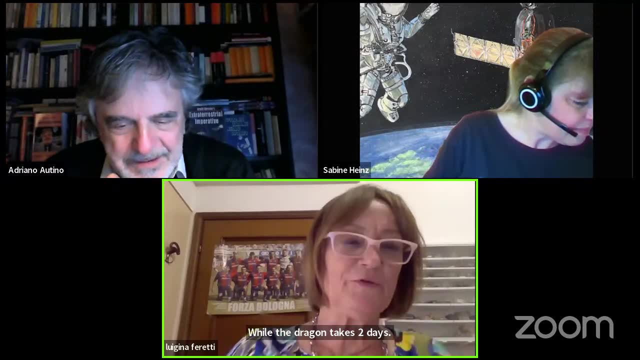 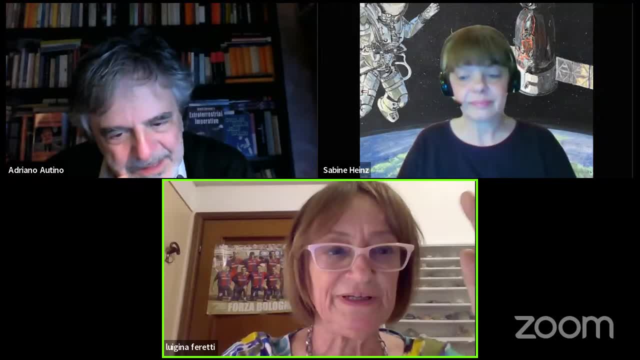 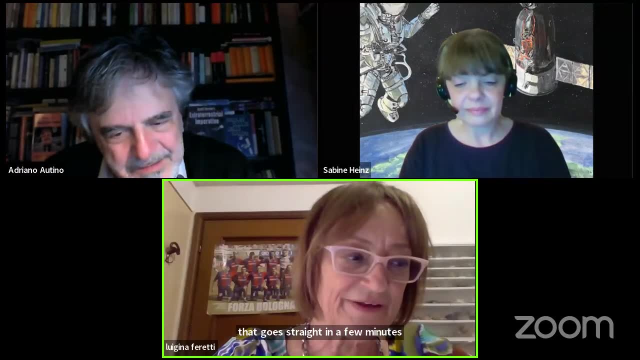 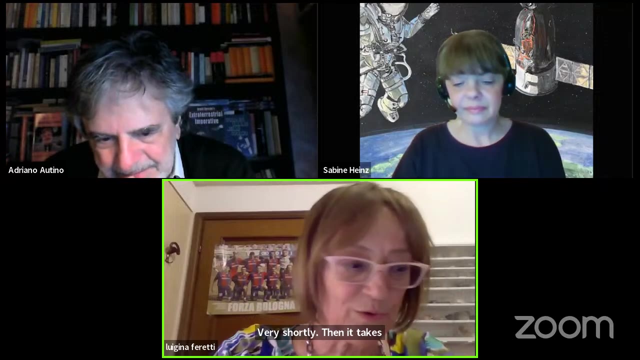 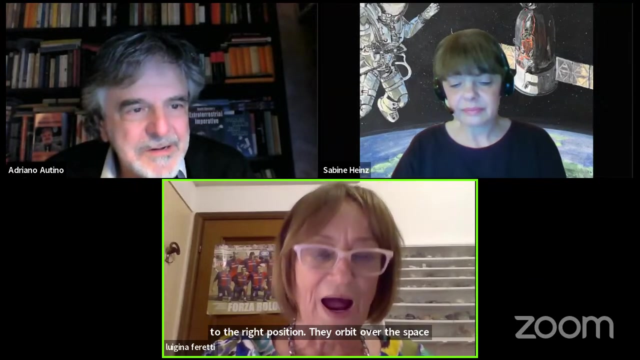 So at the speed, at the escape velocity, the spacecraft could go straight in a few minutes. So the spacecraft can reach the height very shortly. Then it takes hours because it has to go to the right position. orbit of the space station. i just showed one orbit but you know it changes continuously. 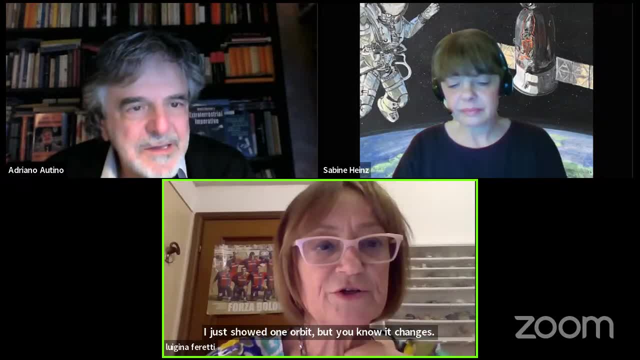 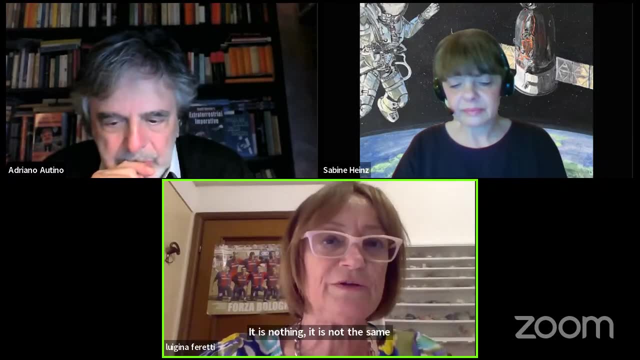 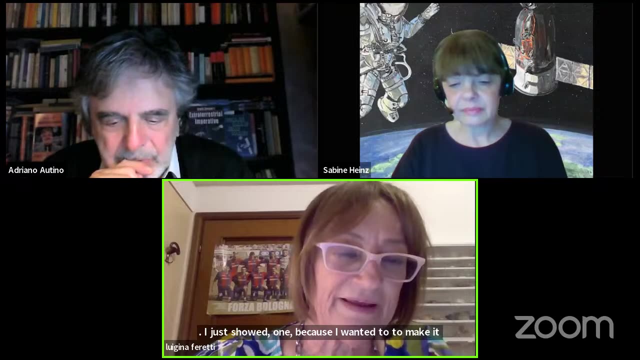 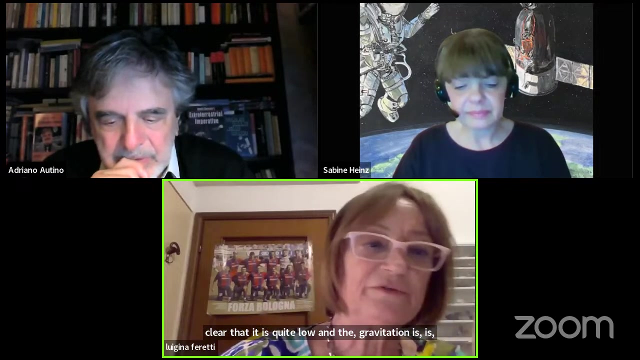 it changes continuously the orbit of the space station. okay, oh, by the way. uh, it is not around. it is not the same. i just showed one because i wanted to to make it clear that it is quite low and the gravitation is. is you don't feel gravitation? not because the gravitational 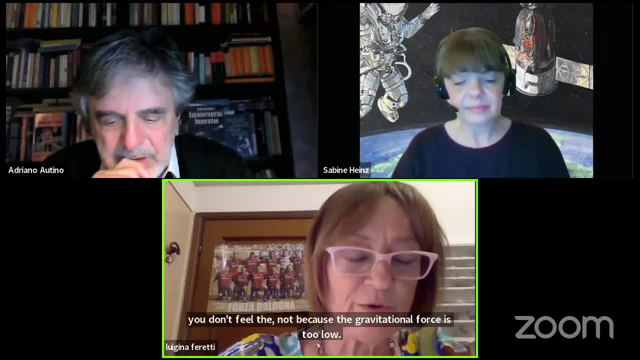 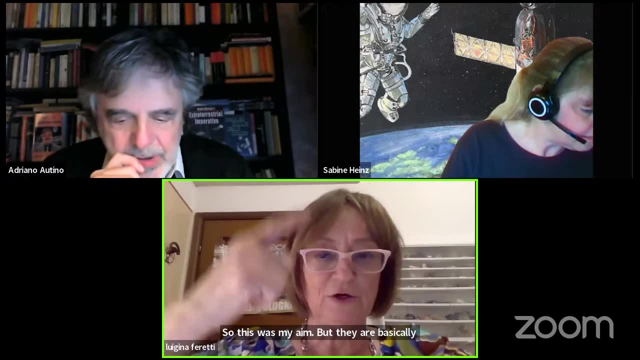 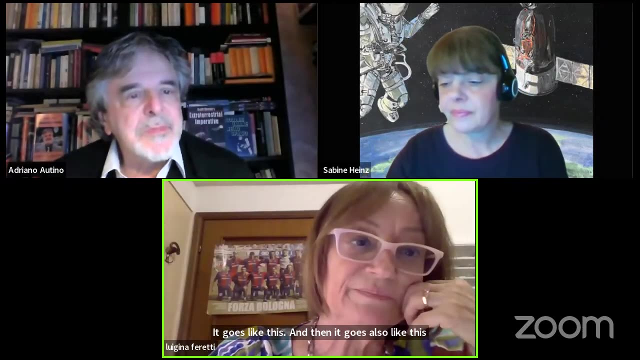 force is too low, but because you are in free fall. yeah, so this was my, my aim, but the orbits are very, very different. it goes like this and then it goes also like this, otherwise you'll see space station every evening. however, we have a. we have an answer by alberto cavallo in the chat. 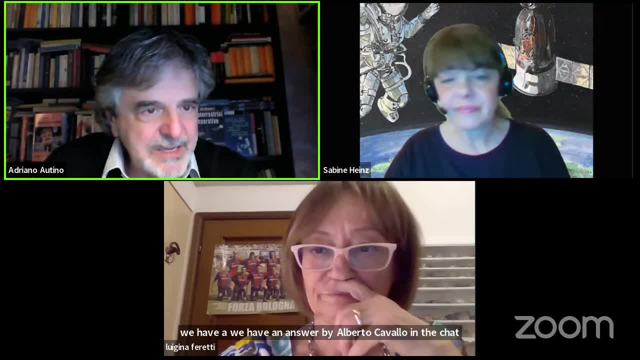 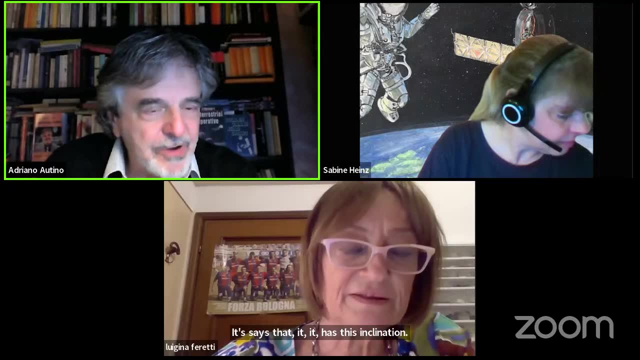 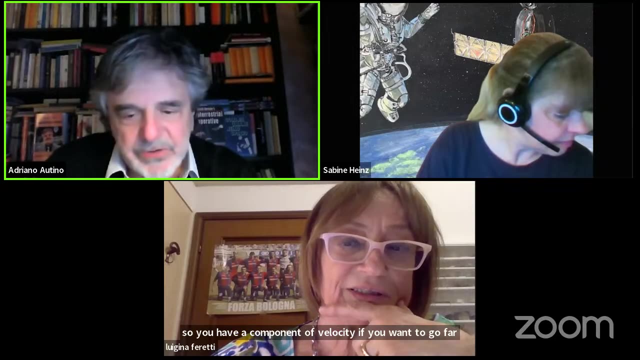 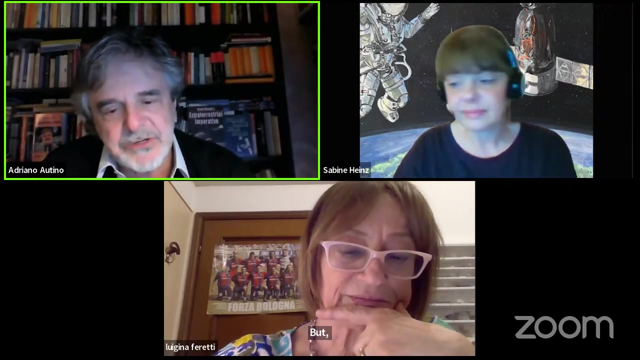 it says that: uh, it, it, it has this inclination. uh, it is not circling around the equator, so you have one component of velocity if you want to go farther. this inclination was chosen to make it reachable from biconor, but but uh yeah, also the, the particular inclination is also not useful. 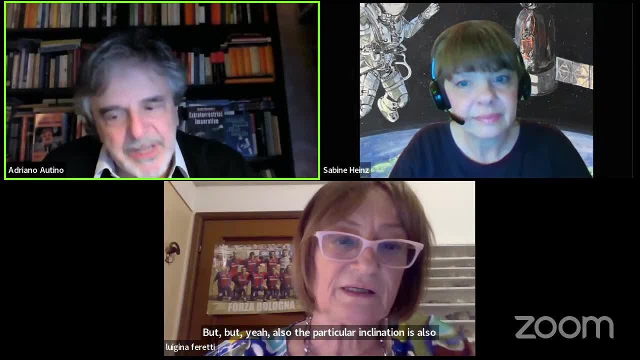 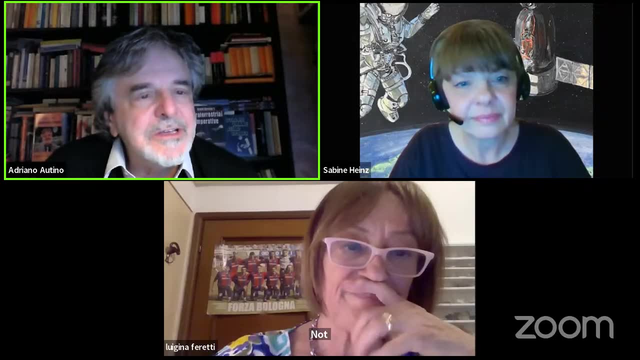 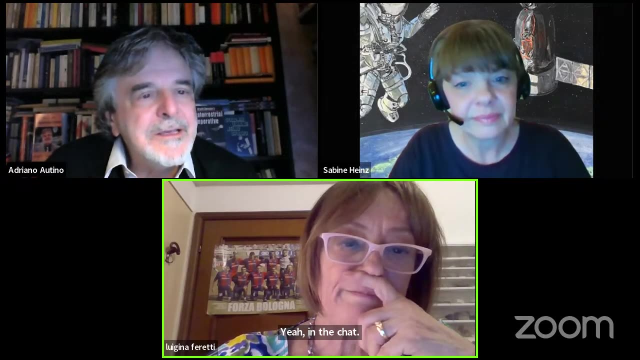 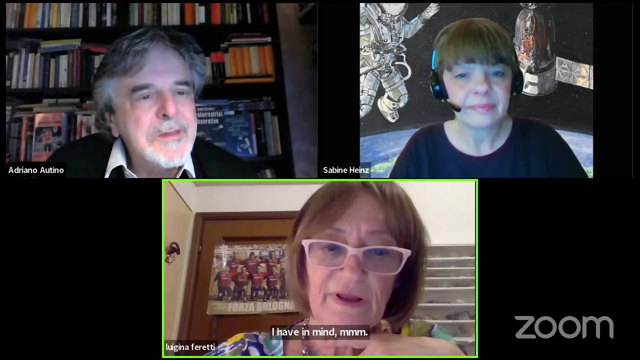 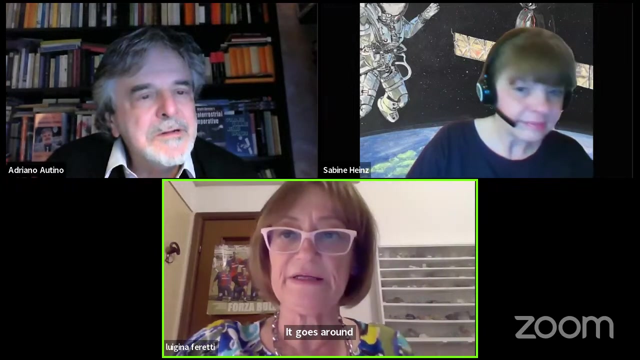 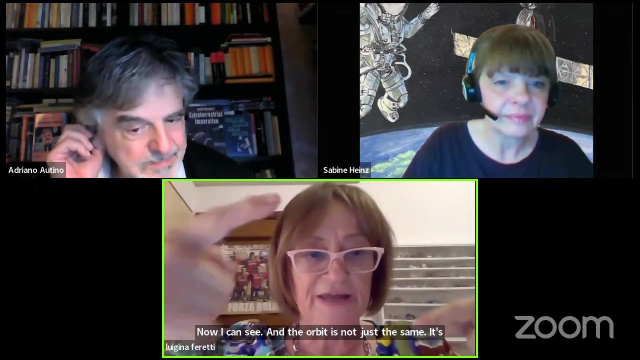 to for uh, for starting from there and going to go farther. not only i have in mind that the orbit of it goes around. now i can see, and the orbit is not, uh, just the same. it's not always the same, it changes, it changes continuously and it. 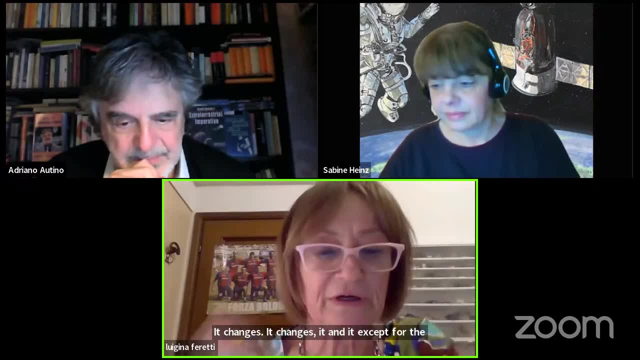 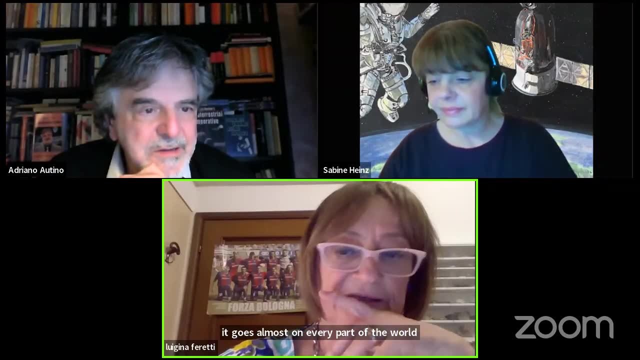 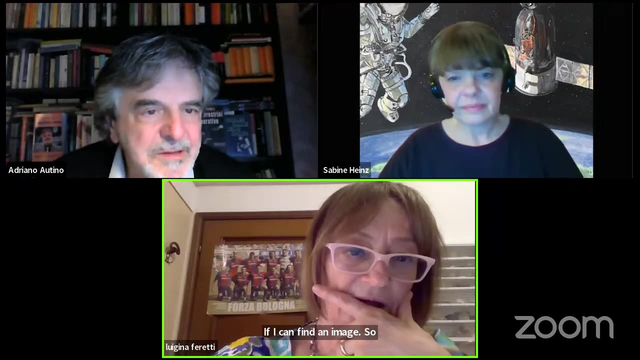 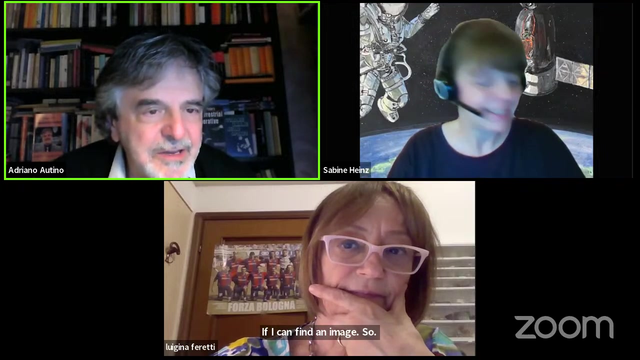 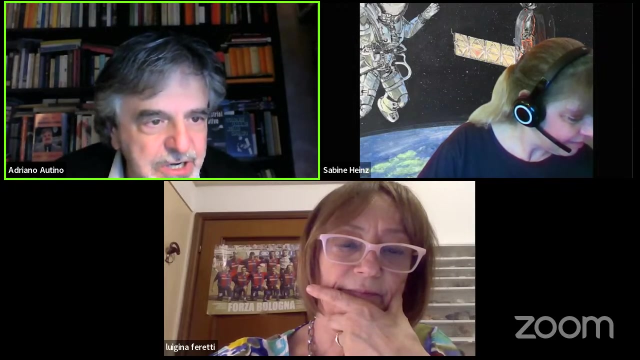 except for the poles. it goes almost on every part of the world. if i can find an image, so i'm doing okay, and thurston frank is saying that about the time to reach the iss. roscosmos is also using very tight launch windows which enable a short transit time. 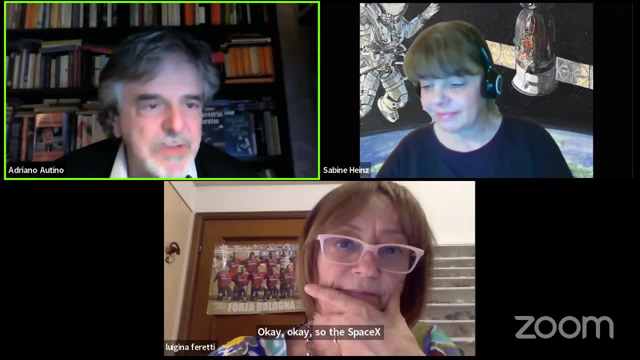 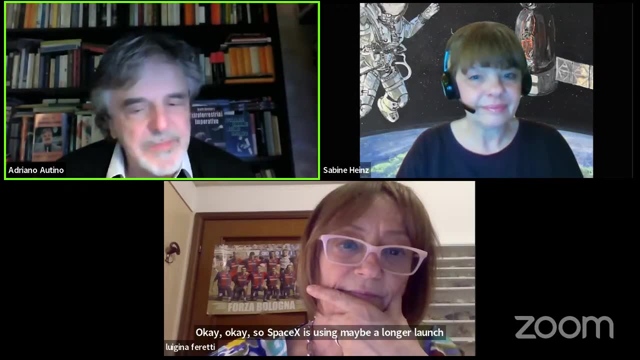 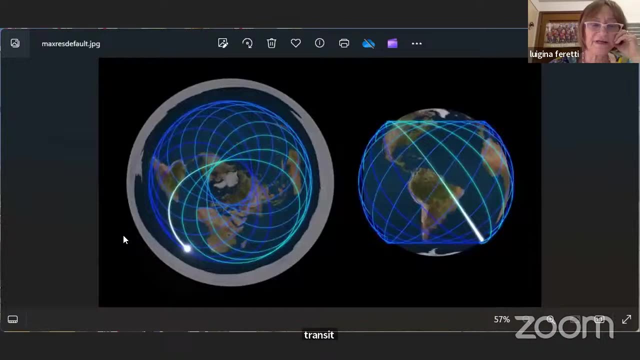 okay, okay. so, uh, spacex is using maybe a longer uh launch windows. that uh give some more constraints about, uh, the, the, the, uh, the transit time. oh, can you see the screen? yes, these are. the orbit of the iss is not just one that i showed, but it changes continuously, you see, but it's not never equatorial, however. so it's never equatorial. 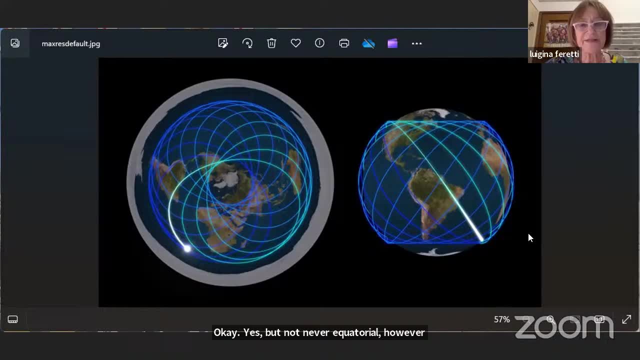 and it doesn't go on the pole. yes, but it goes like this: alberto is saying that an equatorial orbit is uh important when you have to to escape from from orbit. okay, okay, that was saying it is not circling around the equator. alberto saying it's not circling around the equator like she. 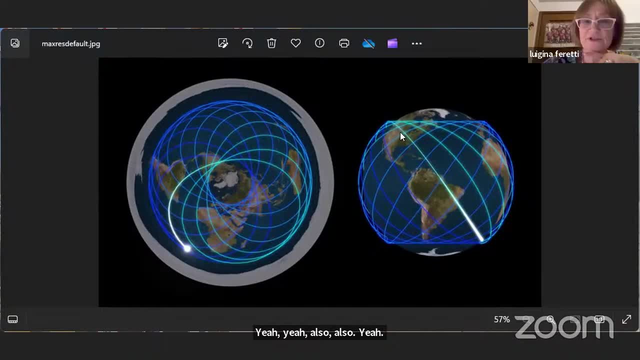 is telling us: adriano, no, i'm not, i'm not saying, i'm showing the image. yes, yes, yes, yes, yes, but he is saying the same, like you. what i try to say is that there are different parts. yeah, yeah, yeah, yeah, yeah, yeah, the one, uh, this is just one orbit that i showed in the presentation. i will change it because it's. 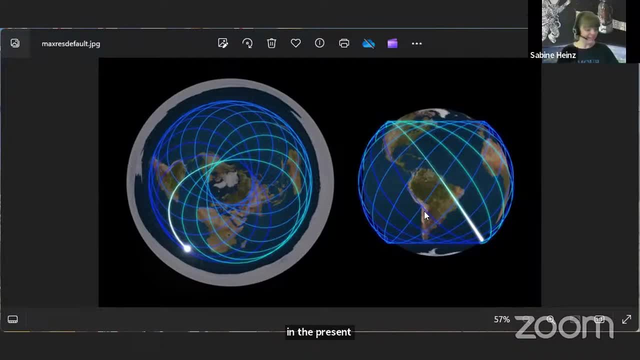 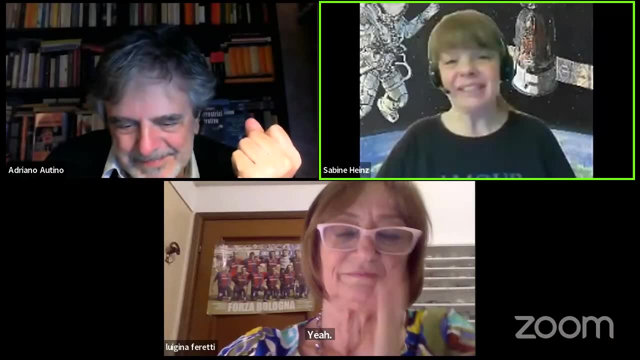 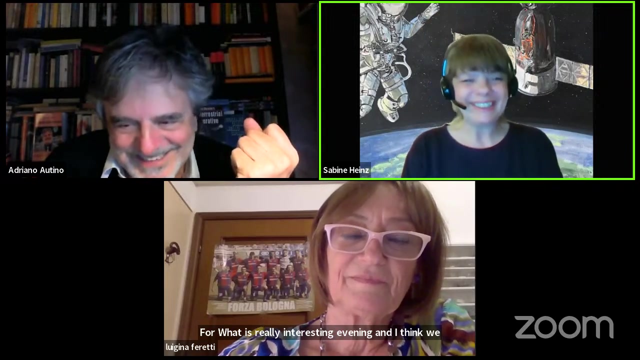 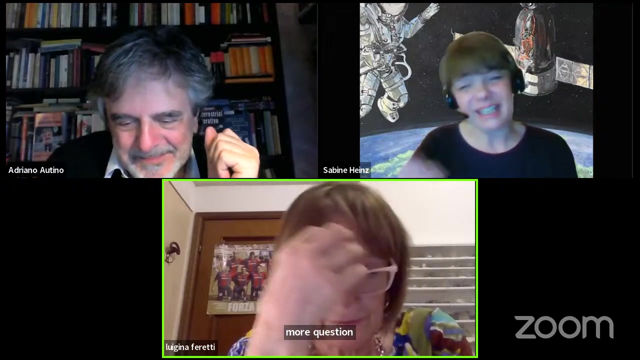 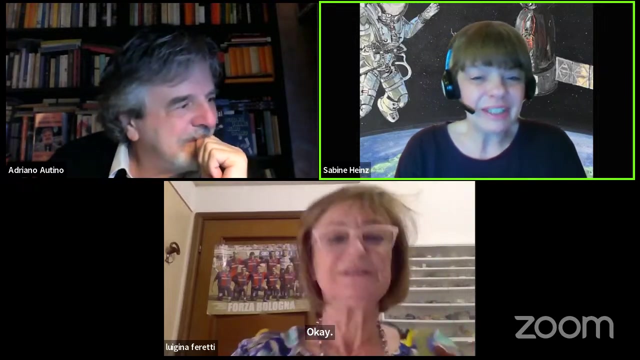 misleading. yes, yes, it's the same like you, okay. um. i thank you so much, um, for for this really interesting evening and i think we would like to invite you again. uh, i i think we have more questions uh we can talk about and uh, okay, as i told you on forehand uh, so maybe we can uh use this. um. thank you very much, uh for this. 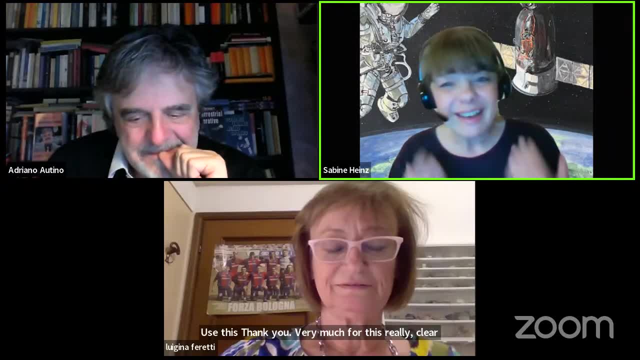 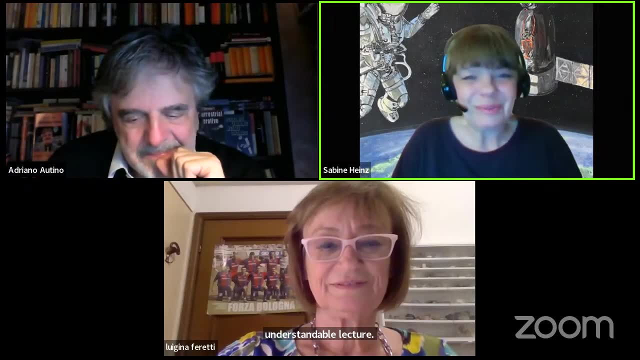 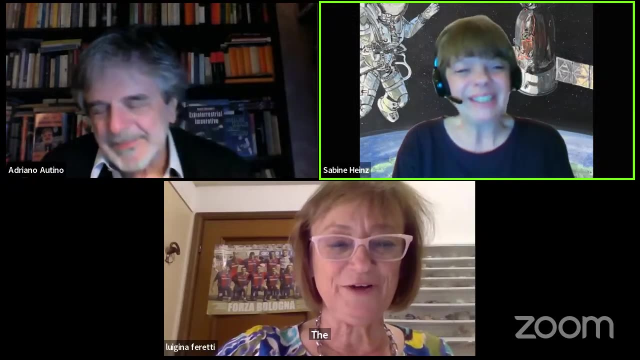 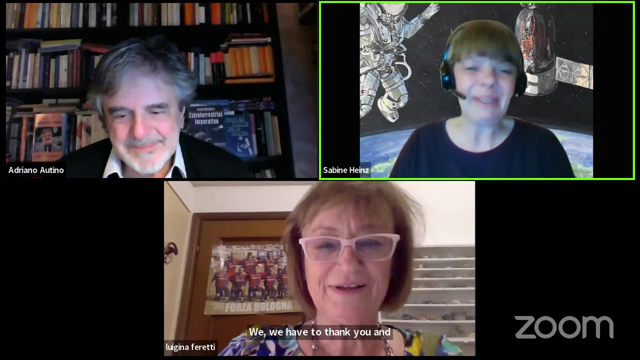 really uh clear and uh understandable lecture and uh, yeah, i i took a lot from this. um, okay, no, i'm, i'm glad, i i thank, i thank you for the we we have to thank you and and i'm really happy for your in interest in, uh, yes, uh, we are really happy and, um, thank you again and i would like to mention that